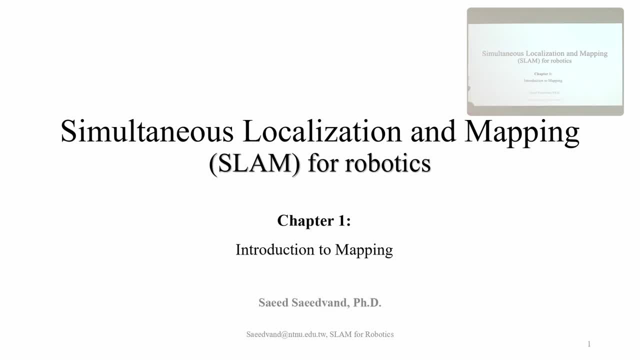 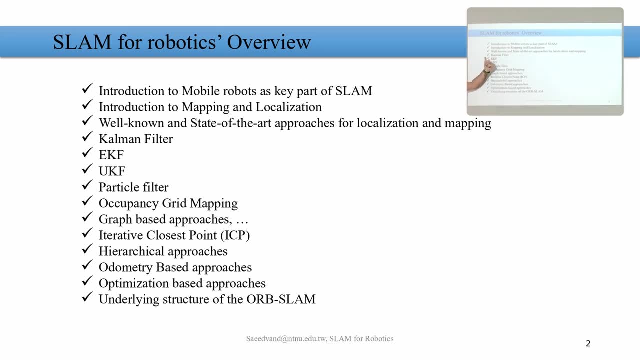 are the real challenges in the SLAM algorithm. So we discussed that. the topics that we have are introduction, then we will talk about the localization and mapping, then we dive into the different algorithms. We start from base filter. we talk about Kalman filter, extended Kalman filter, unscented Kalman. 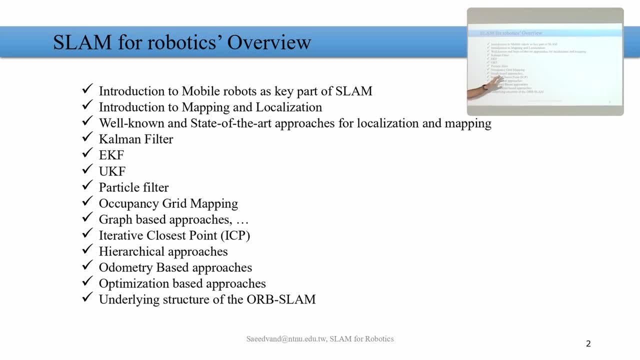 filter, particle filter, and continue with occupancy grid mapping, the graph-based approaches, and then we will talk about the localization and mapping of SLAM algorithms, ICP iterative closed map, that we use it for 3D construction of the map in the 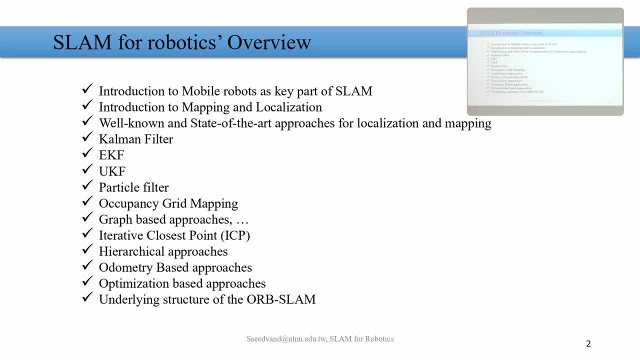 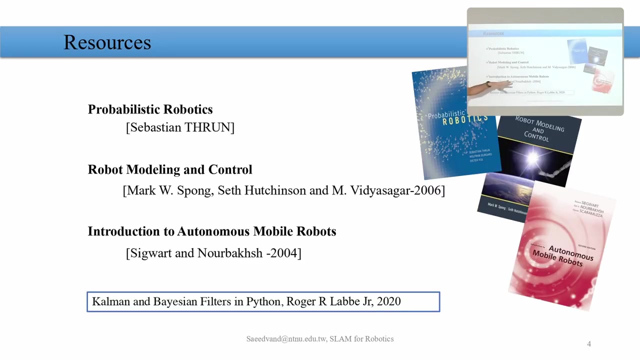 environment, hierarchical approaches, odometry-based approaches and we will move toward the optimization and more algorithms like Orb-SLAM. that is one of the famous and the most strong algorithm that we have in SLAM area: simultaneous localization and mapping. So we introduce three books, but also- I forgot to mention there is one useful- 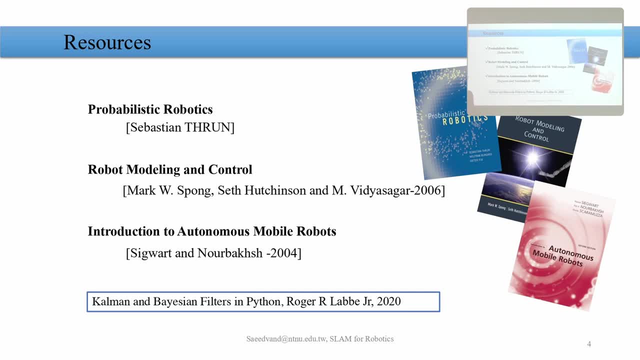 book that later I will introduce and talk about it in detail when you're gonna implement the codes, the examples, whatever I'm talking in the slides, the equations, the algorithms that I'm explaining mostly are implemented already here. It is pretty decent step-by-step book that that, for example. 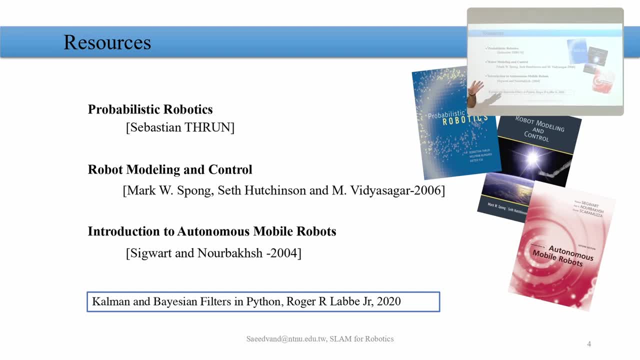 We will study the Kalman filter. then, after you understand what's happening there, You will move to the book and same example, very similar example, already implemented there. You try to re-implement it. first, plus, There is Python code plus. then later I will give you some assignment that you need to work on it. 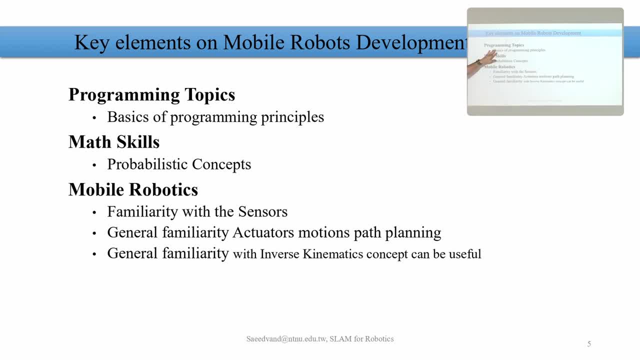 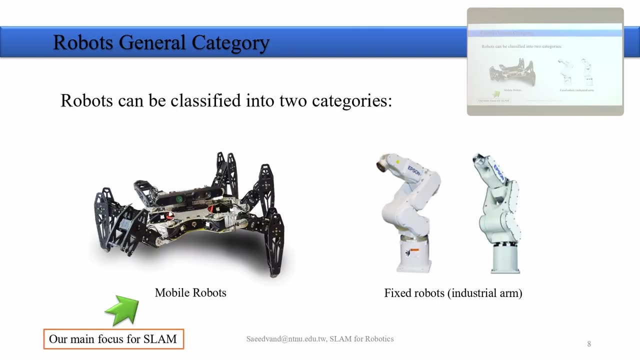 So, as I mentioned last week, you need to know programming topics, you need to know the, You need to have some math skills and know the basics of the mobile robotics. In this chapter we are talking about the basic introduction. We talked about the: what's the robot, What's the mapping? 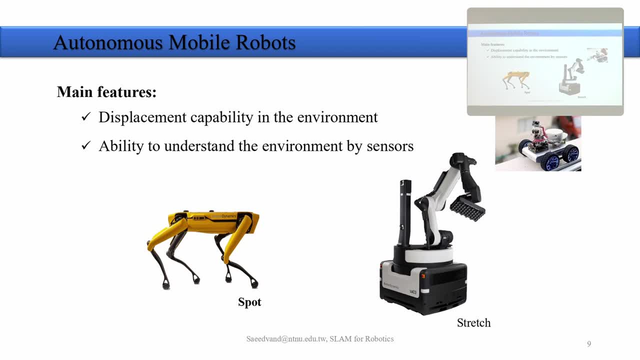 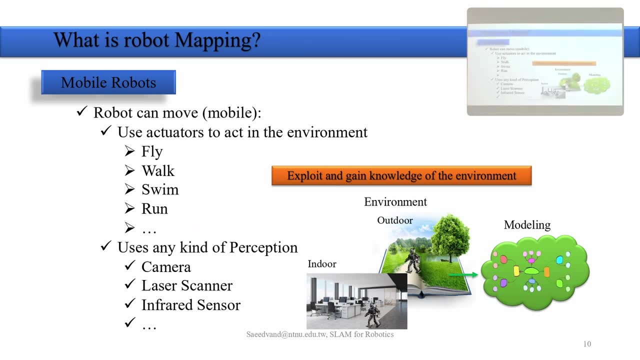 What's the mobile robot? What's the fixed robot? We talked about different famous robots and general introduction of spot stretch and simple robots. that we said doesn't matter which kind of robot we have. if it's Just mobile, then we need the SLAM algorithm to solve the problem. 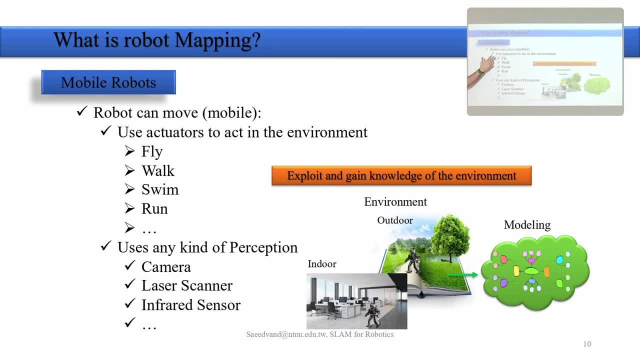 Different kinds of robots that we have and we can apply SLAM algorithm like fly, fly Walking robot, swimming robot, running robot, whatever the robot that is Mobile. and in the environment. we talked that we can have two types of environments: indoor, outdoor. Because of that challenge, because of the scenario, the challenge can be different. 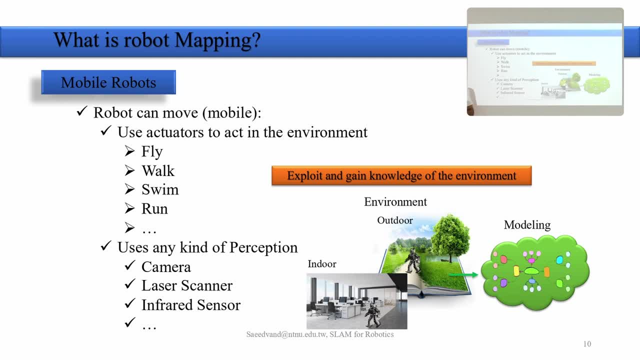 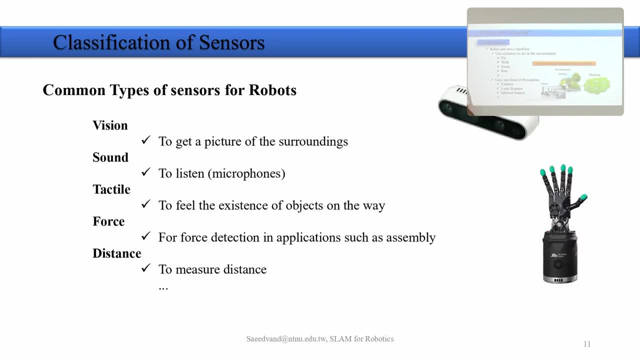 Of course we would like to have general proposed robot that can work in either environments, but usually for now They are split it into two, in different challenge and competitions. so Different kinds of sensors. we will dive in in some types of sensors. We will also try to formulate it in mass form in order to be able to use it in our algorithms. 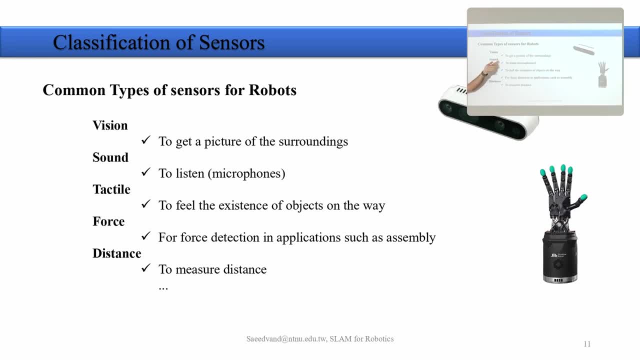 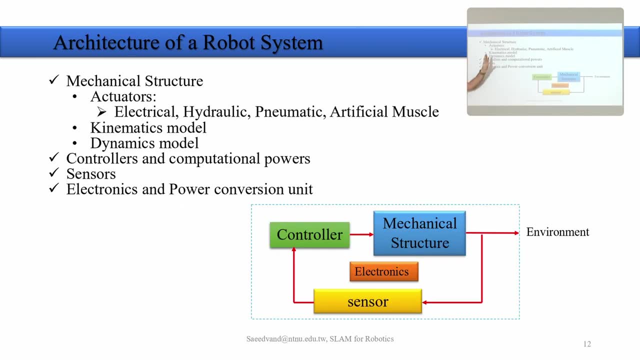 but we have vision and We have some sensors: tactile sensors, force sensors and distance sensor. that I lastly Generally described it. We had a look at general structure of a robot. whatever the robot is. we said that we follow the sensor, electronic, mechanic and controller that you basically already knew in advance. we saw the 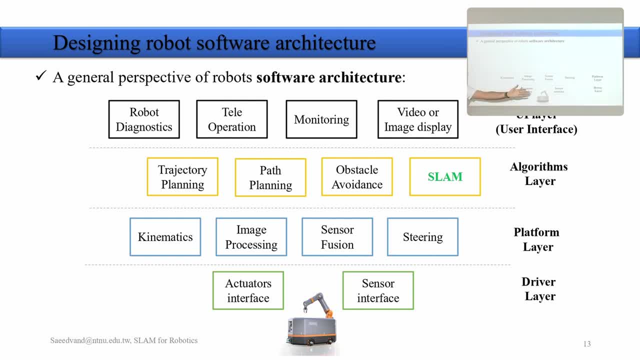 hierarchical level of the. our robotic system is working in driver layer, platform layer, algorithm layer, then UI layer, that these are all connected together to to Launch a robot. that robot performs in the environment. but why we discussed this? because we wanted to see Where the SLAM is. the SLAM is located in this part here and we are going to dive in. 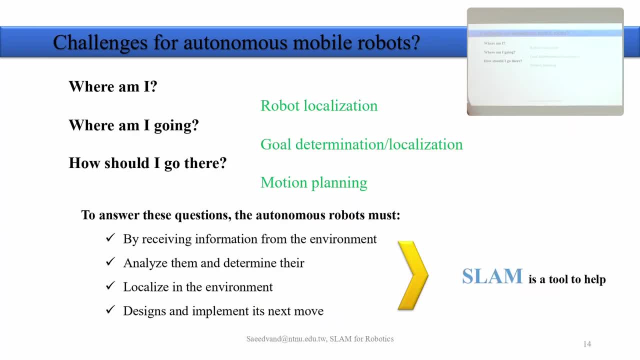 one of the algorithm layers in robotic system. So then we answered the questions: where am I? robot asks Himself or itself: Where am I? That? the answer is robot localization. So imagine here robot is somewhere. if asks where am I? we say we. The answer is the algorithms in area of robot localization. 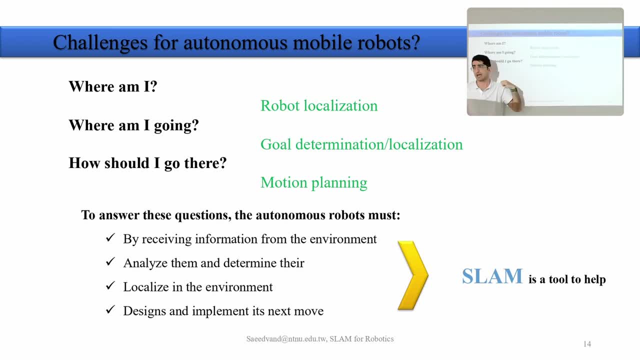 Then where am I going? the goal determination and again localization and how should I go there? The answer, the answer in this question was motion planning. so all these and the answers moves to our to Show the importance of the SLAM that we discussed and we said for understanding SLAM. 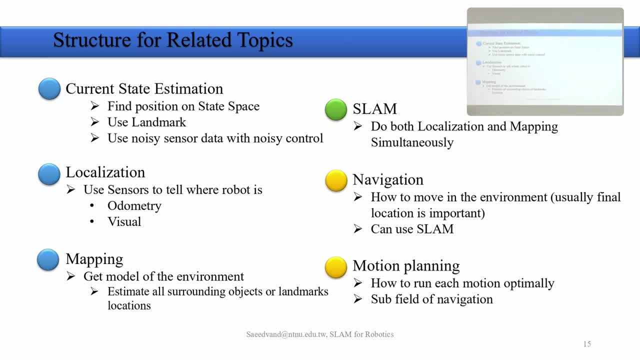 There are multiple topics that better to know and we need to know. actually, One is current state estimation, that we have the state space we discussed and, based on the state space, Robot tries to guess where it is. so Current state estimation. we talked about localization, the same, and we said there are two types, that today we are going to clarify them. 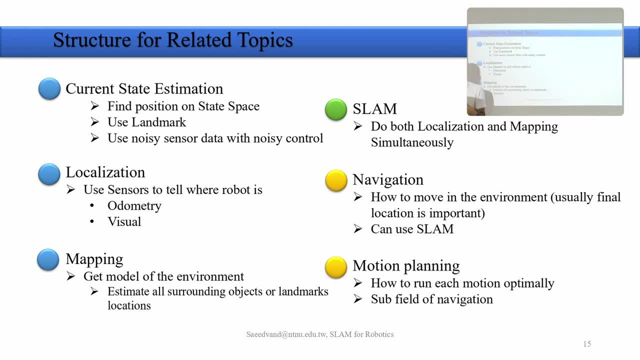 Then we have the mapping. Mapping means that when robot is moving in the environment, We want to construct a map, and today we will see what kind of maps We can have and and what are the applications are we can, how we can use them, based on those relevant topics. 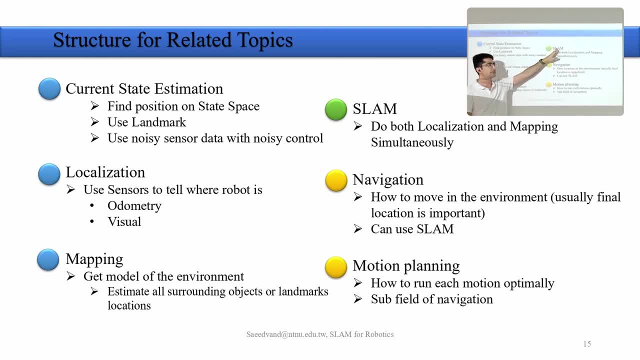 We said we have the SLAM, that SLAM is trying to do both together Simultaneously: localization and mapping. Meanwhile, we have some topics that also we discussed, like Navigation and motion planning. there are relevant, similar topics that we need to know and we need to be able to distinguish when studying and reading. 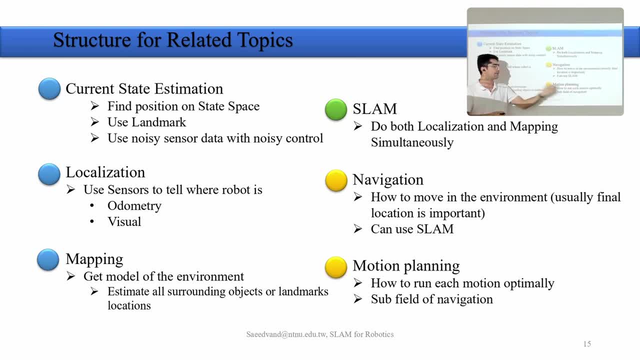 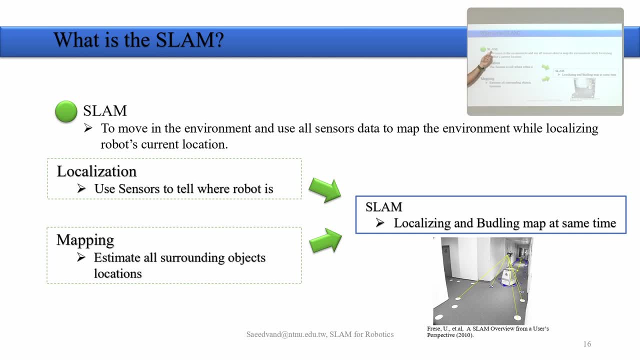 different papers and understanding them. Navigation and motion planning: we discussed that, how robot is trying to do, But generally, as we said, SLAM is most importantly focusing on Localization and mapping and finally we have the SLAM. you can see the robot there that moving in the corridor and localizing different. 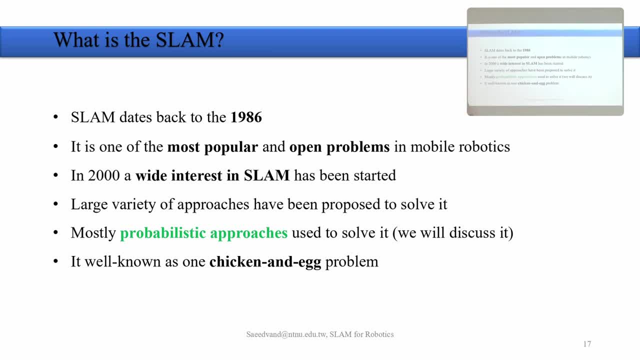 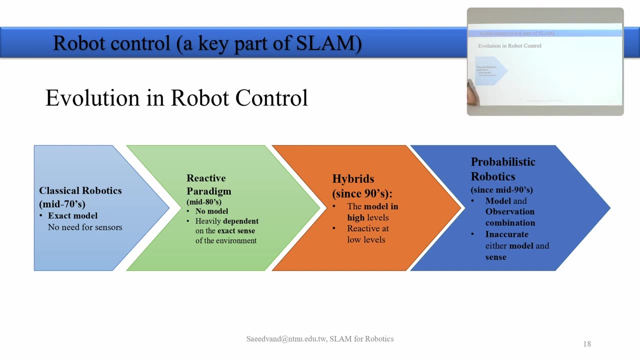 Landmarks or different objects where they are based. on that Robot can say okay, Where am I, answers Where am I, And and construct the map of the environment. So we discussed quick What is the background and we saw the The evolution of the robot control. why? because it was very important for us, because we are going to use the probabilistic. 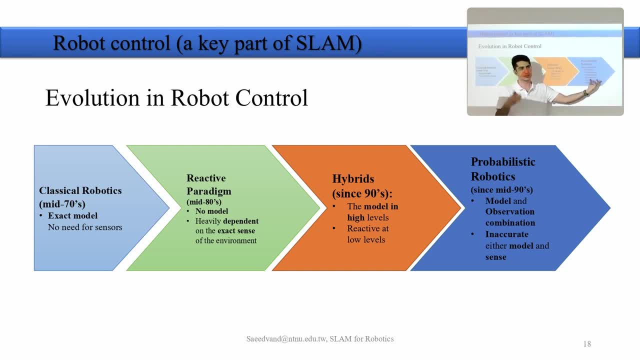 Robotics. at the last stage- that is the most advanced stage that currently we are, and we will see what it is- We try to actually In whole course, we try to formalize it. We try to first bring it into mass form, then try to Engage some algorithm to solve it. 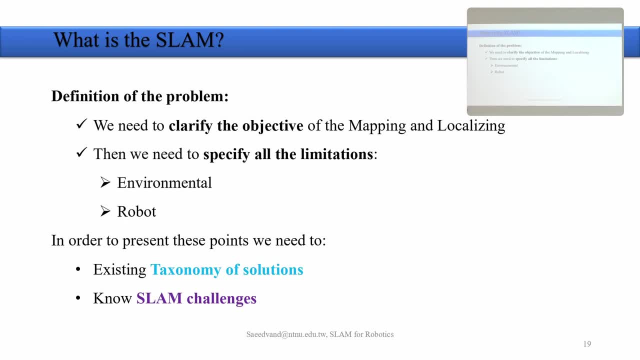 Then Did the definition of? in the definition of problem We say we need to clarify the objective of the mapping and localization. Why? because the objective can be important. if you have a robot that is moving into the environment on the surface, on the Floor, and we need to construct to the map of the environment. that's different from the flying robot That is flying your outside. 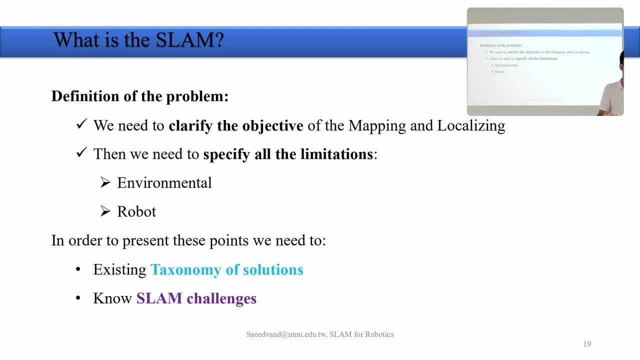 so and Landmark can be different too. So a humanoid robot, a mobile robot inside, Like when it's on the floor and walking and moving, the kind of map that we can have and the kind of localization that we have is different from the robot that is flying, because 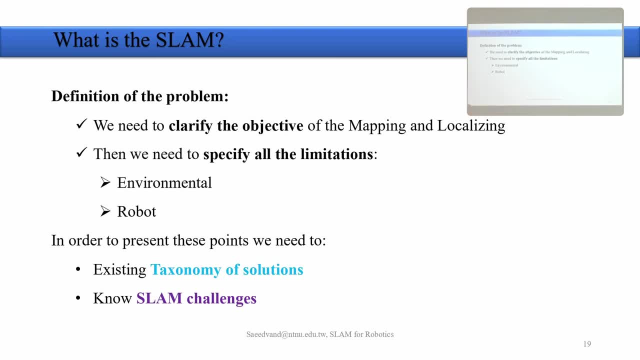 You don't like the object from this features perspective that you see can be totally different from uptown view. So the the goals should be determined based on the what we want to do, then Apply the localization or if you are going to. basically, in this course we are focusing on robots. 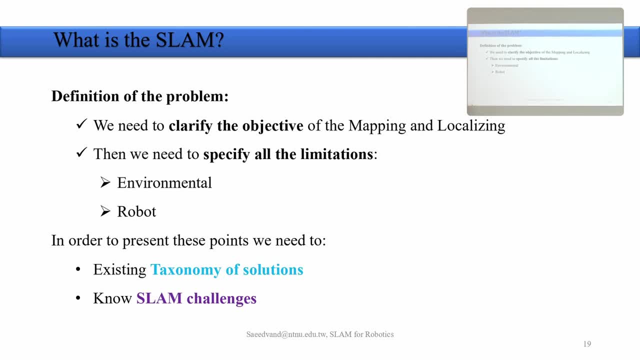 Not the unmanned vehicles, and there can be some small differences, some different challenge too, because in in unmanned vehicles You have pedestrian That walking and those are very crucial to take care of. for nine robotic systems We have slow robots Basically. I mean they are not go as fast as the car and 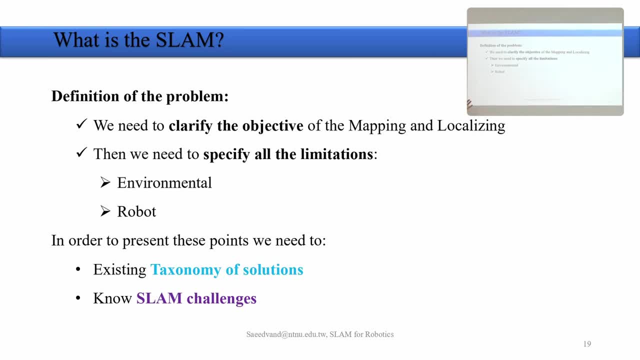 some kind of challenge are a little bit different. general thing is same, but We need to determine the goal and specify all our limitations, same as solving any problem We need. we have some in our environmental limitations and we have some robot Limitations that, based on those, we need to take it in consideration. What does it mean? 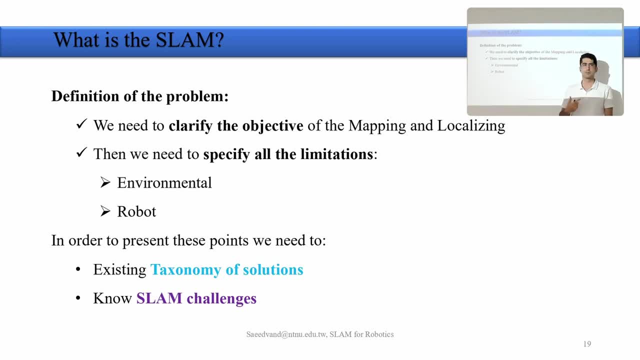 It means that, like, what is the robot limitation? So imagine you have access to different kinds of robots and, based on the robot that you have, you have different capabilities, different sensors, different Actuators. based on those, you need to solve the problem of SLAM. so that can. 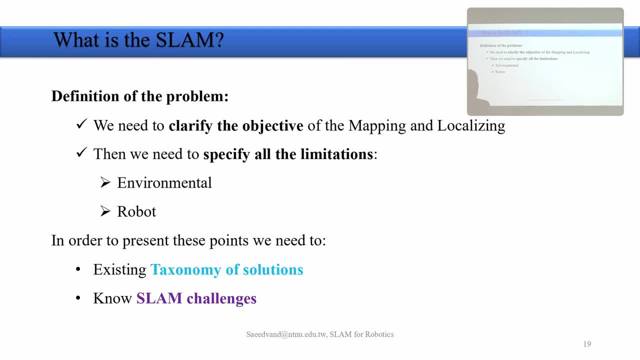 Make a lot of differences in the algorithm that you are gonna solve and work with it, and Today we will see how. In order to present these points, We should have a look, of course, at the taxonomy of the solutions. taxonomy mean like kind of classification of the solutions in 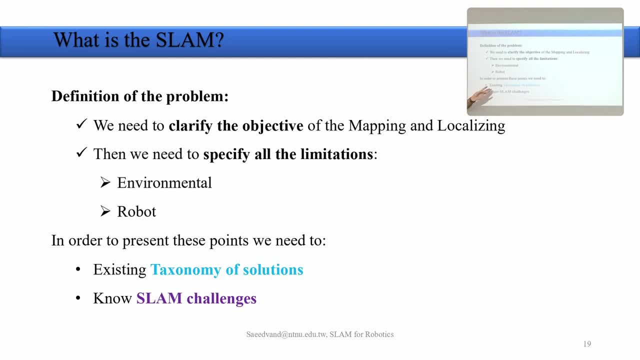 The world, what kind of algorithms we have. if you just search on the internet, the research studies, There are different types and they are totally different with each other. So We should, we should- have a look at those and, of course, the most important part is to know the challenge. 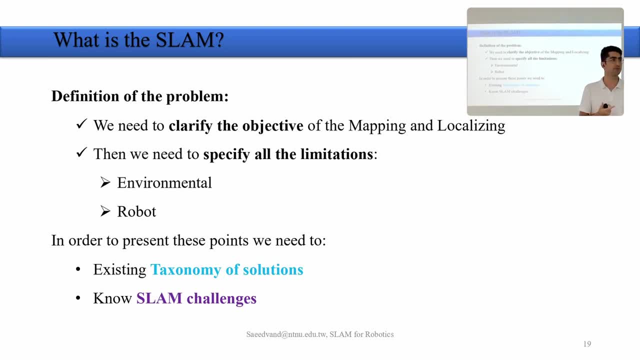 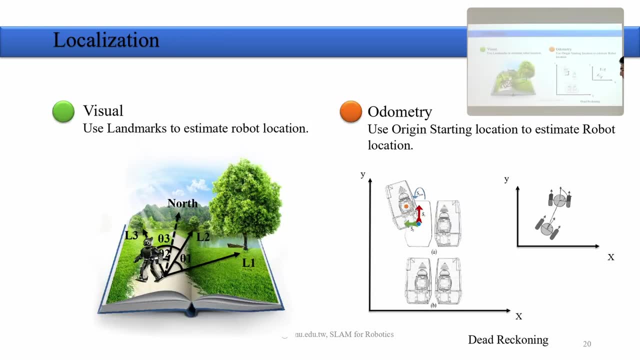 If you don't know the challenge, solving the problem doesn't mean too much. we need to know What we are facing with, what kind of Problems we need to deal with in underlying level of the developing algorithms for SLAM. so now I want to introduce two major classes of the 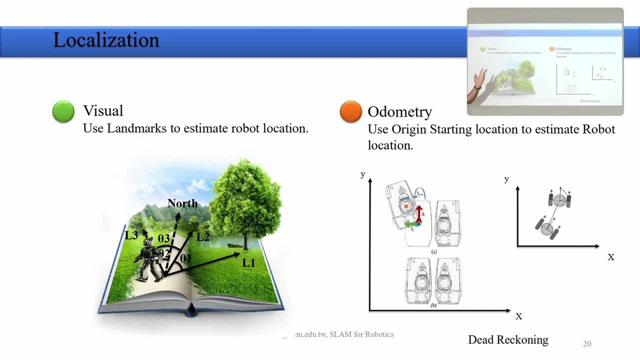 Algorithms for SLAM. one is visual, second is odometry. We have implicitly third one that is combination of these two and we will try also cover all of them. What is the visual? visual says Okay, use the landmarks and different objects, try to localize Or construct the map of the environment by 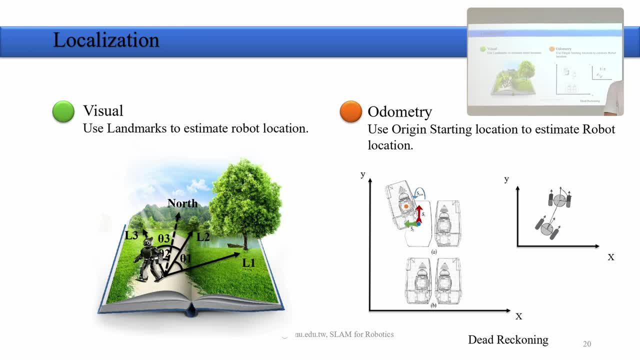 So what kind of sensors we have for that? of course, the obvious one is camera- Second font can be lighter- scanner, and any visual information that can be gathered from environment can lead us to have visual Localization. for example, here we have a robot that moves in the environment and gathers. 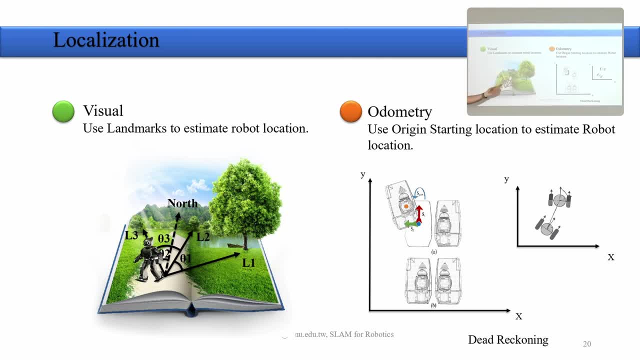 different features from environment and Finds out and localize itself. on the other hand, We have the odometry. What is the odometry? Odometry is using the Amount of movement in the environment by the kinematic model of robot. What does it mean? It means that okay, if I'm humanoid robot. 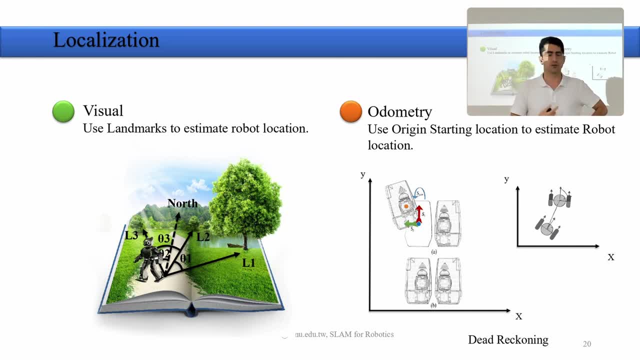 Let's say I don't have any camera. if I close my eye, Then if I move one step to the right, Second step to the right, I almost know where am I right. If I knew where, where I started after some movements, I can guess where am I. 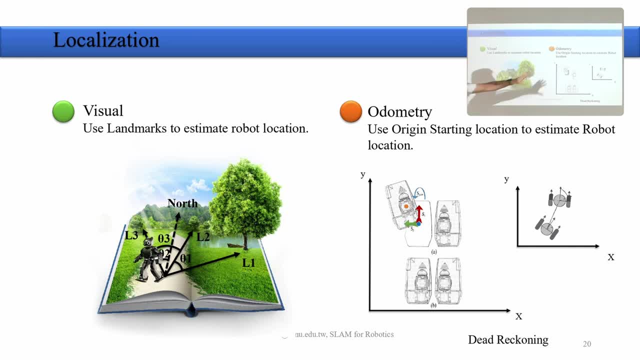 So doesn't matter which kind of robot we have. odometry says: use the locomotion, use the movement estimation in order to say where the robot is. So sometimes This is very difficult to achieve, sometimes not that hard. We will try to formalize everything. What does it mean? why it can be difficult like this is- this is top-down view of a robot- that it has two wheels. 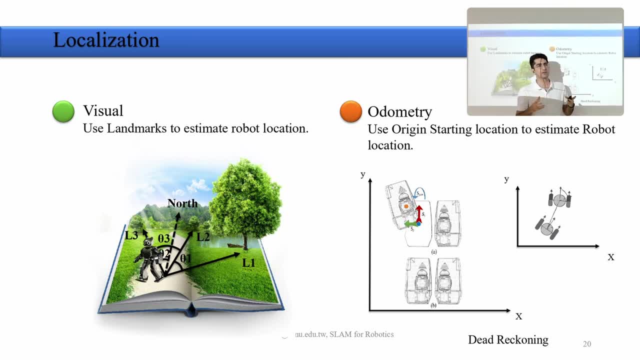 So we can have the counter on each wheel. Then we can count how much robot is moved in the environment, and some with, with some mass. we can calculate where the How much robot moved in the environment, how much rotated how much, how much translated in the environment. 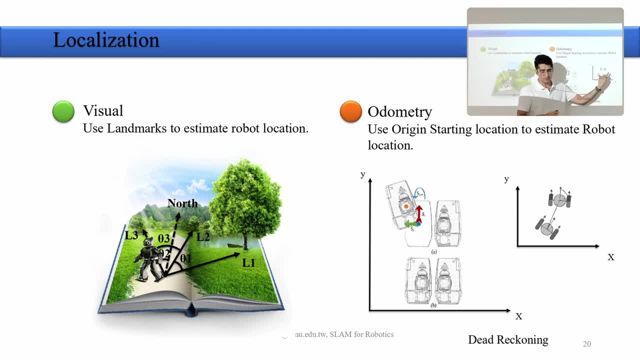 So, But what about the humanoid robot, for example, as one of the complex robots that we have? So calculating the step size is a little bit more challenging, Because if you have only directional walk, it means that robot can walk freely in the environment to any direction and meanwhile also rotate. 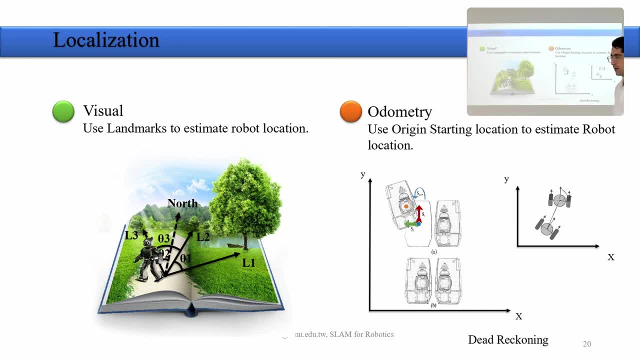 So I'm doing these all motions, But I need to have an accurate calculation of the what is happening in order to say from there to here, What was the distance that I moved, and you have too many joints that is affecting these movements in the environment, So I will also clarify what's happening, how we can also calculate that one. 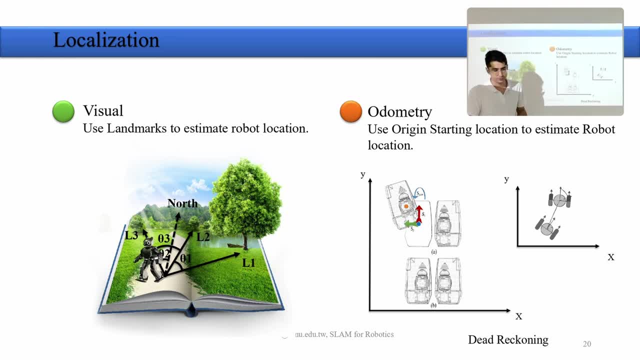 To achieve it in simple or complex robots. but what about the drone? then We cannot count the steps there, how we can use automatically for flying robots- guess it- GPS. so if GPS is accurate, GPS is one parameter we can use, but basically we never use in Islam because 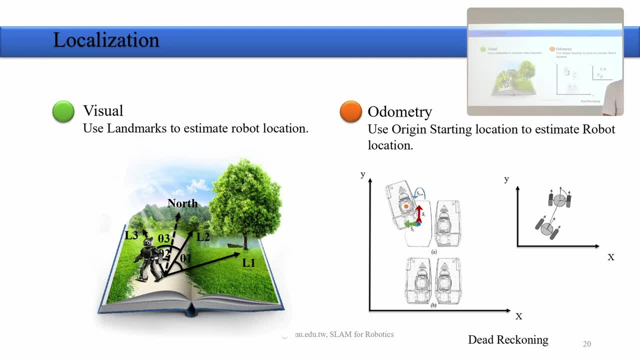 Let's say it's indoor, Can be, can be, but not really because You say, okay, we tilted the robot like this direction but you don't know how far it goes, because it depends on the the Motors speak to. if you are, your robot is like this, it can go 100, it can go 10. 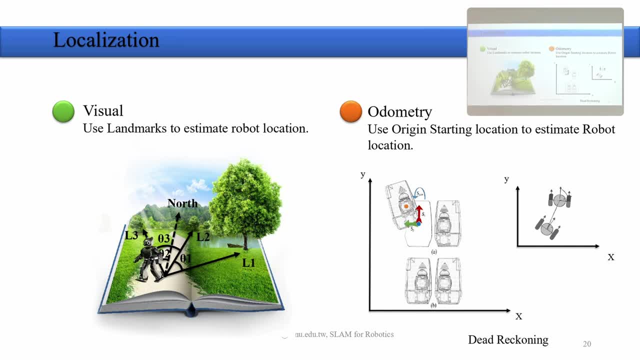 Any guess, Ingram, any guess, Ingram, any guess. We will see velocity based modeling. we can calculate the velocity of the robot based on different sensors and based on the velocity we can estimate the movement of robot, and that's also one of the elements of the most advanced algorithms for Islam. 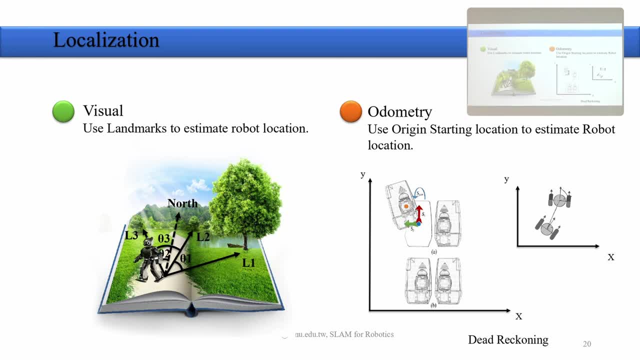 For example, you have IMU. everybody knows what's IMU. Is there anybody you don't know? you know what's the IMU. who knows what's the IMU? rise your hand. Who knows what's the IMU? Ingram. you don't know what's the IMU? oh, 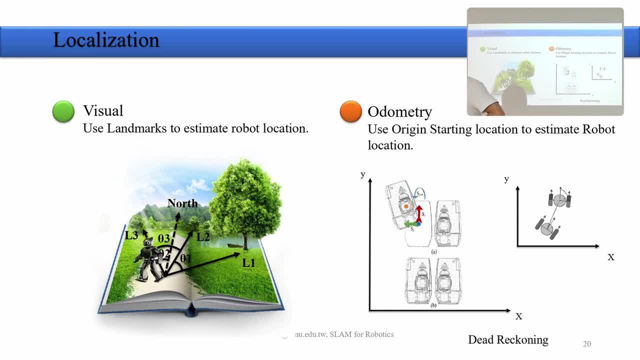 Okay, Okay. so so We have IMU sensor in robots. that is very common to use. What does it mean? It means that so you can, if I explain in simplest form- you have IMU. that is like kind of a sensor. Let me say this is the. 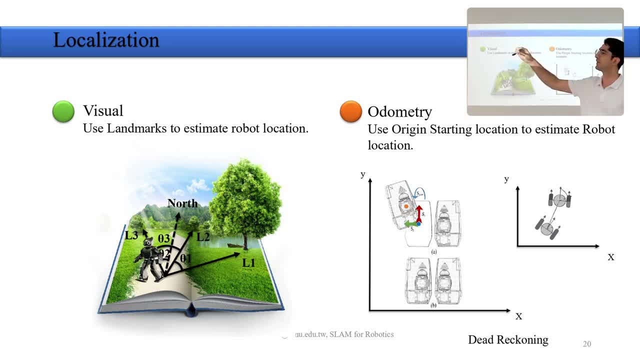 So consider, this is the IMU sensor. Okay, so you can understand amount of the angle of the sensor Based on degree. you can read it in X, Y and even rotation Z. This is three dimensional IMU that is very common to be used in different kinds of robots and 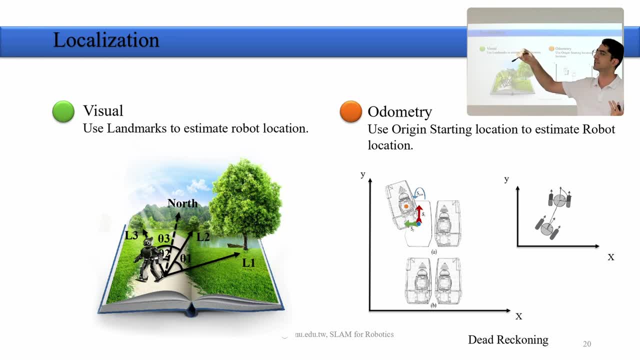 Plus those three that we have, this X Y Z, We can have amount of the velocity of movement for X Y Z. So three, four, angle three, four, velocity, for now, so far six. we have nine degree of freedom. I am used to that. Gives you more information, more parameters, but for now just consider the six. 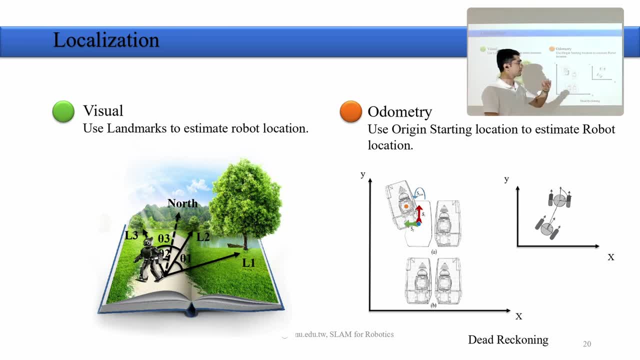 So whenever I'm talking about IMU, we mean that so that in in many of the robots we have it and And then robot is moving in the environment. and if you have IMU that can be made with, like I am, you Can be a third element that can be merged with. 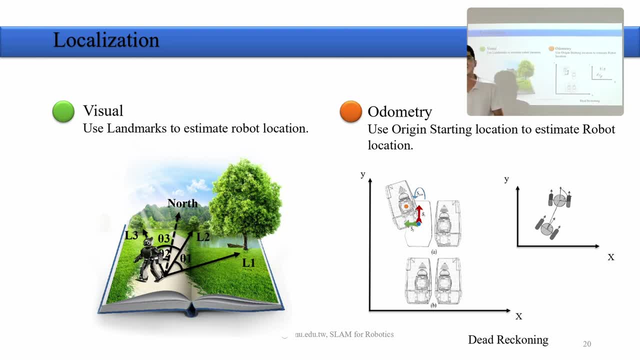 Automatically. and visual, and all three of these can help us to localize and not the environment. So no worry, We will break it down one by one. Well, how, how the metric can be work, how this can be work, and how The model of the velocity motion model can be presented in mass form. then later we can measure them all together. any, 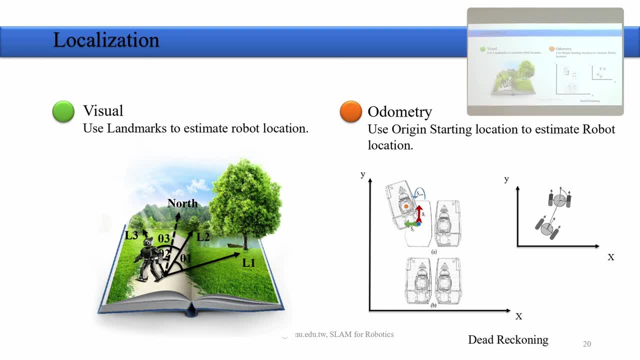 Any question? so far No. So I'm explaining some elementary topics, sometimes that in my view you already know it. If you don't know, please ask it. Feel free to ask, Because if you don't ask now, after two, three lessons. 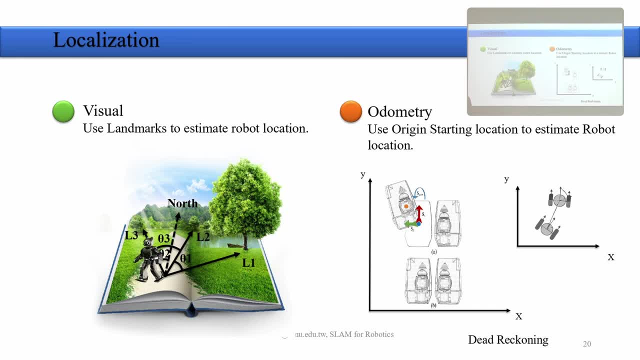 you don't understand anything more. All the time I'm going to refer back to those And the things that we are going to use. if I want to every time explain, it takes very long Because of that. please feel free to ask anything. 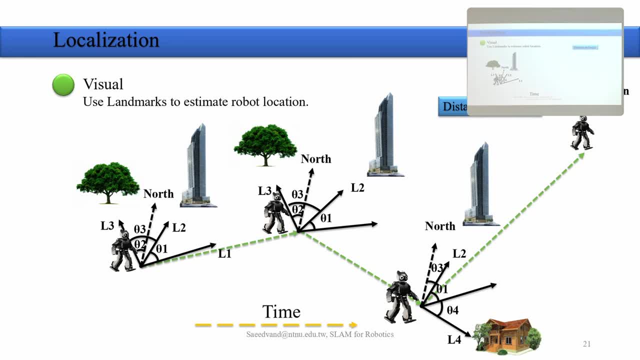 that you don't know what it is. So let's have a look at visual: What is happening and what are the general difficulties and challenges. Let's say we have a robot, This cute robot over there, Darwin OP. So this robot is walking in the environment. 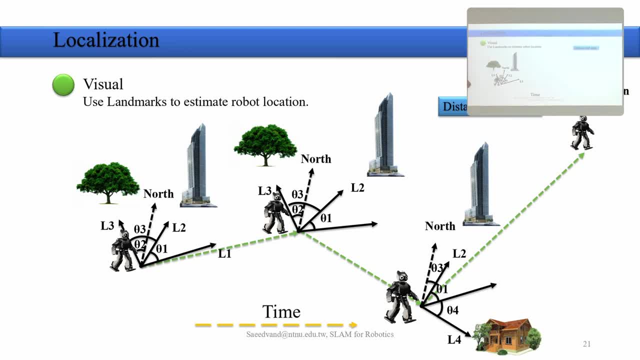 And we want to say: OK, let's use visual information to localize where the robot is. For now, we are talking about localizing, not mapping, Because we need to split them, So robot is moving. How robot can localize? As I mentioned last week, you need to find some landmarks. 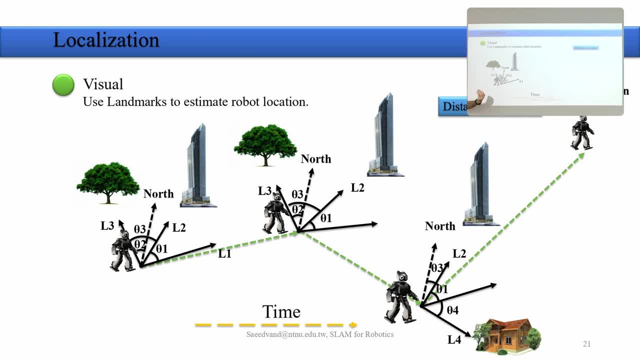 Robot needs to see some features from environment to estimate where it is Right. So these landmarks for now, as assumptions. say, robot knows how to detect tree. Robot knows how to detect building. Everything that the robot sees we assume that robot can detect for now, 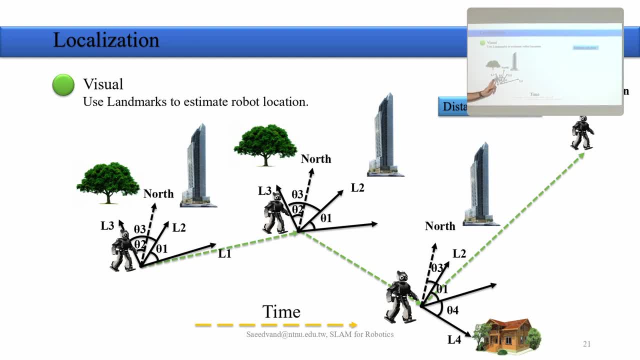 OK, Now of course, if robot is here can see these two objects, can do some mass calculation So that what is the angle of my body with my neck where I'm looking to the right, left, And based on that angle differences where the object is? 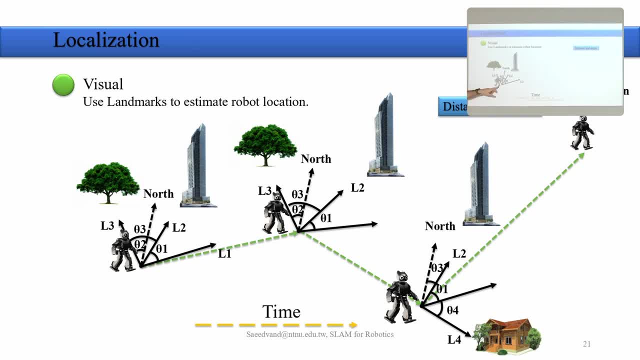 then where am? I? Can estimate the distance almost, and can estimate the angle of the robot. OK, So, based on these two, can say: this is almost north of me. This is the left side, right side, And we usually call them the different landmarks. 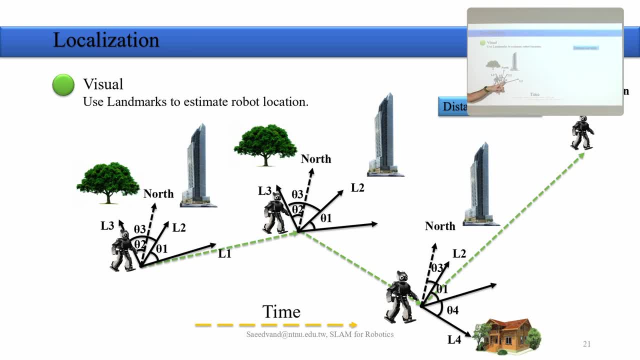 with L, L1,, L2, L3.. And for each one of them, some tetas that shows what they are. OK, OK, OK, What's the angle? But time moves and the robot tries to move to other location. 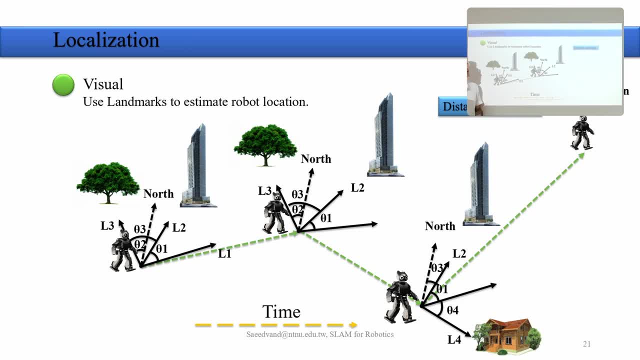 And after robot moves to the new location, of course, again sees maybe new landmarks, maybe the same ones, depending on this distance that robot moves. And we will now talk about this huge challenge Why? Because robot sees two landmarks here, moves there. 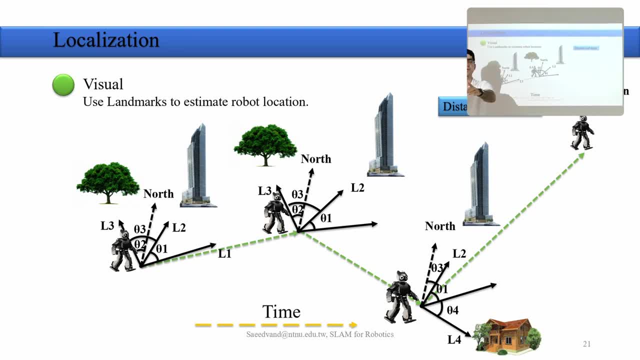 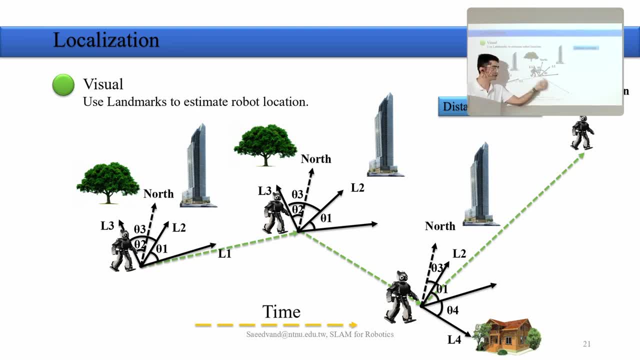 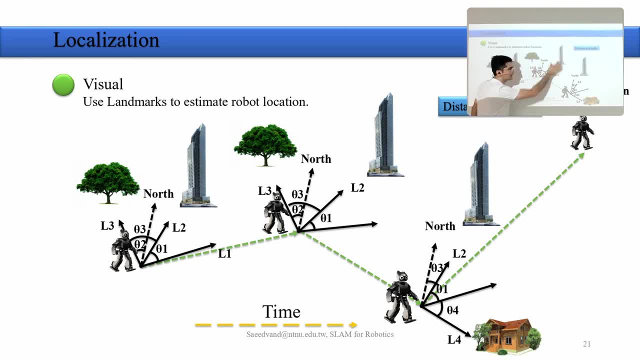 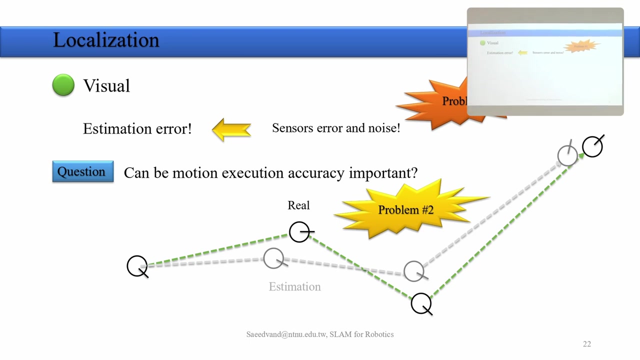 But whole scenario is like this: Robot moves, sees some visual information, tries to localize, moves, sees some visual information, tries to localize, and it is inside the loop Again: new location. So but what is the problem here? Main challenge that we have, we know that. 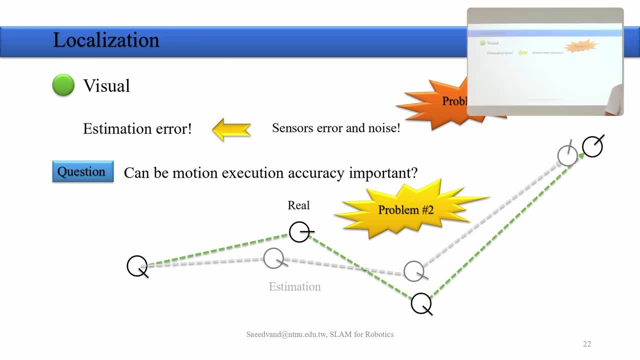 sensors have errors. You don't have any 100% accurate sensor If we have it in visual especially the SLAM problem already almost solved most of the part. But sensors have error, Not only sensor. because of the environmental condition you may have error. Robot is walking- if it's humanoid and his head is shaking. 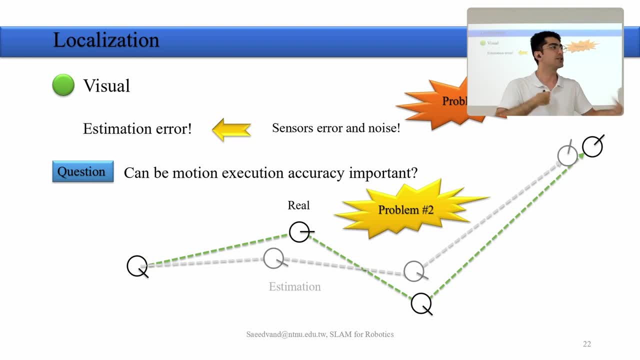 and that changed everything: All the parameters, all the distance estimation, everything is changing. Because of that, we have error And this error is called estimation error, And this is very important. All the efforts that we are going to do in this class- actually most of the efforts that we are trying to do- are trying to detect. 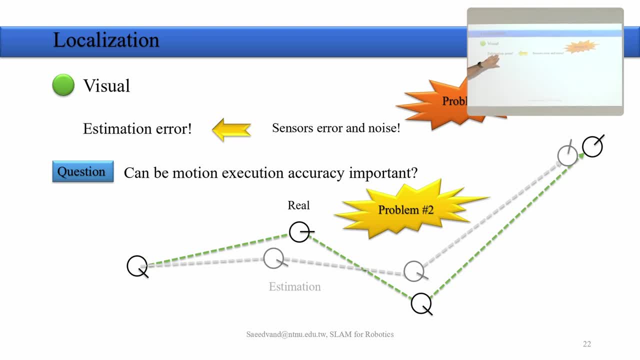 it and reduce it in our estimations. The question so, when we have the robot that uses visual features in the environment to to localize, can motions, motion execution accuracy important for us? Do you think, Depending on the algorithm that we are using, yes, it can. For example, for now, 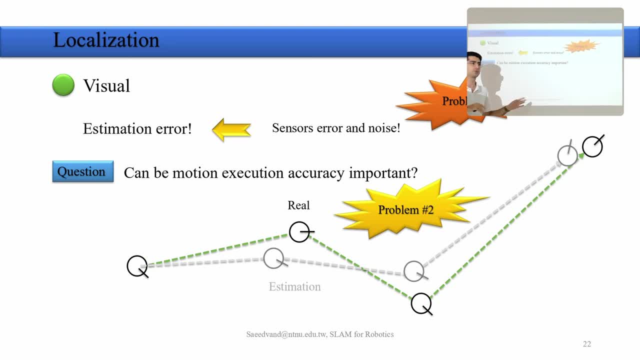 let's say I explained the odometry. We are going to see it soon, But in visual my algorithm says, ok, that laptop over there is two meters far from me, So I want to go one meter forward With visual information, visual odometry with visual 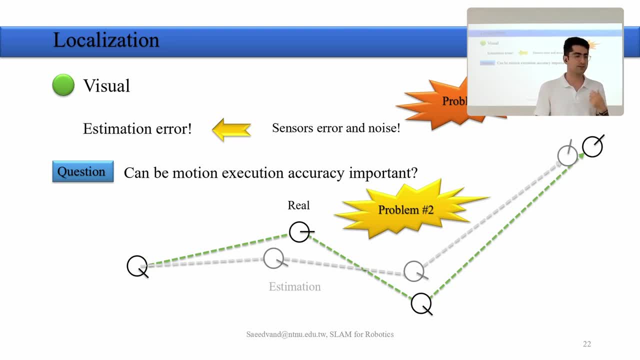 localization. I say I'm gonna go one meter, But my motions are running wrongly. Instead of one meter I end up one meter ten centimeters. Then that ten centimeter is the error that I have. that can affect the expectation of the visual estimation of the where I am. so let's say again: two meters. my let's. 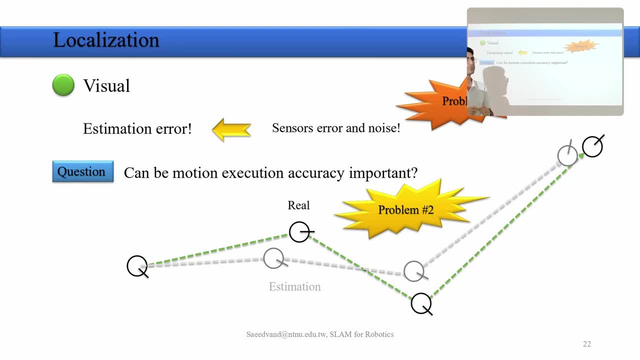 assume that the distance is quite 100% accurate. visual exactly can detect it, but after some movements, if my movements have error, then my estimation shows something wrong. it is expecting, like the laptop somewhere else and we don't know now. now that that also makes confusion. we don't know. the error was from sensor. 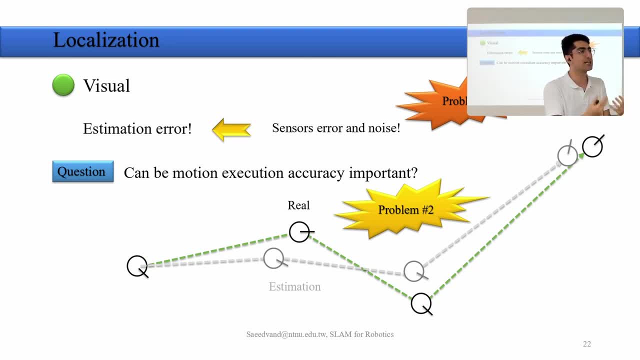 the vision or sensor error was from the motion execution doesn't matter about the automation, so when when you robot is moving can can ruin everything. if you have error for visual localization, any question? is it clear? ok, so let's have a look at visual demonstration of the problem. 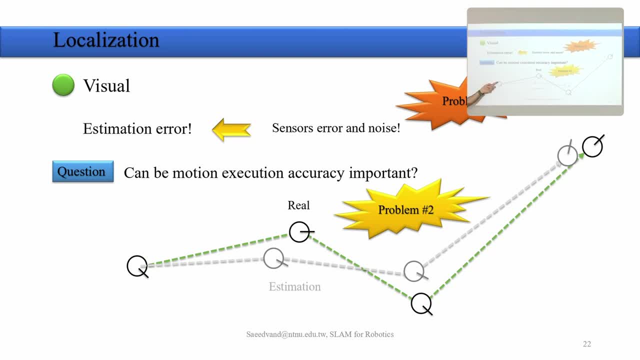 also we have the robot here. this is the robot and this is the robot is heading toward like here, then really like rotates and moves, hear, and from their rotates and moves here on moves there, like the. this is the real movement, but the estimation can show somewhere else based on the visual information that comes. 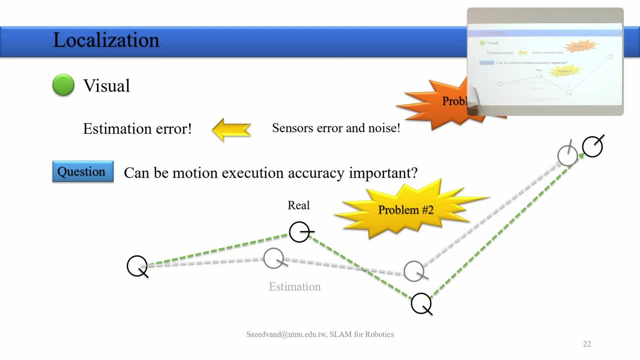 Why? Because if we assume our sensors are very accurate for detecting visual information 100%, that is impossible. but our visual information says that robot must be here, but we have error on motion command running and robot is over there. And this continues and we have all the time error of the localization, even for visual. 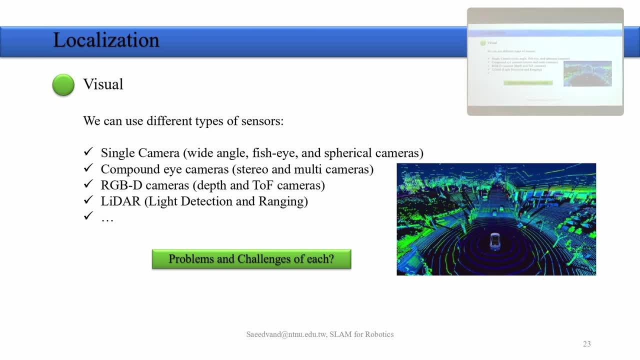 So for visual localization we can use different kinds of sensors. For example, we can use single camera, webcam- that already you all know. We have wide angle camera, Fish eyes and spherical cameras- different kinds of cameras that we can use. We can have compound eye cameras or stereo or multi cameras. 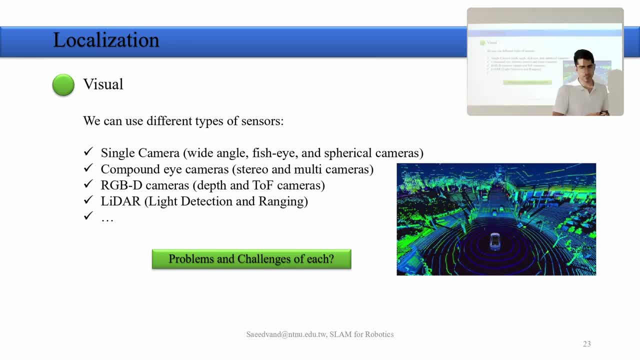 Stereo means that we can put two cameras together, but final vision is just one picture. What's the benefit? The benefit is not the angle of view. The benefit is that you can extract the depth of the object. There are some techniques that you can study on the internet how they are working. 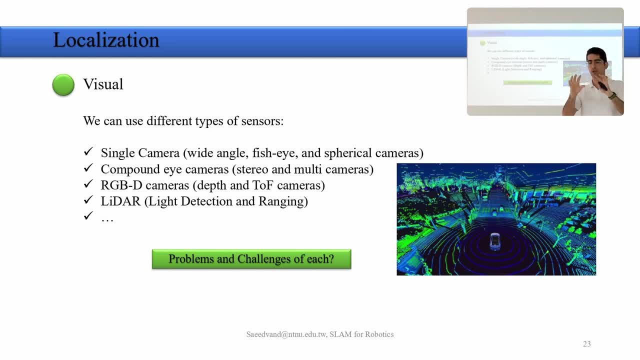 For a stereo camera. they put two cameras and based on this distance of the two lenses for each pixel that you can see, you can find also to calculate the distance of each pixel and estimate it. And now we have industrialized stereo cameras that you can buy them and they give you the estimation of the depth of the object. 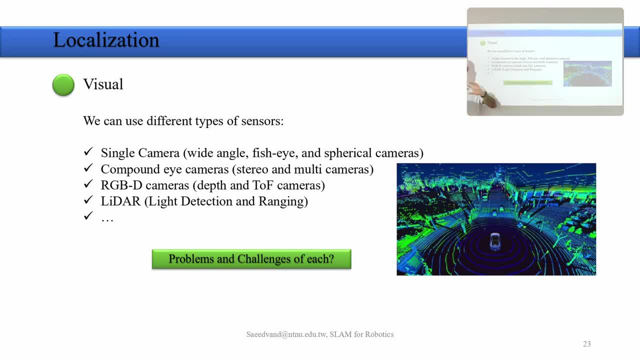 And now we have industrialized stereo cameras that you can buy them, and they give you the estimation of the depth of the object. They give you the estimation of the depth of the object, The anchors are guided through the lens and trying to see the depth of each pixel too. 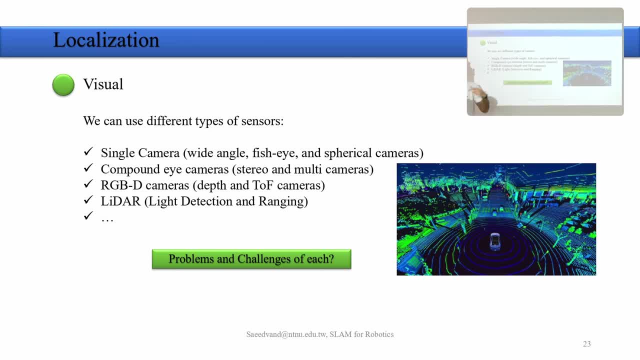 But with multicamera, you can put multicamera and use them as visual infomation, as input for your problems. On the other hand, we have RGB cameras. that RGB is same RGB similar to simple webcam, But it has depth sensor 2 inside that. 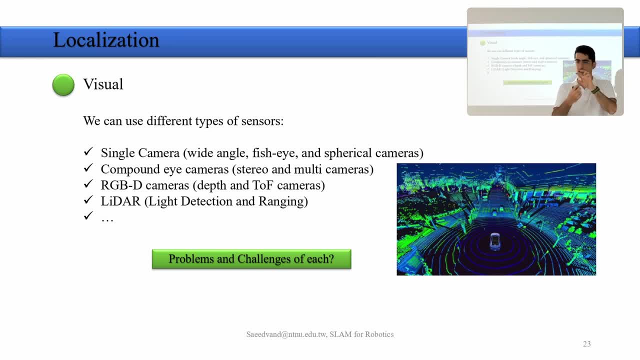 But it has depth sensor 2 inside that camera and some techniques- depending on the kind of camera that we can have also- that can give you the depth for each pixel. You know, for each camera, for each picture we have, is each pixel, that each pixel contains three. 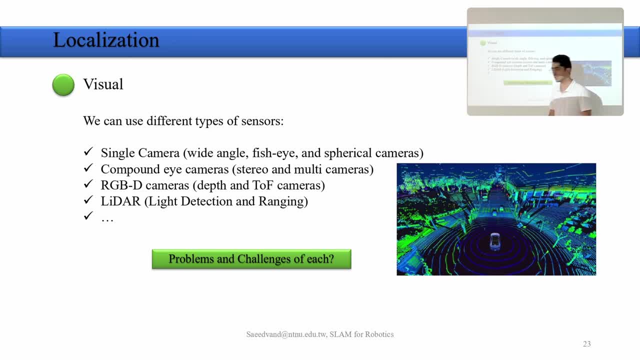 colors, RGB, but these related to depth and one more information of the environment that we can have. And also we can have LiDAR as light detection and ranging that is usually used for measuring the distance of the environment. So there is no color, basically, and you can stand the environment and get the 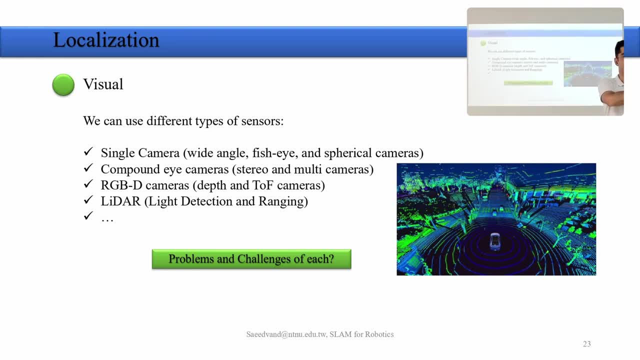 distance of the each, like if you have Raytrace like this can one line of the environment. then we have different types of LiDAR that can he scan one line of the environment. So if you scan one line of the environment, you can get one line like this, depending on the angle of the sensor that you can have at each moment. 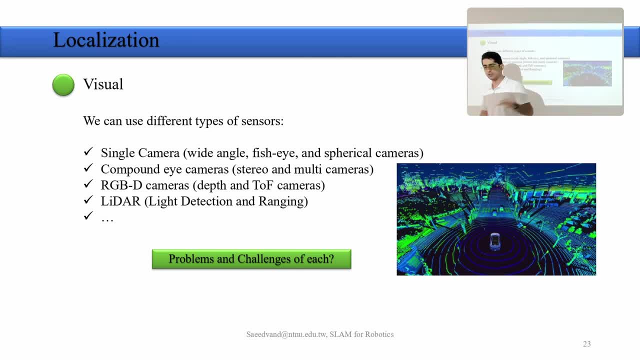 i have one slide later i will show its internal structure and how it's working and how there is like uh, there is a motor inside that rotates, the, the laser point you can. you can consider like uh, lidar scanner, exactly similar to laser point, but it it moves quickly, all the time moves quickly. 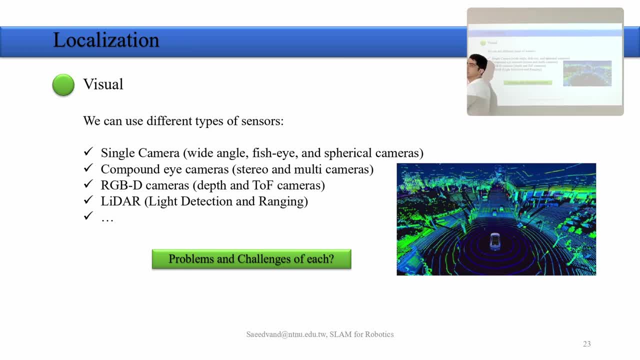 and each time measures the distance based on this, uh, this red point that it is there. so now, if you want to scan like environment, like this distances, it moves, like this, and if you want to scan whole in 3d, so we have two options. if you have sensor that it is like just one linear one. 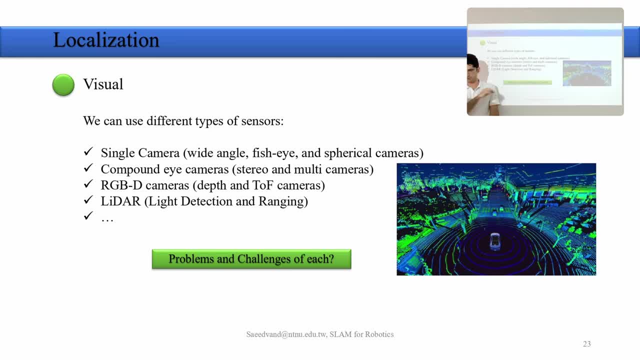 then we need to do it manually each time, like from here, do this, and then next time go upper, do this, go upper, do this, go upper, do this. and with the resolution that we move that, move that line, we can scan whole environment. so this is one kind and we also we have 3d one that 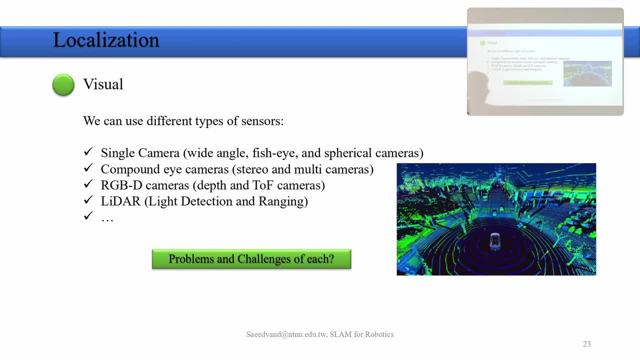 automatically does this and it scans whole environment. so why we are talking about details of these? because we're going to formulate this in math. we want to use it in- uh, in our algorithms in order to finally say where the robot is. you will see, we have mesh of those points. 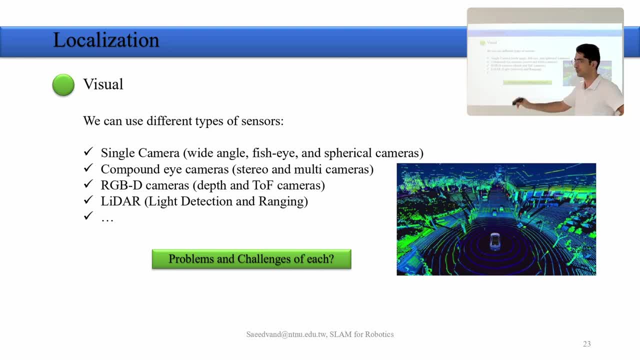 so let's say you, you, your robot, scans the environment in 3d. then you have mesh of those points. then we want to say, okay, where the robot is. in all the matrix of distances, we want to say where the robot is. so that's very interesting and that's very nice in industry and nowadays. 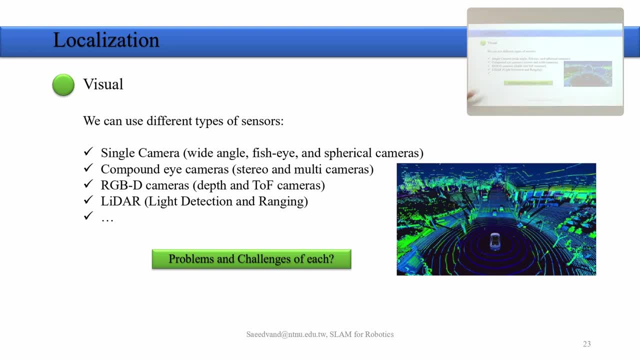 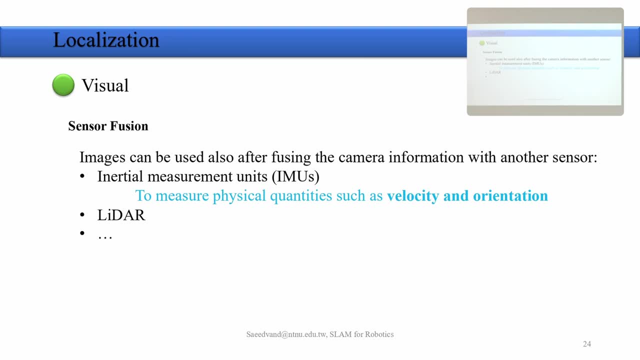 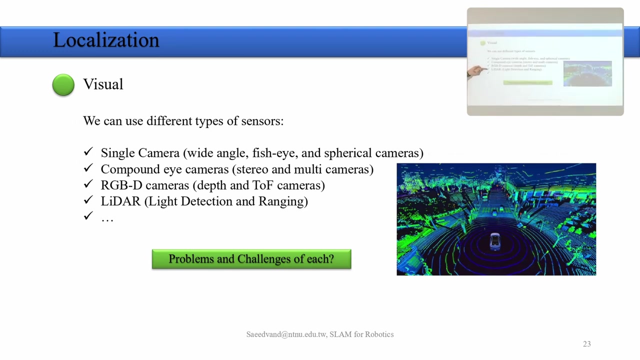 everywhere, uh people trying to use it in high level, robotic developments for visual uh localization. we have some also topics that we need to know, for example, sensor fusion. who knows what is it? sensor fusion says, okay, let's say, my robot has not only one type of these sensors. 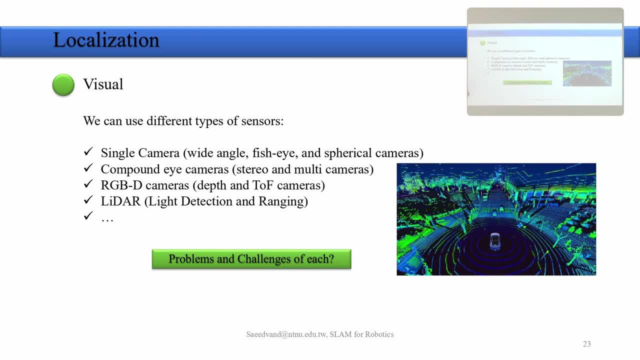 my robot has like two of these or three of these. then, for example, i have lighter and i have single camera. how can i connect these together? how can i say: okay, my robot vision sees um, sees tony, this is student over there, my webcam sees him and and my lidar scanner also gives some distance from there. how can i make? 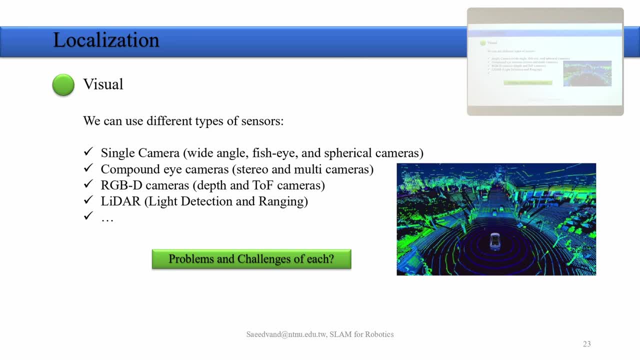 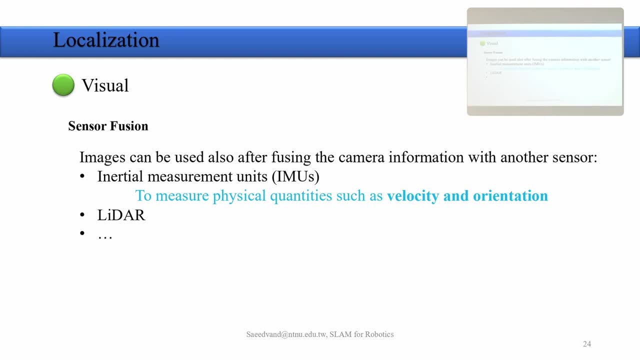 these two combine these two information together. that's called sensor fusion- very interesting topic: research study in the world. also just google sensor fusion. go to the google scholar search sensor fusion. you will see many algorithms over there. that that's how we can do that, how we can merge those information together. 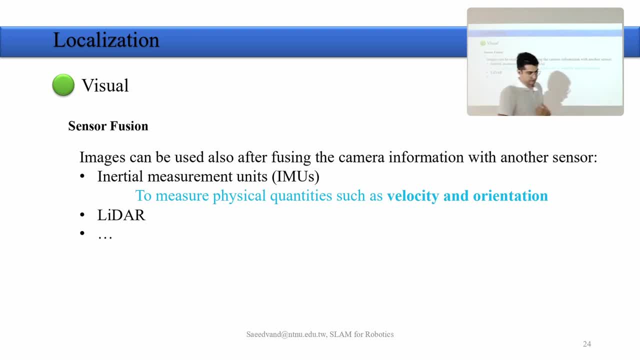 so, in addition to, in some techniques, if you study, you will see that, in addition to visual sensors, we also can measure it with initial measurement unit, or imu, so that it can give you a more precise vision of the environment. what does it mean? it means that, let's say, i have webcam and this webcam looks at the environment and i can measure it with micro lens. 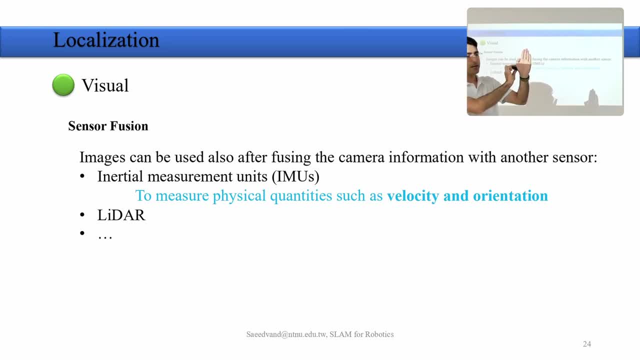 let's say i have webcam and this webcam looks at the environment and i can measure it with micro lens, I can move it And if I have IMU here, this can give me a lot of information, right Based on where it is looking and the velocity of movement. And if I can merge IMU information that I told. 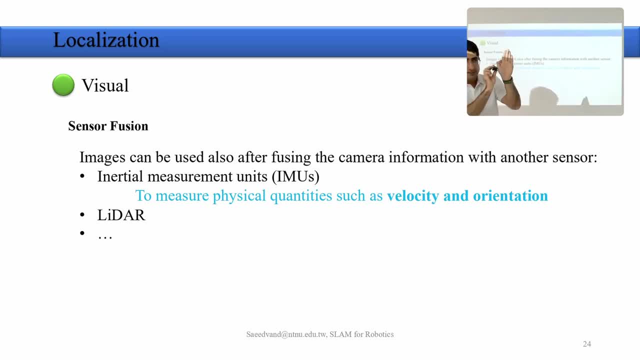 you. it can give you the angle of the rotation and velocity With this camera. how important it can be for especially SLAM algorithms, Because then you don't have single camera that looks around, You have IMU that can give you a lot of information: what is happening in the environment. 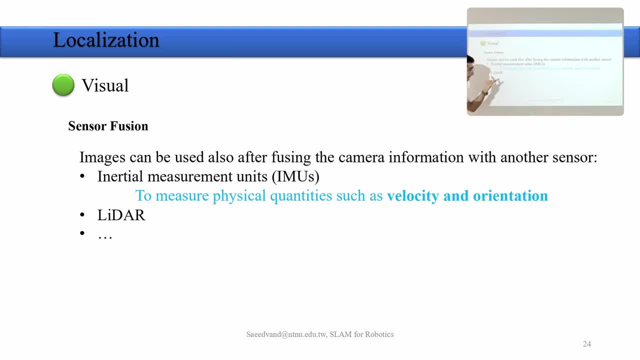 How we can merge these together. We will also discuss IMU combination with in form of sensor fusion or etc. The same sensor- IMU can be waged with LiDAR, can be RGBD or any kind of visual sensor that we can have. It can be merged. 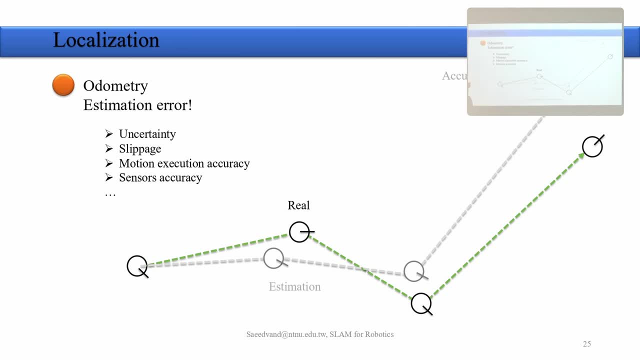 Okay, now for a few moments, let's forget about the visual. We want to talk about now: odometry, second part of information that we can use for our robot localization. First of all, we need to consider the estimation error of the odometry. I already explained you what is the 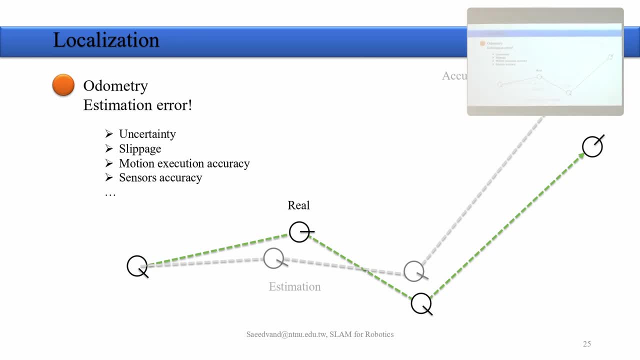 odometry. I'm walking in the environment and if I can measure how much I walked, I can estimate where I am. This is very clear. What is the problem? The problem is the estimation error. And this estimation error comes from where? It comes? from uncertainty, It comes from slippage. 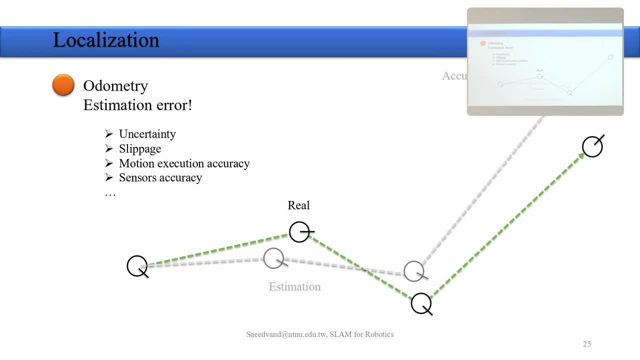 It comes from motion execution accuracy, It comes from my sensor reading accuracy. All these together can give me can cause error of the movement. So so that you see the same example here, that our estimation is different, but here is based on the odometry. 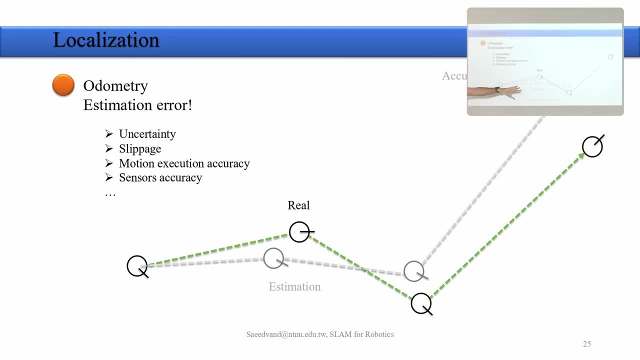 So in previous one we were talking about the movement, but here reading of the information, not just specifically just motion execution that we were talking about. last example: Here the combination of all those can cause error, But the most important part is the accumulating error that 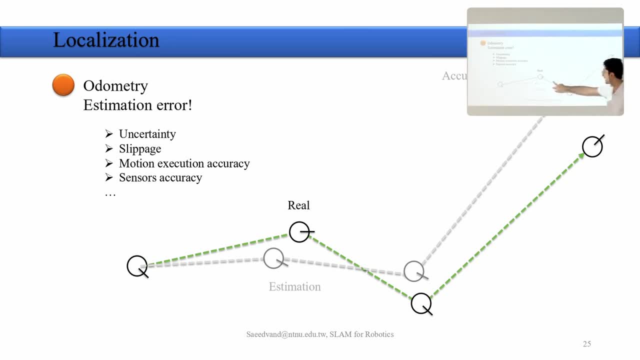 finally can happen. Here the most important part is the accumulating error. that finally can happen Because every time the error is happening, it is accumulating and it is growing And if you continue this, you see that robot is here. Maybe the estimation is over there. 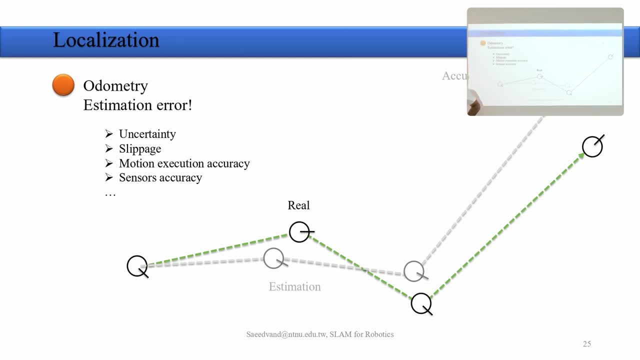 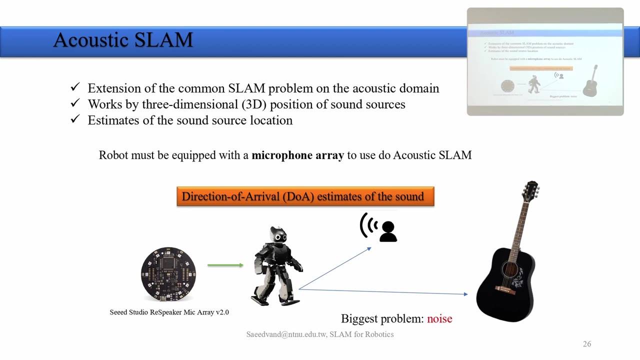 Any question? Is everything clear so far? So we split it visual and we split it the odometry and we understood the basics of what is happening there. In addition to those, we can have some autistic Islam, that it is also open problem and very nice. 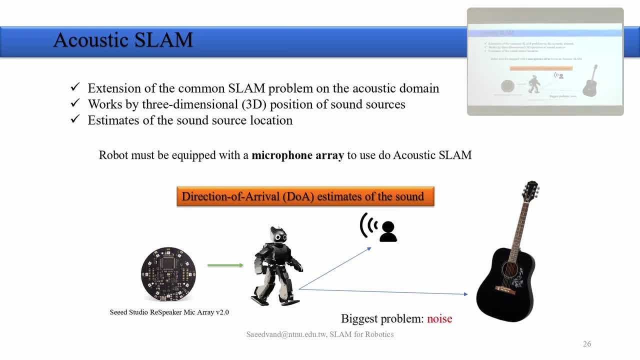 example of localization. We have some kinds of sensors, like see the studio boards that they have multiple microphones in around it and it can measure if the sun is coming, what is the direction of the sun and if there is any movement, If it is the direction of the sun. 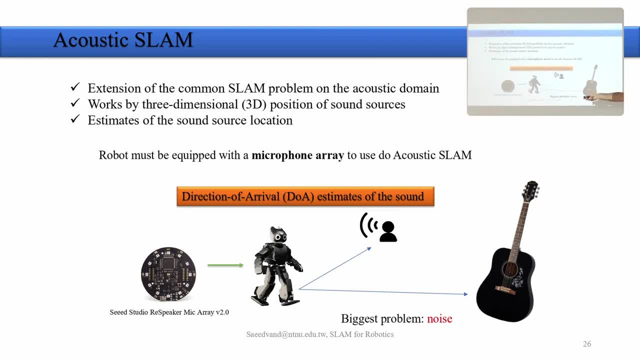 of the sound and if you can use this sensor inside your robot then, similar to human, you can detect where the source of the sound. if some of you are talking, i can. if i close my eye still, i can say where that person is right and and this information. 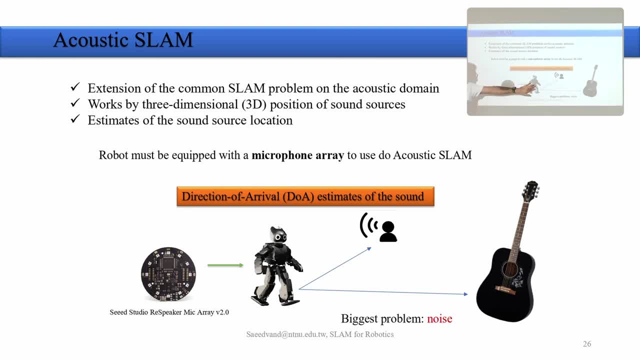 can be used by robot in order to localize where the landmarks are, is similar to you can imagine a blind person moving in the environment and hears everything and knows where the car is coming. what is happening around now? ah, this is like open problem again. open problem is a problem. that is in the world, is still challenge and everybody trying 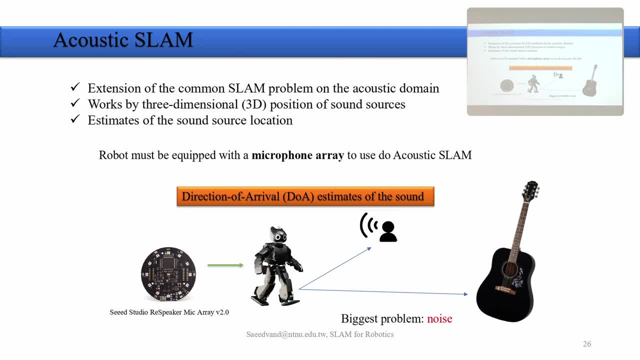 to solve it. we don't have algorithms that can merge this with other islam algorithms. well, yet have you heard that this robot can also localize by hearing? not really, this is very advanced, that you can research on this topic also in future. so we call it as microphone array. that, and the technique is autistic islam. 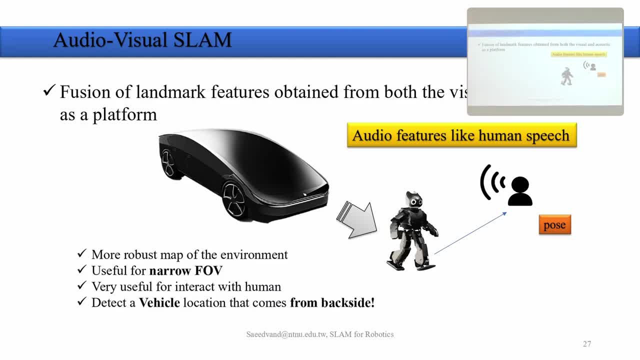 for example, fusion of the landmark, then can give robot more ability that it can move in different directions. for example, if if robot is localizing based on the camera or rider's camera or whatever, it has limited field of view that sees just from like human. but if a 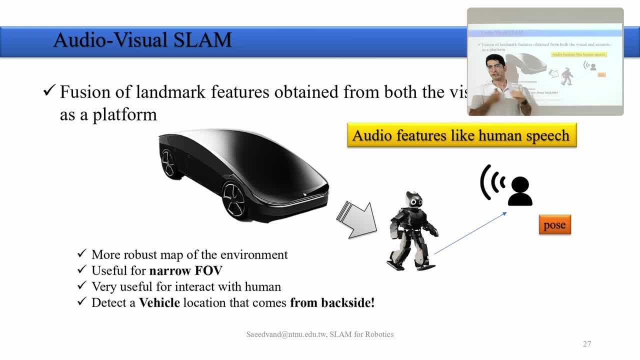 car comes from backside, then robot has no idea mostly, but human does. then we can give that capability to robot by adding that sensor, using sensor fusion and how it can happen. try to open it later. Of course we have to go to math, have to go to algorithms in 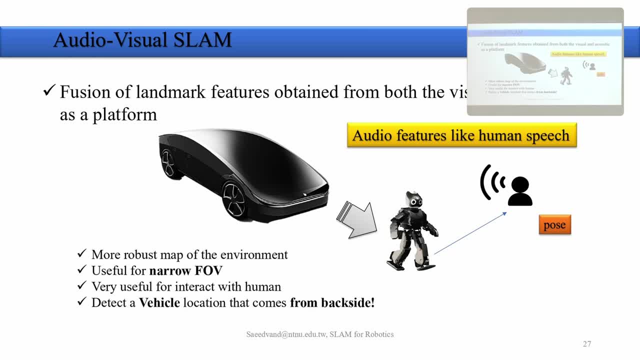 details how it can be come to our our system and how we can manage it to be. Let me see what points we have here. More robust map of the environment, useful for ah. one important point also that we can have: you can detect hidden objects. so 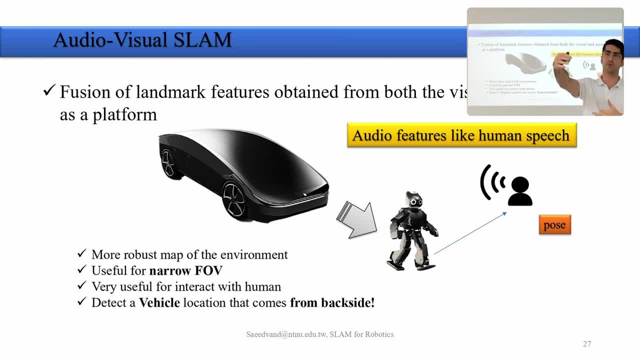 there is some, some object behind the other object. human can hear the sound and detect it, but robots so far can So like, like if something is on the table, some cat is there moving, I can hear and localize where it is, but can robot do this? Not any robot can do this. We can also try to use those information, but of 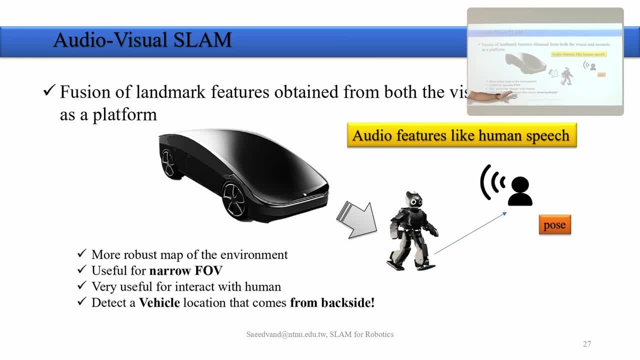 course, still we have problem of the accuracy of those sensors. Those sensors still are not very accurate. For now we can have the angle where the sound source is coming, but not very accurate. And of course, if you are familiar with advanced algorithms, deep learning algorithms, later on that can be used as estimation. 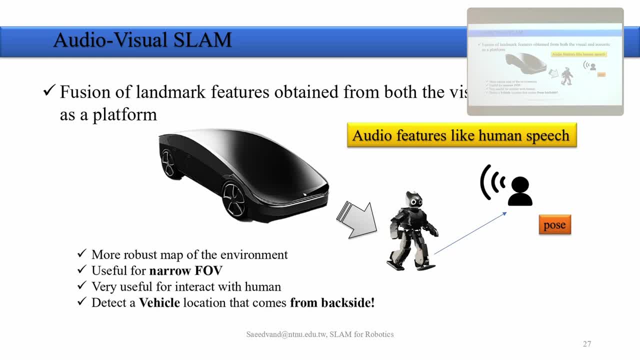 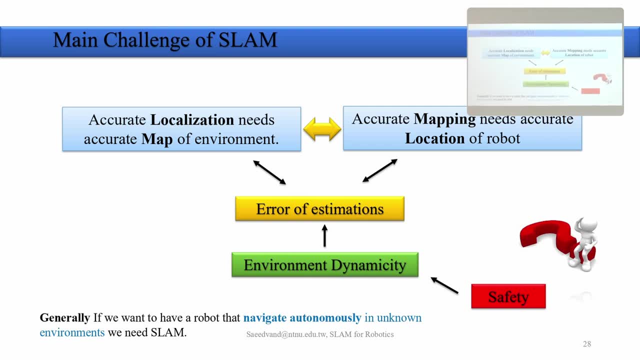 of the, where the source of the sound is. So we said: we have the localization that needs the map and we have the map that needs the location, and this was chicken egg problem. they need each other and both of these. so that's the one challenge that we have. they need each. 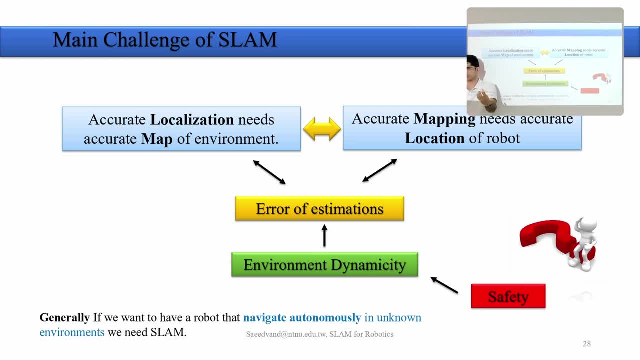 other in our course- localization and mapping- And when they need each other. meanwhile also, we have the error of estimation, Either in mapping either in localizing. so this, both of these error are- we will clarify later also what. what's the mapping and the problem that we can have. 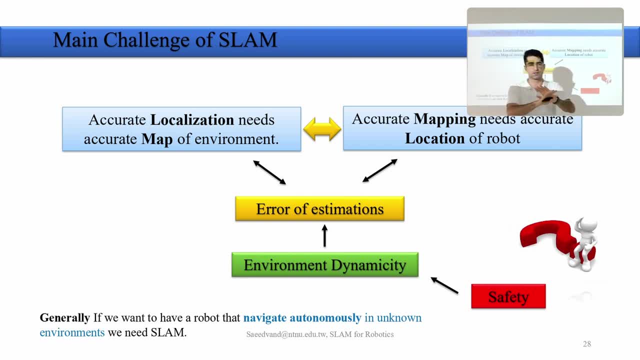 there because, simply you can understand if I want to explain quickly: like you have a map inside your robot, like I mean the brain of the robot or the memory of the robot, you have the map and that map is not accurate. After a while you have another map of environment and that has that is not. 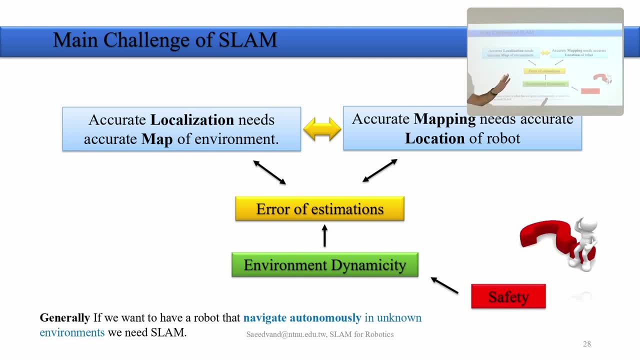 accurate too. So these two inaccurate maps, how should be measured together? So that's the error of estimation inside our did. the map of the robot that knows from environment? And besides all of these, where is the more challenging part? is dynamicity of the environment. 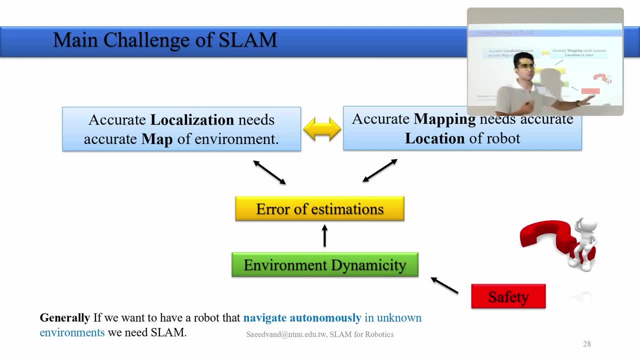 now let's add: not only the robot is moving, the objects, landmarks in the environment are moving too, so that creates more challenging part. here, of course, we will simplify and we, as I assume that we don't have dynamicity at the first, but later on we will see how we can add it plus, though sometimes we 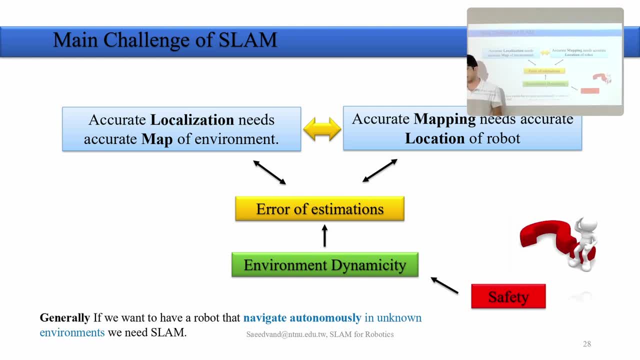 have safety problem, that that that is crucial in some applications, for example car application. or robot is moving in the home. let's say you built a robot that works in the home environment and there is a kid there, then they should not fight each other, right? if robot wanna keep the kid, then the mom. 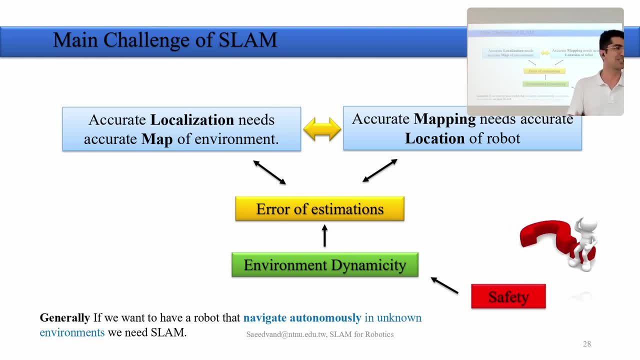 comes and keeps the robot and as engineer you are developed. you will be punished because of that. now you need to know that. okay, I'm trying a lot to develop slam algorithm, developing complex algorithms. it works very fine, but I didn't consider safety and my robot is doing something that. 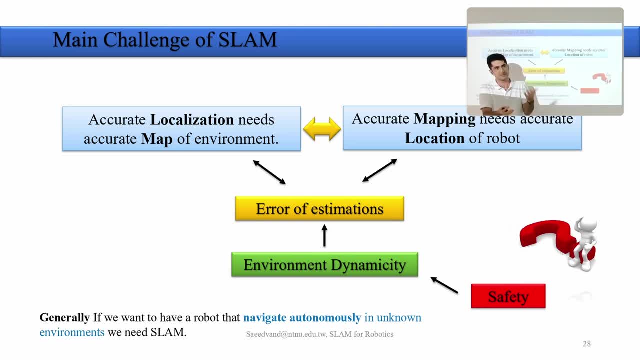 like kid is, like big human is different from kid. like it tries to push the buttons, play with the robot, jump down, throw something, then you need to consider it in your techniques and algorithms. We have general definition of SLAM that we say: okay, the environment is the. 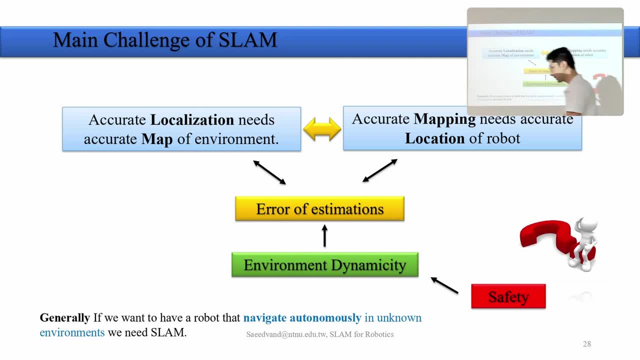 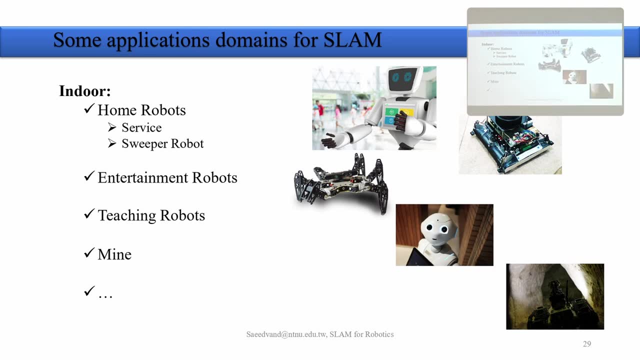 environment is unknown and we want to localize and we want to construct a map. we need SLAM. That's the solution. So what are the applications? Already, you know, we have home robots like service robots. we have sweeper robot that needs to sweep. 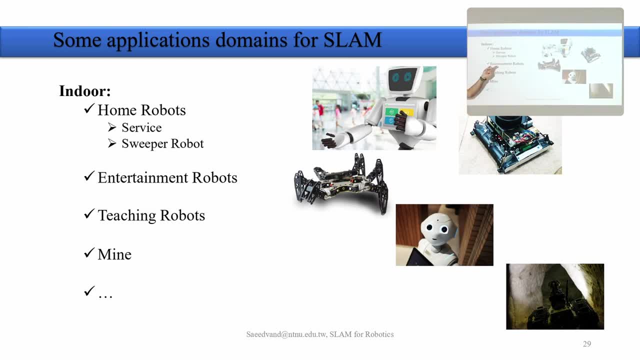 the environment like this robot is sweeper. we have entertainment robots that they try to play with other people. of course they need. if you have a robot that try to tries to play with different people, If robot is on the table you can have some sensors to: okay, don't fall down, but it's better to have local. 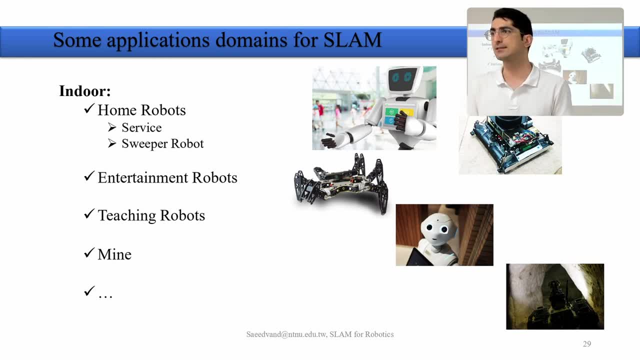 the map of the environment. if you want to do interesting things, it's much safer. smart things better to be able to localize where it is and construct a map. Then robot can memorize where was the charger, can charge itself. This is very nice application, for example: 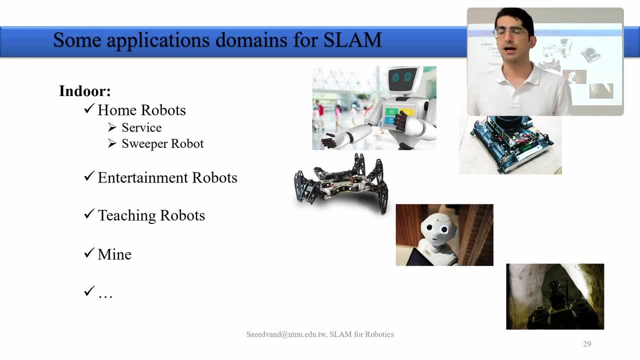 Or then, like there is a pen and you want to ask robot, go, bring me pen. If robot is able to construct a map of environment, then can know where the pen is. This is next level of robotic applications If you want to move to the next. 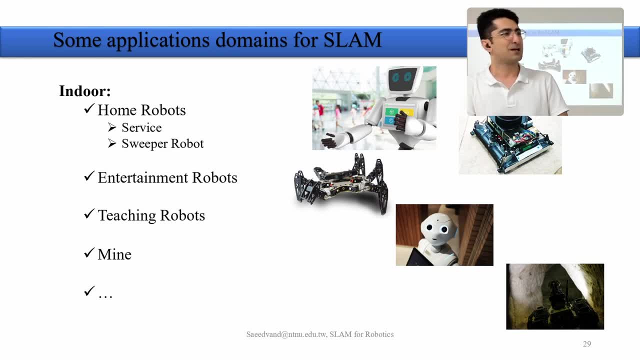 don't stay on stupid robots just if else is some distances, if this is stop or like, like very simple robot that we have, we need to move toward that direction. I mean from simplicity when it can be humanoid robot, But if your algorithms, techniques are in level that are not upgradable to. 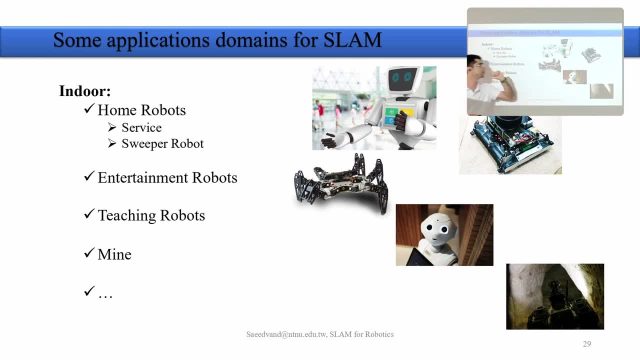 algorithms, then it is not a robot. But if your algorithms techniques are in level that are not upgradable to algorithms, then it is not a robot. Advanced topics: then we need to understand and move to that direction. Teaching robot: let's say you're going to replace me with another teaching robot. 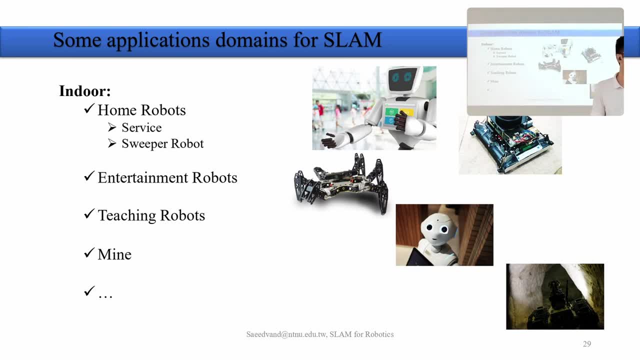 So better to know the location and where the robot is. otherwise the robot moves. It stood here and just talks one, two, three hours, then it moves back, Or maybe a little bit of movement with some sensors if you wanna have really a robot that can interact. 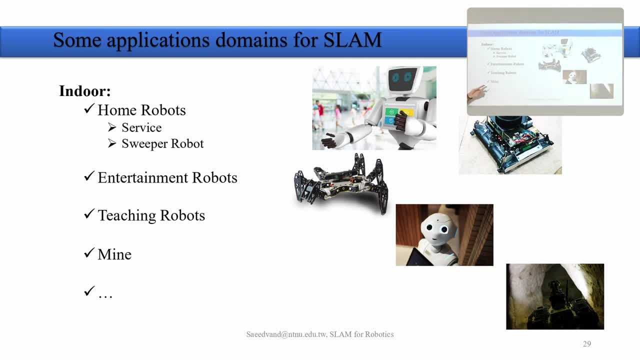 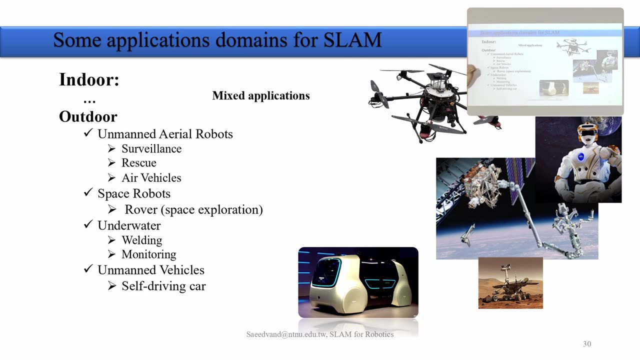 environment pretty well, even if it is teaching. it can be used in SLAM, in mining application and so on. We have many different. So in indoor we talked. outdoor it can be unmanned aerial vehicle for different applications. You can see different applications here: surveillance, rescue air vehicles. So each one of these. 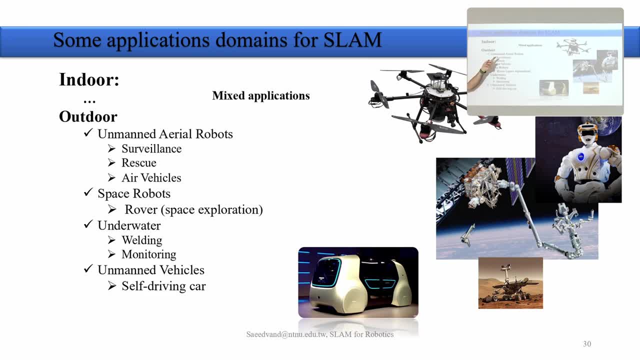 if you search on the internet, there are different challenges and different algorithms. try to solve surveillance, try to solve rescue. Now think about it like a disaster happens. robot is going to try to help people If really it want to happen. robot needs to be able to localize. 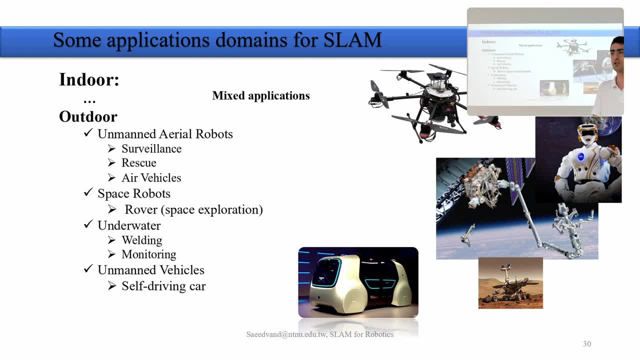 and map the environment first, because everything is changed. Earthquake came. you have very advanced robots And you want to use that robot to help people. How you can do that For rescue application. of course you need to be able to implement very nice SLAM algorithm first. 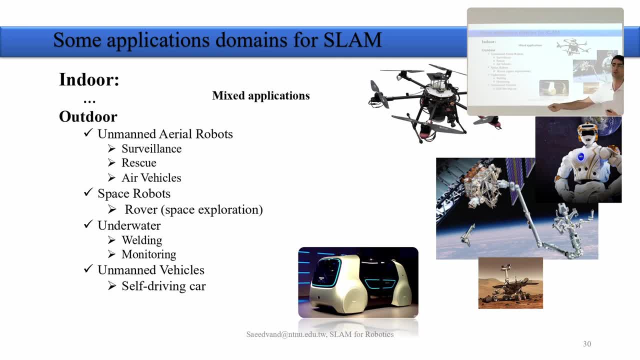 then say: okay, this is the guy that I need to help to rescue, That guy needs medicine, That guy needs ambulance. So also we have space robots. You can see the Robonaut 5 here. This is from NASA And a couple of years ago there was big announcement: competition. 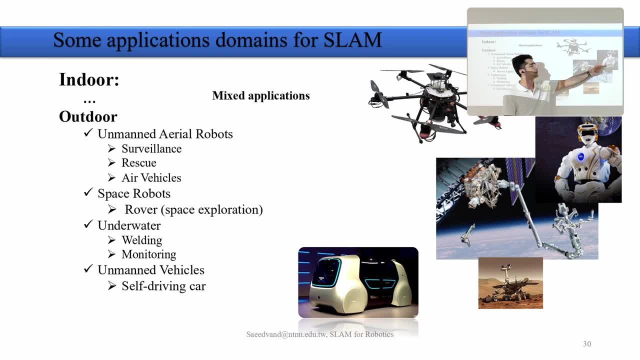 I think one $2 million for the competition that everybody could join. Like you could have make a team to join That. the challenge was like there was a simulator for Robonaut 5 that you needed to program it in order to do some missions in the space. 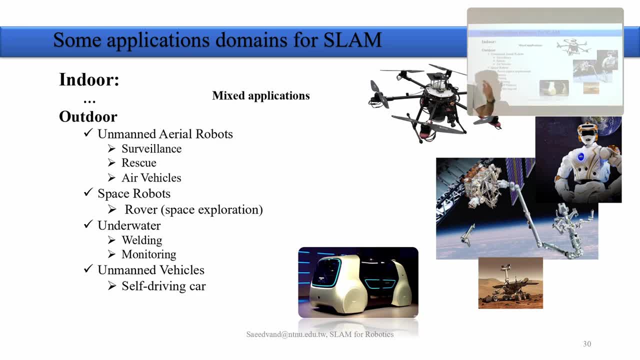 Then team was competing against each other And the winner had the chance to go and program directly the robot and work in NASA to test the algorithms And if it was successful they were going to use it in space applications. So why we are talking about this? because we have same SLAM problem there too, right? 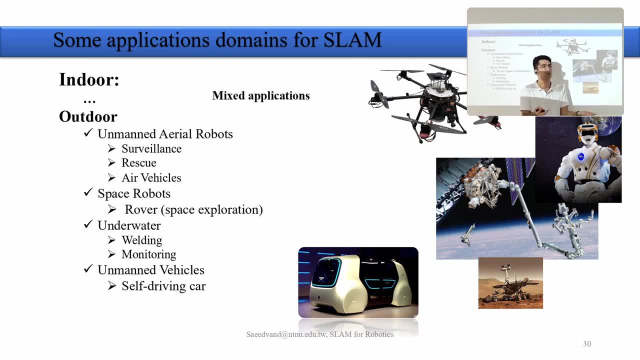 The environment is unknown. Robot needs to localize where the things are And map the environment and then start to do something. So this shows also importance and how important it is. in future, Of course, we can have different kinds of robot And, most importantly, that is right now is applicable and 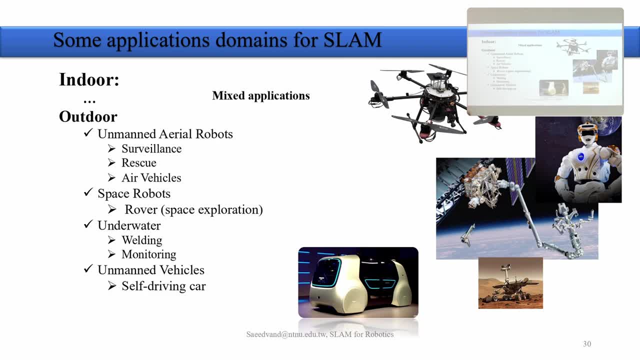 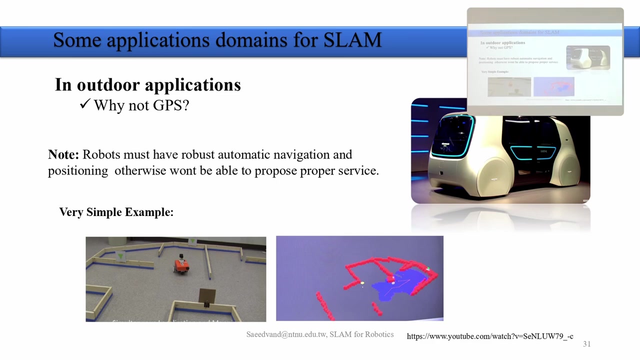 we are luckily able to use and try is self-driving cars that Tesla and Elon Musk are doing a nice job there. But still we have lots of challenge that haven't solved yet and it can be improved. So in outdoor applications, why not GPS? Because in outdoor, not indoor, Why not? 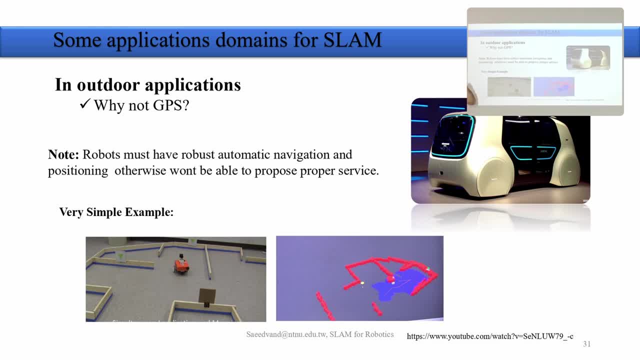 Because it's still. we have error on GPS, So the GPS is not very accurate. You have meters of error, So the GPS is not very accurate. You have meters of error, So the GPS is not very accurate. You have meters of error. 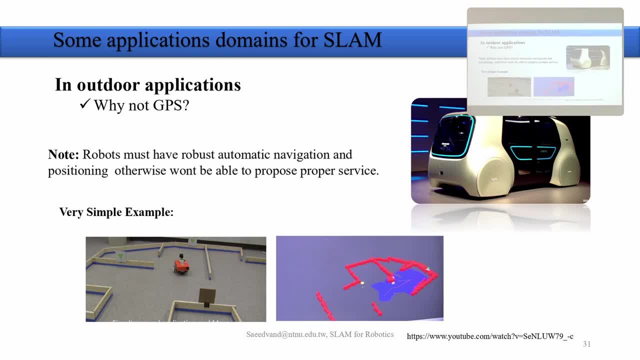 But you may say, okay, we have very accurate GPS too, But yeah, they are military and they are very expensive if you want to use them. Because of that, basically, we are not relying on GPS and also it can have disconnecting problems. 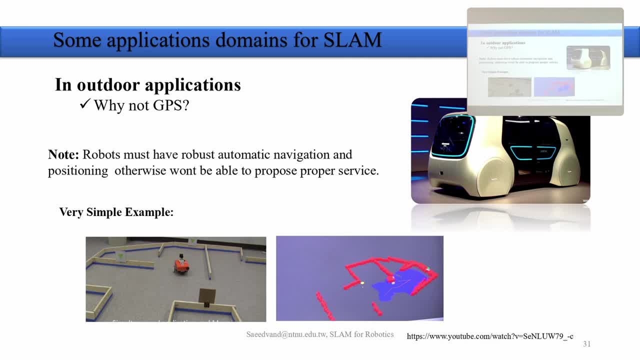 Then, if your robot is disconnected, what happens? Nothing. It stays there and dies. It should not be, So we need to have techniques to solve it. We have note that meanwhile we are doing and solving this problem. also, robot needs to have robust navigation and positioning system that can, as I mentioned already, of course, we have 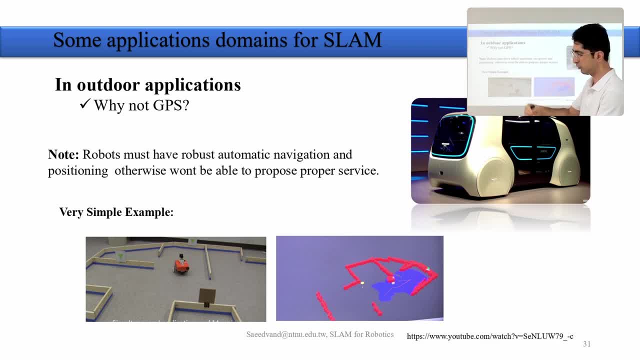 the problem of mapping and SLAM and localizing together. but also, robot needs to move in the environment in order to do something and construct the map and localize. and that moving how you want to say to move, think about it. how you want to say to move at the big first beginning. 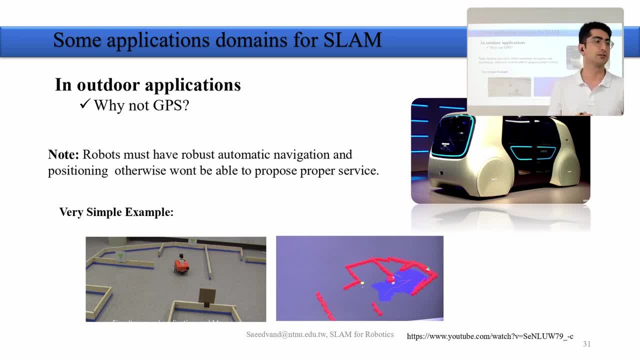 so you need to also have nice navigation technique over there that I will introduce some, you will see in 3D and I will introduce some tidy algorithms. that how? let's say: okay, I am a robot and my localization is very nice. one of SLAM course students. 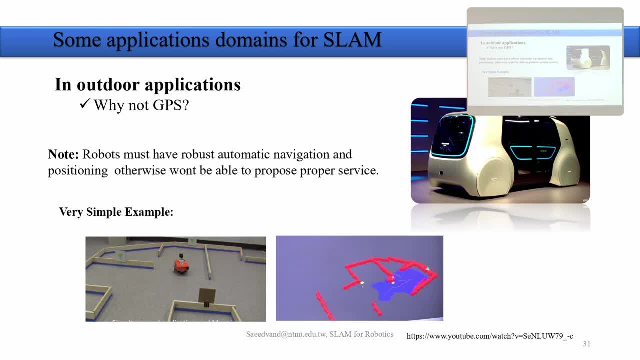 developed it and that works perfect. okay for localization and my mapping is work very well too. the other student from this class developed it and it works 100%. but now okay, how to? how to construct a map of environment. now just seeing like this is enough thing, like this is enough. 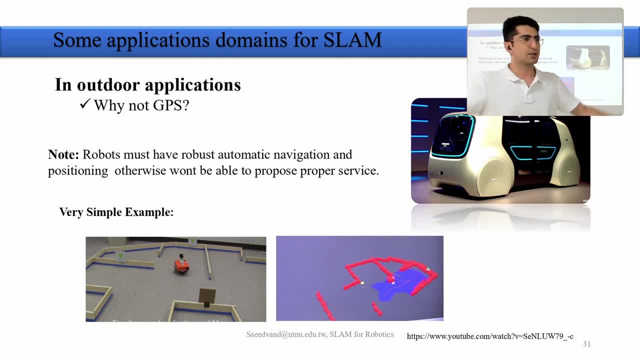 of course it is not. maybe I'm here I want to construct all the map of the environment, so I need algorithms, strong algorithm, to say what to do at each condition and each at each state. so you can see simple examples here that, like you can, if you have very cheap small robot with 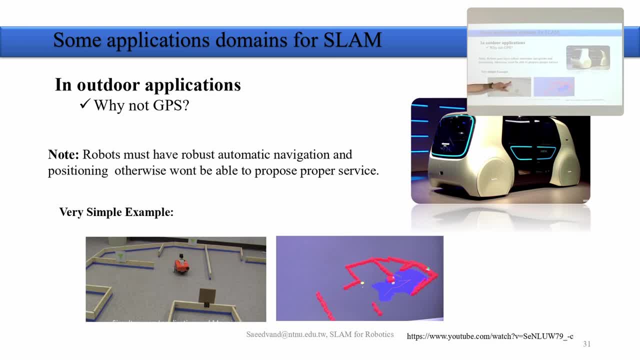 two wheels, very, very small one that it has one single camera, very cheap camera. you can construct the environment like this, build environment sample like this, wherever you are. then put some tapes over here, color tapes, then try to use like OpenCV libraries to detect those lines. then try. 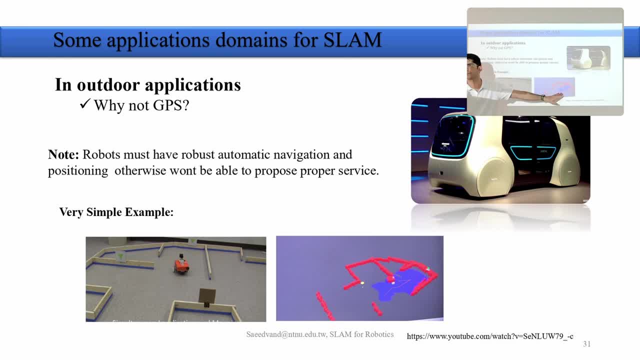 to construct the map of the environment. this is the the simplest example that you can do it yourself. whatever robot that you have that is moving in the environment, put a camera, put some tapes and use libraries or develop the code to detect some lines, then start to construct them. this is, uh, kind of a very simple example of 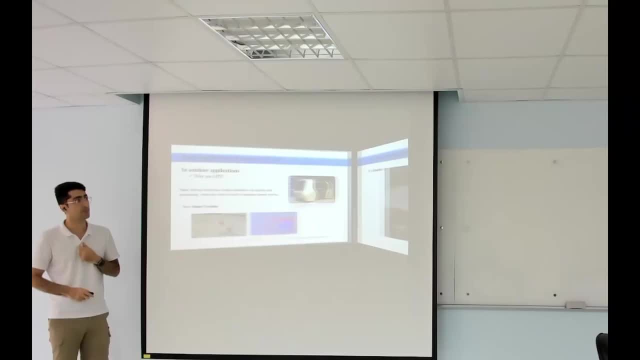 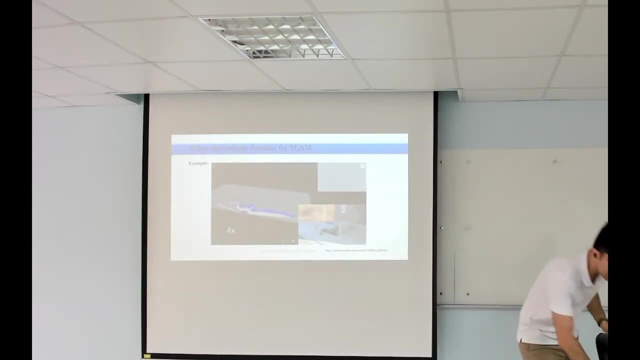 localization and mapping. here we have a video of how it works with drone robots. let me play it. it is a little bit more complex with 3D environment. you can see that drone is over there flying in uh into the dimensional in 3D dimensional, and it has. 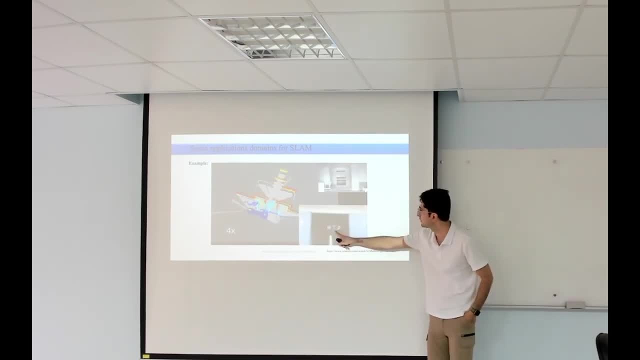 the lighter scanner and it scans the environment. you can see the, the camera here and the camera from robot, the other camera and the uh, the uh Islam technique that they applied to construct the map of the environment. and these green ones are the uh are the LIDAR scanning like this? as I told you, one line of the scan, just. 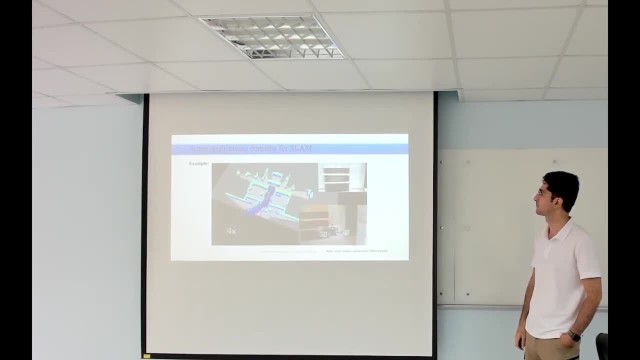 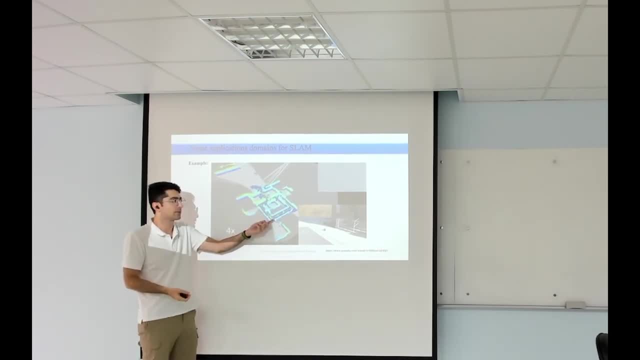 and as much as we can try to even understand what's happening, there are many things that are happening here and if you look at the code it's like big code. but anyway, like here we will later see, for example, talk about the occupancy grid mapping techniques- what does? 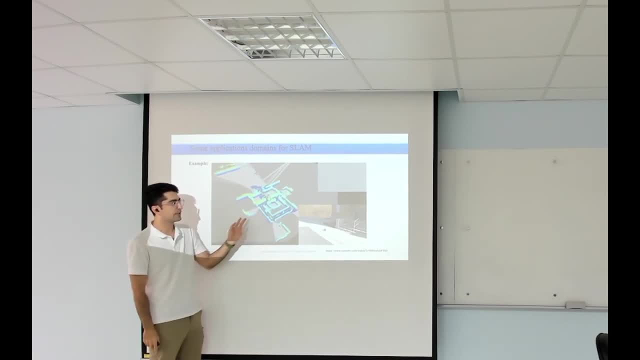 it mean you will see that, okay, we can make grid of environment and if you have our sensor can just measure the distance, like this, like this point, we can construct the wall over there and we can assume, okay, so when you detect something over here, of course it is connected. 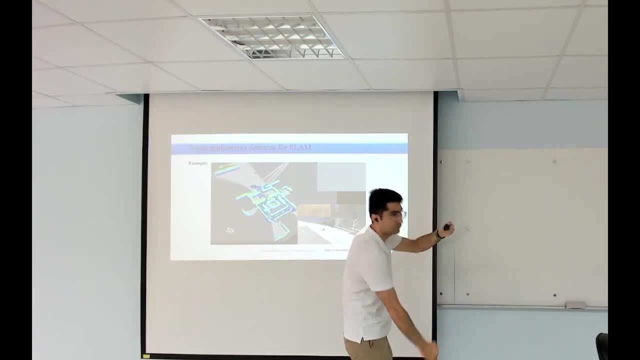 somewhere and we can say, okay, this cell is occupied with that one, and construct 3d environment like this and simplify the problem. i just want to give you intuition of the what's happening in simplest form, but of course we will see also much more advanced algorithms like icp. 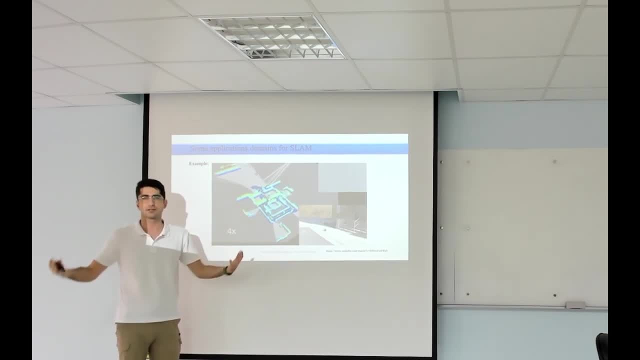 that we said and that's that's trying to show us how to do that, and that's what we're trying to do: merge 3d- construction of the environment- and merge it together. we will talk about any question here. can we have other applications, more complex applications or interesting applications? 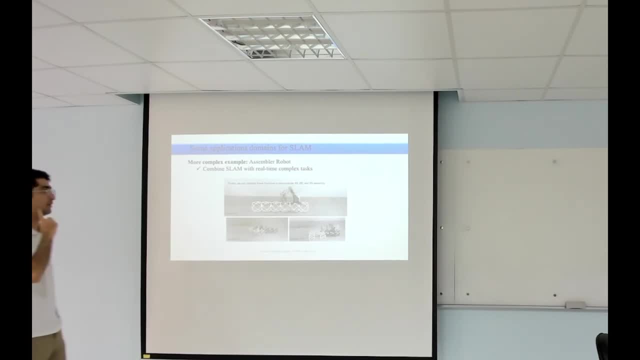 or kind of let me say, new ideas. let's say, okay, we have a robot like this that is trying to construct building or construct the path for himself, or whatever it is. of course, we can still use slam algorithm, slang techniques in such problems too, because this robot may needs to in the environment. 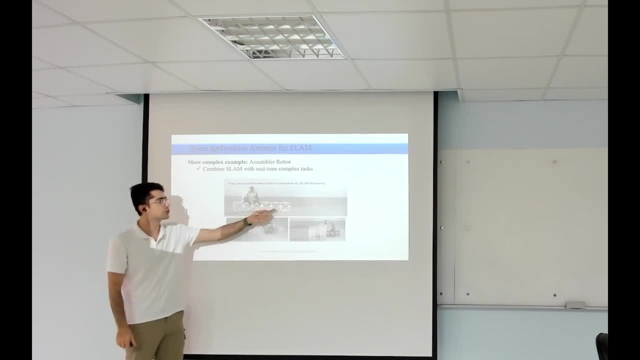 like this robot cannot work. only floor, for example, just needs to go with this one. And and, of course, if the Islam can scan the environment and if the environment is challenging, find the passage and use those items in order to move in the environment. and 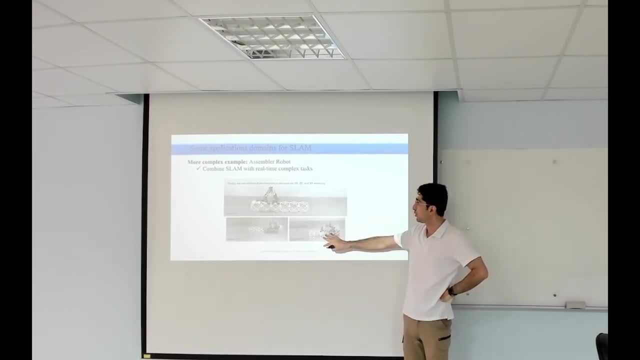 the Islam can be applicable. So, based on this idea, you can think a lot. You can use your imagination to imagine very interesting applications for this. For example, if we have a robot that cannot swim but has some objects. go on on the, on the. 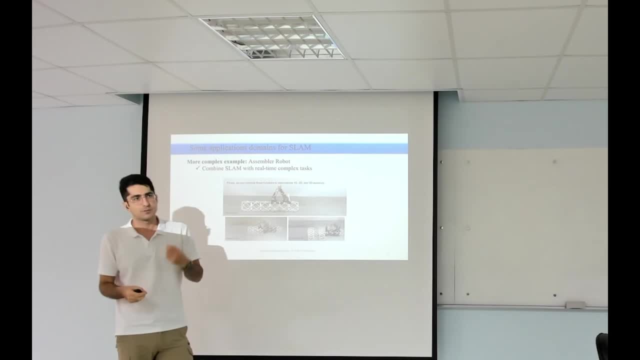 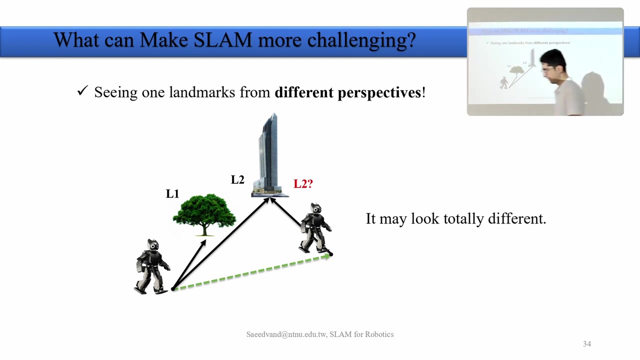 water, for example, Or micro robots in human body, Or you can imagine many applications that also robot uses and other objects. but Islam is also applicable there And it's real time complex, So this task can be used. OK, Let's talk about the more challenging parts of the Islam now. 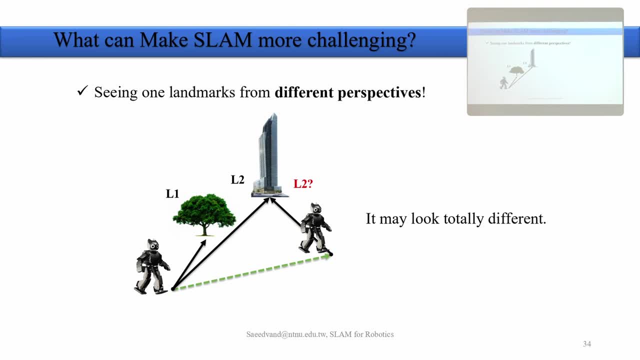 I gave you a little bit of introduction what is happening, but let's see in more details. We have the robot. This robot sees landmark one. two, then robot moves in the environment And sees this one First question that I explain is OK, is it L2 or not? 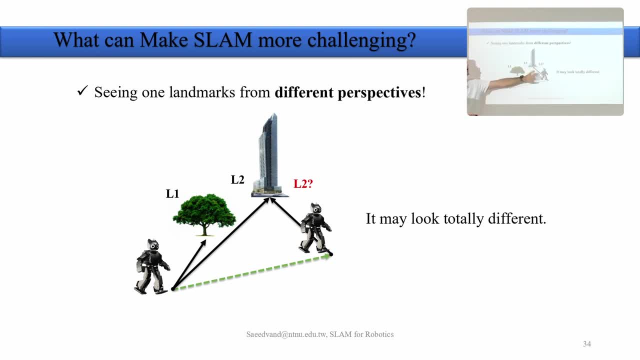 From this different perspective sees and maybe looks like a little bit different. not exactly the same. Is it the same landmark or not? Who knows how we can solve this If the landmark is a QR code on the wall? no, definitely, If it's QR code, yeah, that's very simple. 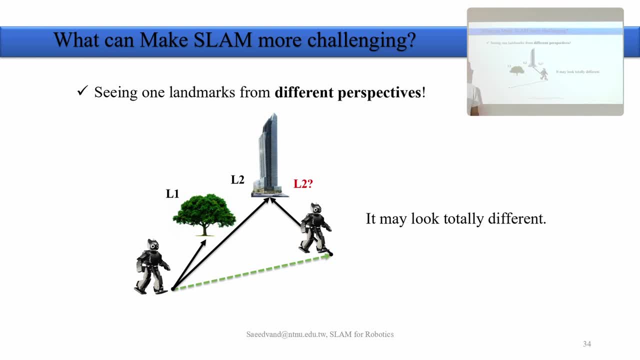 Or just mark the landmark. If you can mark, yeah, that's OK. But let's say we want to have real application right, And robot is moving here. Then you cannot put mark on everything that my robot wants to look like. 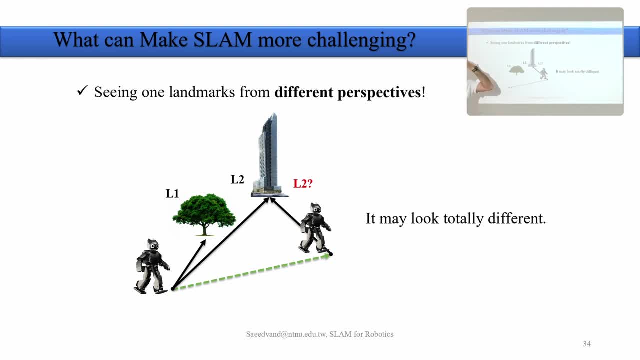 And what if I'm walking there too? You want to put mark on me? Any idea? OK, Yeah, that's a solution that can be, But the answer is like: in order to be able to do this, we have different courses. 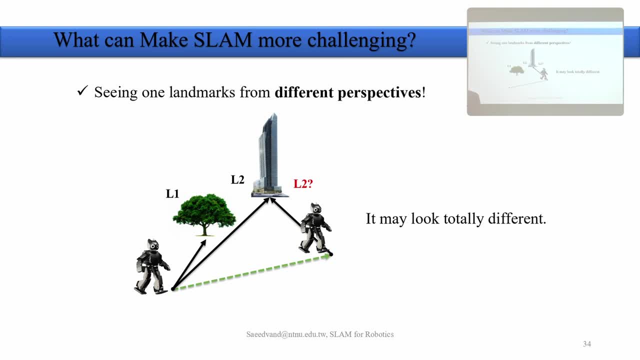 We have two courses. We have computer vision, We have neural network, We have deep learning algorithms, We have machine vision. All these different courses, all these different algorithms, based on what kind of problem that we can have, are applicable on this problem. 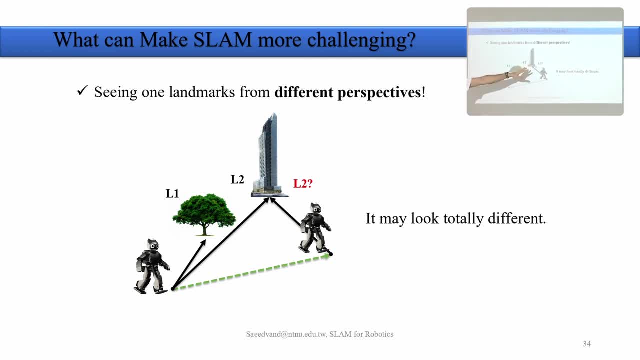 And still this problem haven't solved completely yet. We have algorithms like 90% accurate, 80% accurate, 99, 95% accurate, but it is not solved completely yet. We will see. We will see in this course. 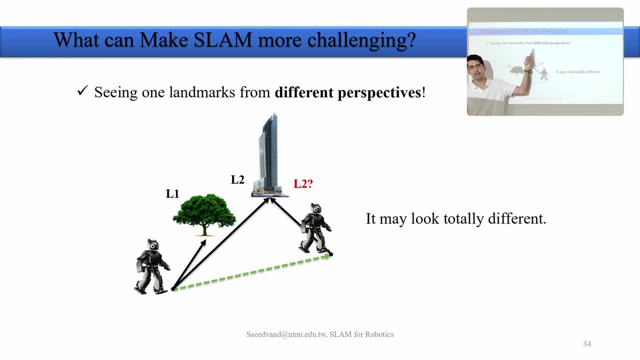 OK, If you have this problem, how we can guess it, Not just only based on visual information. Now you should like spark in your mind, OK, So how we can do that. Now if I'm, my robot, is here and move like one kilometer or move 10 centimeters, 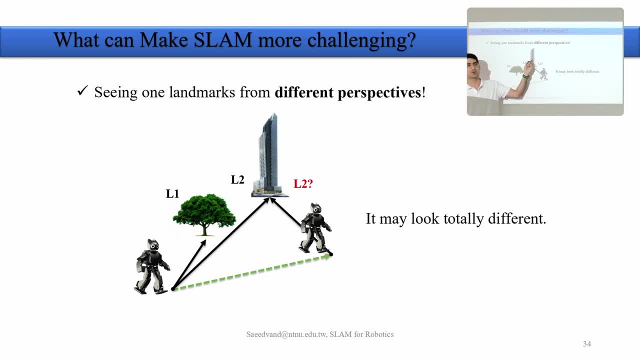 Can that landmark like fly if I move a little bit or if I move a lot, that can be changed. So you can think that, OK, I can kind of imagine robot kind of can imagine where it is, can kind of estimate where it is. 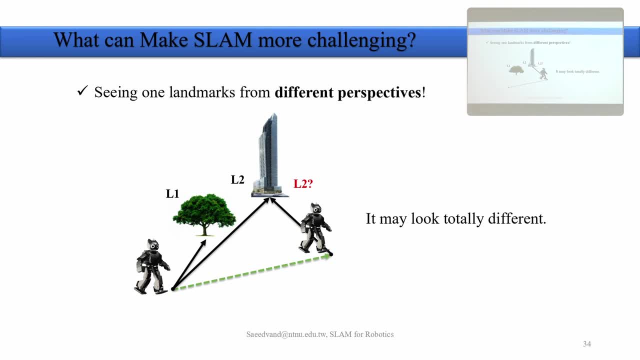 And we will use it a lot. So to help the vision part, to help visual part. What about other problem that we have? Robot was here, moves here. This time, instead of this L2, see this one, L1.. Is this L1 the same one that we've seen or this is L2, 3?? 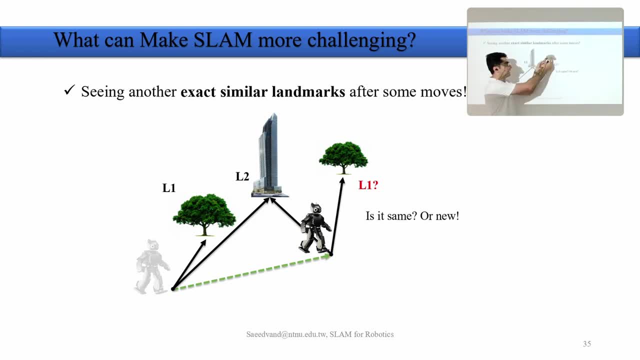 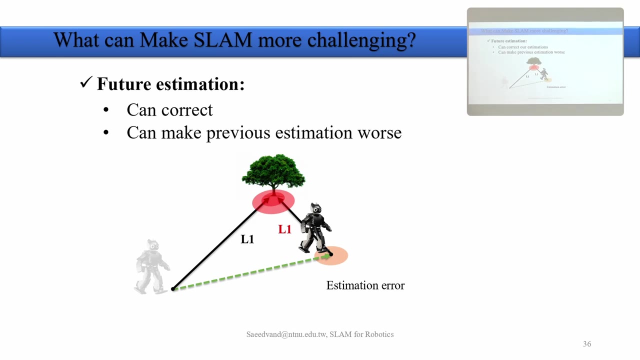 Because trees are all similar. Is it same as this one or this is new one? A question that in SLAM we will try to answer. Then we have, OK, two items that we need to say. Future estimations can correct our estimation or can make our estimation worse. 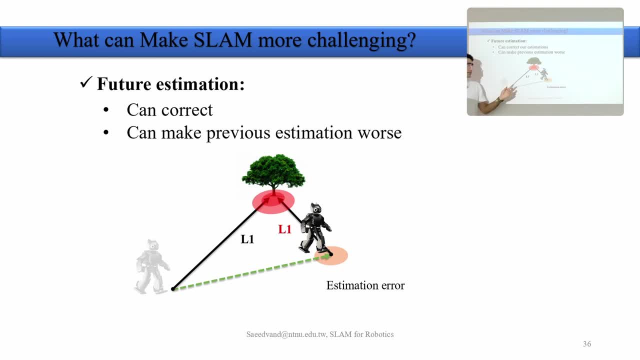 What does it mean? Robot was here, moves here. This one here shows the error. We call it. you will see, we call it Gaussian error, Gaussian estimation error of very robot. This is kind of a circle that we say: OK, robot, if we move from here to there, robot. 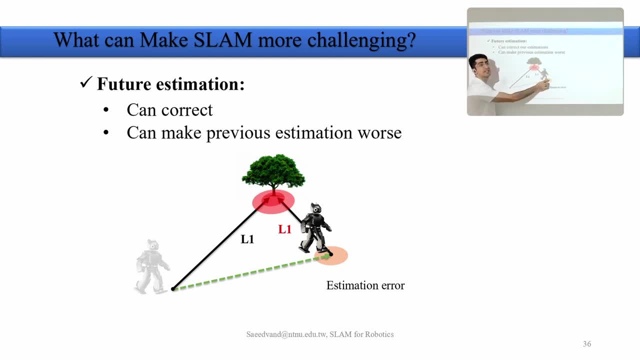 can be somewhere around this circle based on amount of error that we have. If our robot has lots of error, based on the all the items that I counted, you can be very big circle if we have a lot of error. But if it's a small error it can be the estimation error, like this: 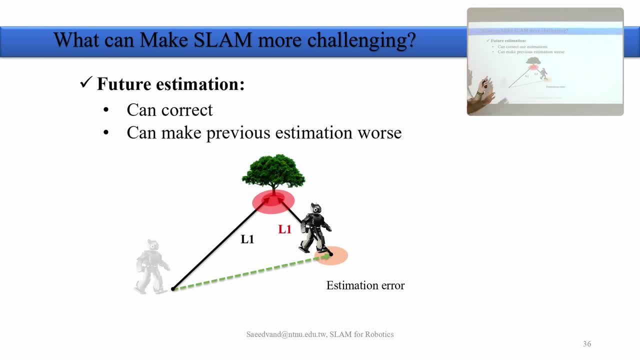 And even if, like you don't know where the robot is, like everything is like 100% error. what happens there? We have a big circle, A big circle around all this robot. Maybe we wanted to go there. Robot is end up here. 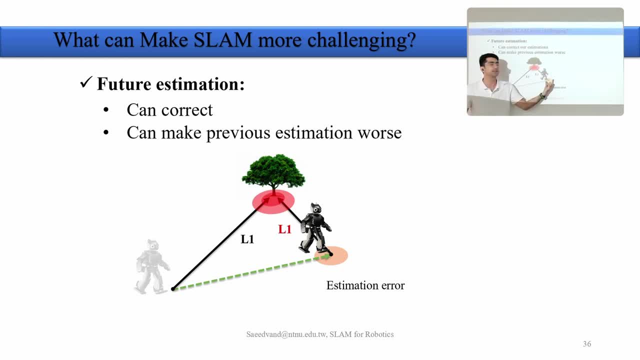 So that circle, that is Gaussian error, we will formalize it. We try to formalize and solve it. This is robot error, It's the location error. And also we have the error of estimation of the where the landmarks are. That again we can show them in Gaussian model. 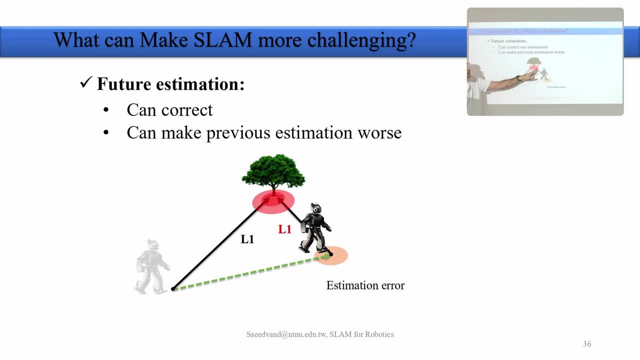 So this circle, like imagine the big circle, The big circle is showing: okay, my vision, robot vision, can detect the object over there, for example. Then, but we have error. We can say, okay, it's somewhere around there inside the circle. 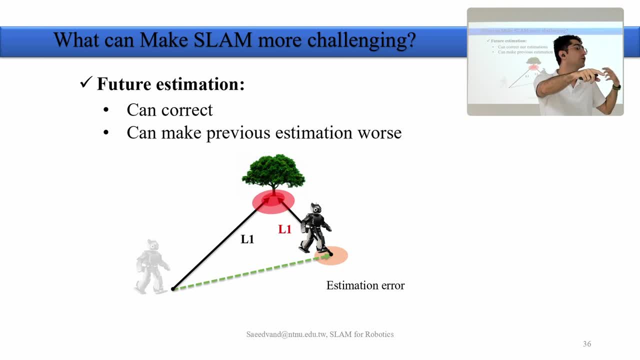 Based on error that I have. I know I know my camera has 20 centimeters error And I can put a circle that say it should be somewhere around there. It should be somewhere around there. This is that one And we say okay if robot in next move goes there and can estimate this more accurately. 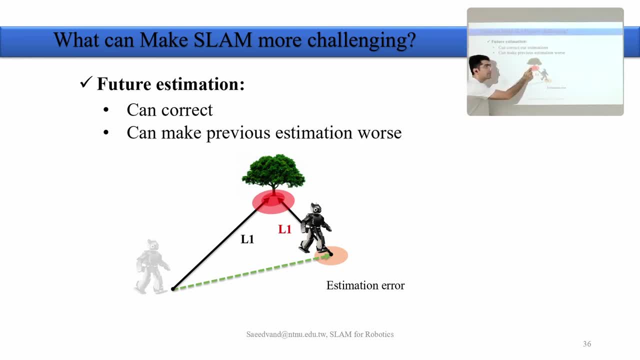 the circle can be shrink smaller And, based on this smaller one, we can correct all our estimations. Or, if it gets worse, it can ruin everything. Based on this change during time, this can change our localization and mapping. You may think: oh, what does it mean? during time, it can change. 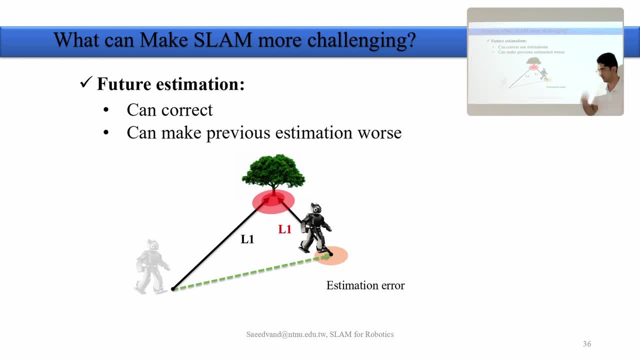 Any idea. We will see No worries. Of course, that's also important. We will see that, yeah, our robot is moving During time. my estimation, these circles can be changed And our objective- one of our objective- is try to make it smaller. 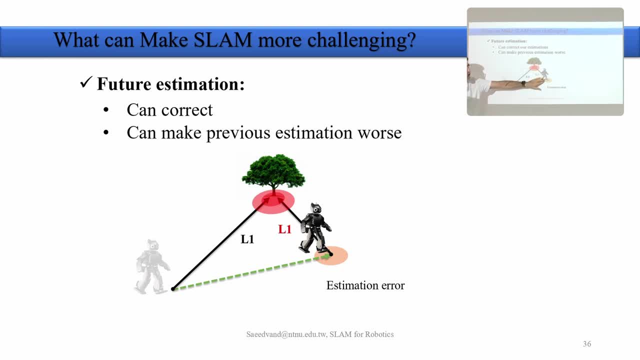 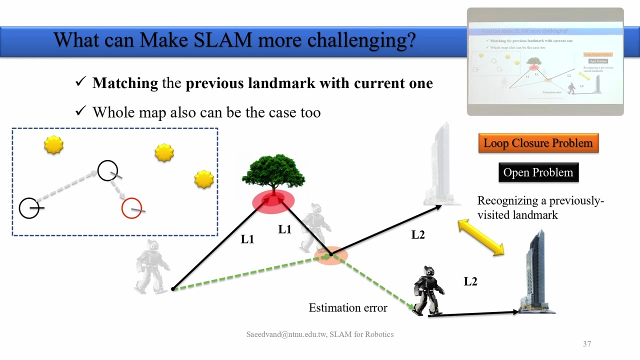 Either for the objects that we detect and for the robot that we detect. We have static error for sensor, But we want to try to estimate to make it smaller. One of the other very important challenge that we have is loop closure problem. Loop closure problem is very famous in the world. 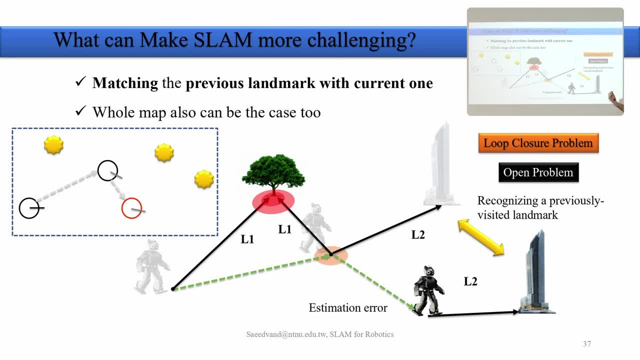 And in Islam it's playing critical rule. What does it mean? It means that robot is moving and seeing some landmarks And moving again seeing some landmarks. If this landmark is the same landmark that robot already seen, we must detect it in order to save. 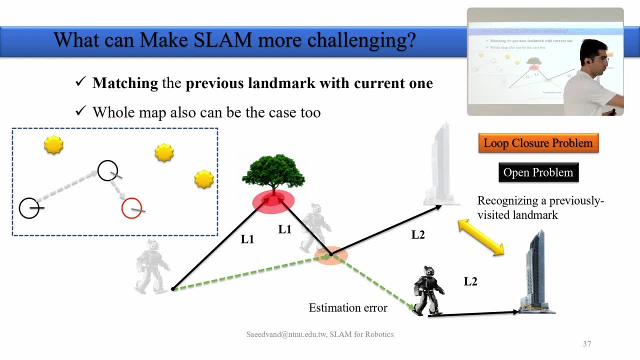 I was starting from here. as robot moved in the class moved, moved, moved, moved- came back somewhere around here And the same landmark that I'm seeing is very important and it is called loop closure problem because I can close my loop. 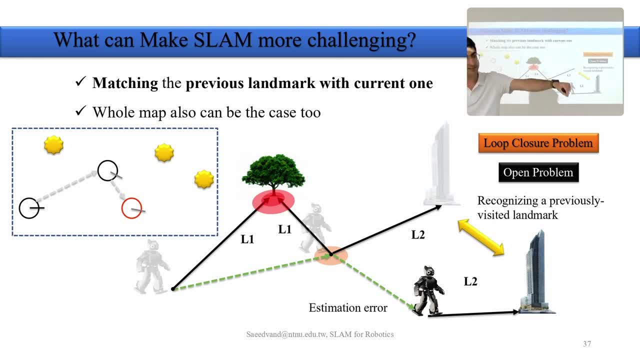 And based on this estimation that at the beginning I've seen that and after a while of coming and seeing again, I can correct all my estimations, all the circles that I showed, all the Gaussian errors that I showed. I can correct all of those estimations during time. 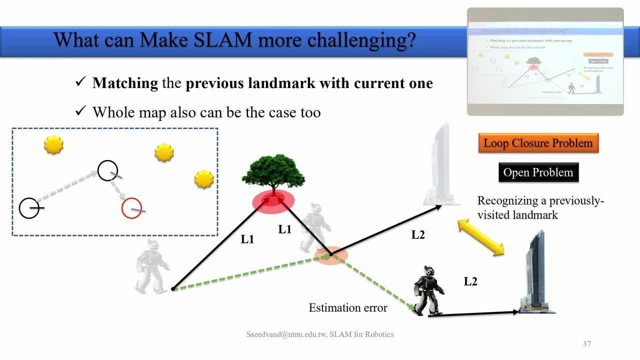 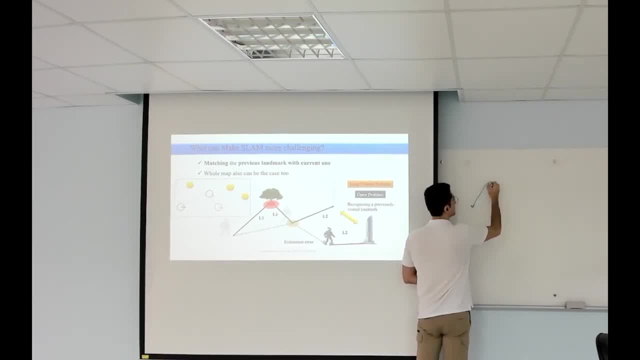 It's like this. We will see, of course, many examples. I think I don't have it there. Okay, So, robot sees the subject and moves, But my estimation, this is the real path. But my estimation, the algorithm that we have can be like estimate, like a little bit of error at the beginning of the motion vision, or whatever it is. 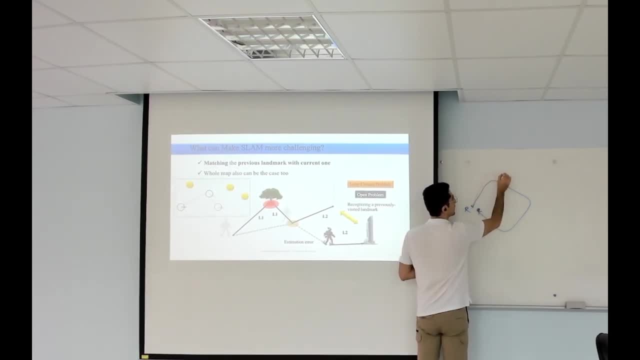 Then rotating, Then like this, maybe, Then maybe like this. This is very common problem in algorithm, that we will develop, even the advanced one. But this is very important as loop closure, because if you know that this is this one, then you can know what to do almost. 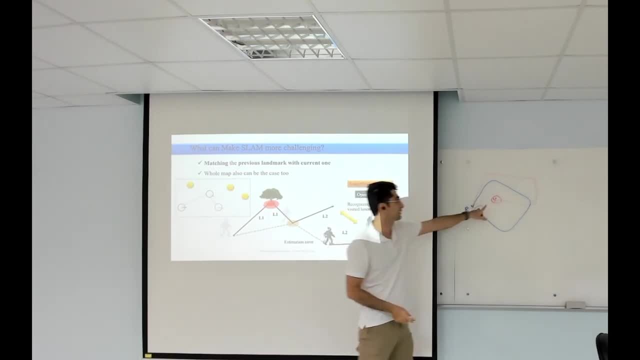 We will see with math how we can do that, how we can solve this, How we can. if we see this over here, that was there how we can deal with it. That is called loop closure problem. It's still open problem. 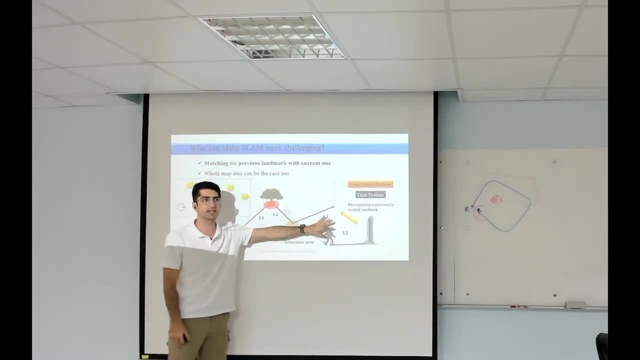 You can publish papers on this, study on it. proposed learning algorithm, deep learning algorithm, reinforcement learning algorithm. Whatever you know, you can engage here to solve it and make it better, Just in this slide, And we will, of course, since the problem is a little bit complex. 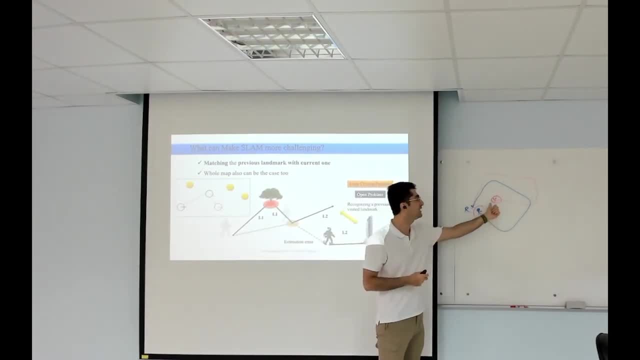 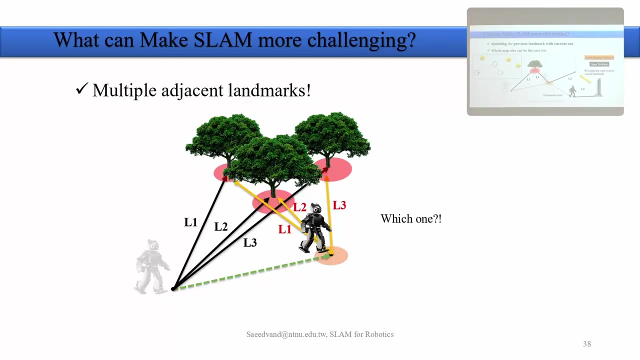 At the beginning. consider that we can detect it, No problem, We don't need to solve it. We imagine: okay, if you see that the object landmark one that we already seen, we know it, We can just match it. But later I will introduce some techniques to also deal with that problem. 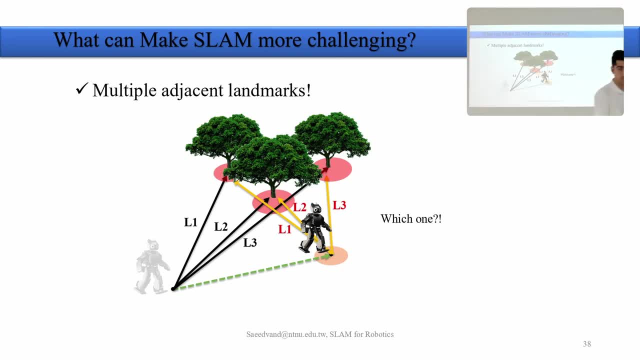 What else has challenge? The challenge of seeing multiple adjacent landmarks. That is very common in real environment. Robot from here sees three objects together that they are adjacent in hidden back side of each other. Moves a little bit and sees them from other perspective. 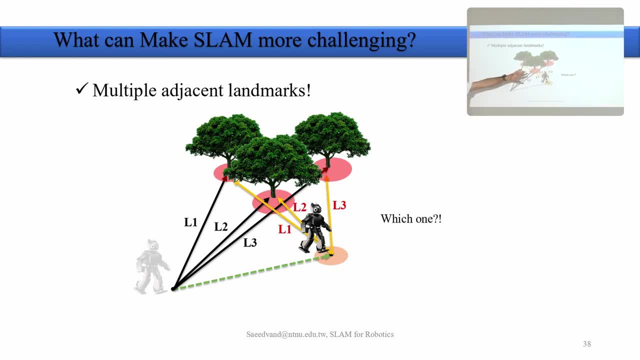 Then we say, okay, which one was which one, and should we consider whole as one landmark or each separately? This is whole Also computer vision, machine vision, challenge that we have, and it is existing in Islam too, I think, two, three minutes. 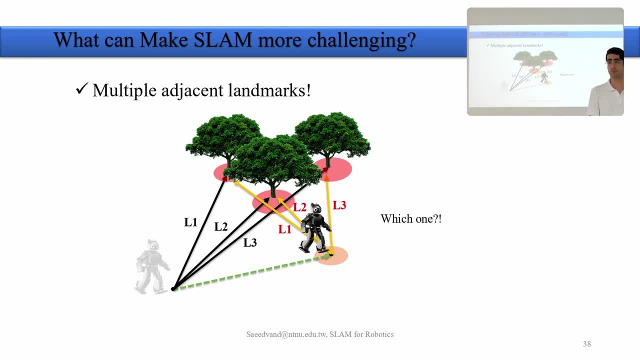 So let's continue. So we were talking about the challenge of Islam and we saw, okay, what kind of problems that we may have. We talked about the multi-adjacent problem, that when you see multiple landmarks in the environment, how to detect which one is which one. 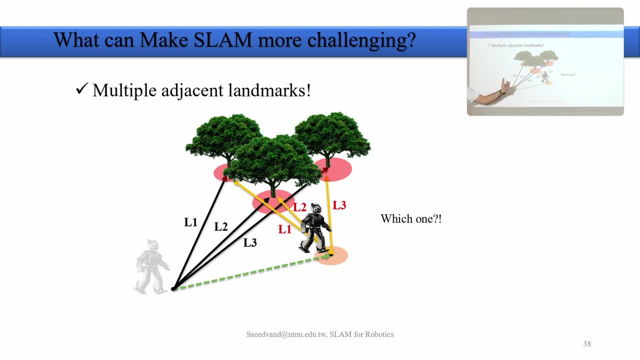 In computer vision. I will introduce some that you can see. okay, instead of talking about the landmarks individually, we can extract some features. Go to our features of the environment and try to extract features and talk about everything based on the features of this information, not just exactly, precisely, the landmark itself. 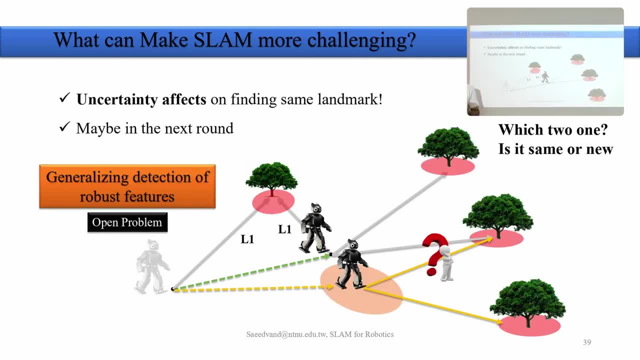 Later we will see that's kind of clue for solution to how to deal with those. but sometimes still you need to detect it separately. We have uncertainty effect of the. another problem is uncertainty effect of the finding landmark. So this uncertainty effect is can be troublesome. 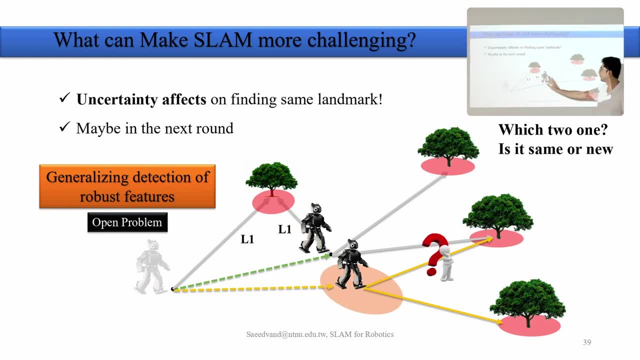 Robot is here, sees some landmarks, moves to point two and sees these three landmarks And, as we saw we discussed together, there can be some estimation error of the object location, like these three And what, what that can happen, what problem that can happen is here: 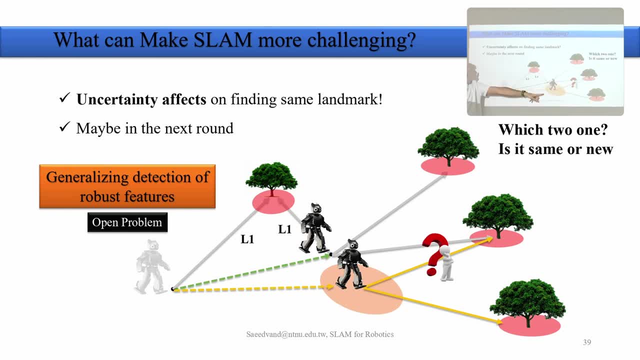 Next time, like previous, like this, this is one time. Next time, robot moves and comes here. Now the question is: from robot side, if robot sees two of these, based on this error, that we have even based on that error. 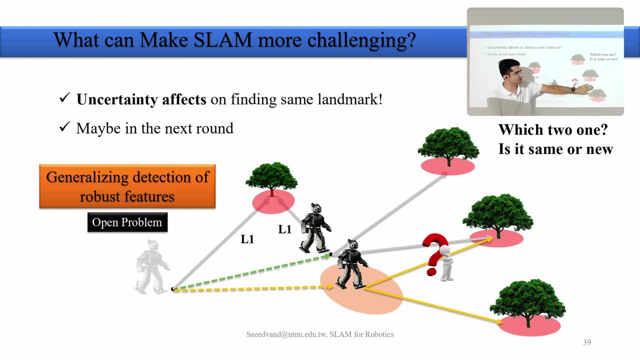 robot needs to answer: was that these two objects or these two objects, These two landmarks or features? doesn't matter. Were these two or were these two? Again, I'm coming from here. robot comes there, sees two, these two even can see these three, doesn't matter. 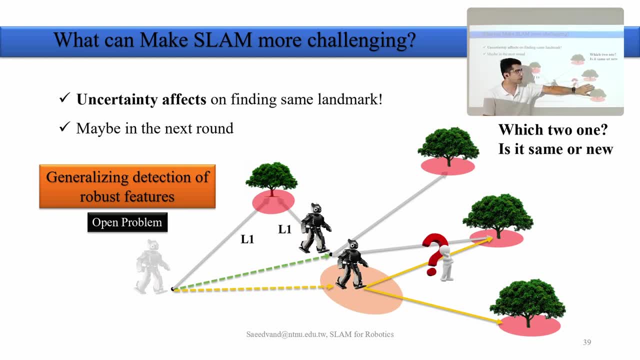 So when robot comes here needs to say: okay, it was these two or these two And why this is happening? Because these Gaussian model and the error that we have Is it clear For everybody. So of course we want to generalize the detection of the robot features. 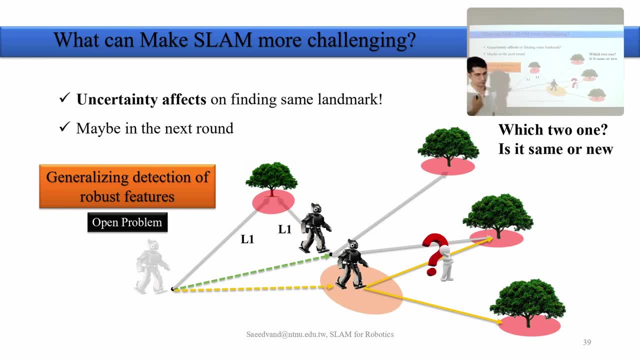 And it's still also- this is open problem- to find very accurate and nice features of the environment that is robust and works every time. Also, you know we have the challenge of the environment, light change, the dynamicity and many parameters that we want to also. 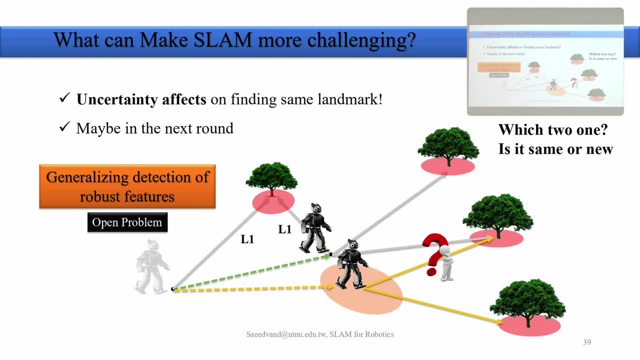 we prefer to have it And this is also open problem. So whenever I say open problem, that's a field that you can go: research, Study for your master or even PhD, And even for companies. These are challenging companies, big, big companies like. 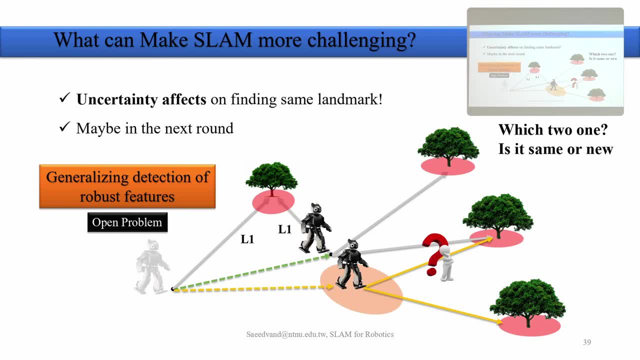 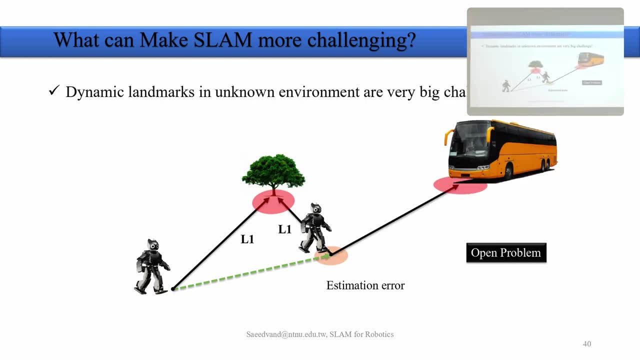 can be Amazon, can be Google, can be whoever is working. related or related topics. Of course, we have the challenge of dynamicity. As I explained, robot is moving, Detects this landmark or detects these features over here. Next time comes, it's not there. 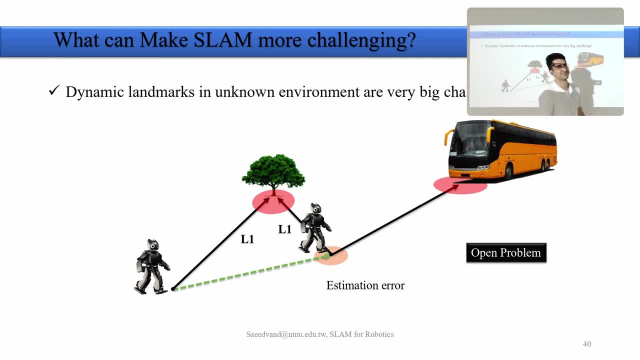 What to do. You need to solve it. Give some ideas what to do If robot is, was there, come here and working 10 times, But this one time this bus is gone. We need to construct same map we had. 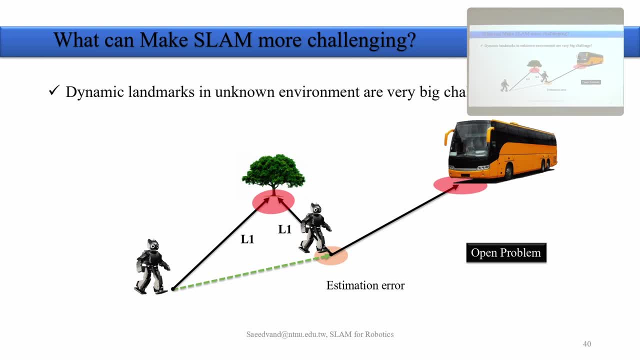 We need to localize the robot that we had. Then, of course, that's also open problem, Not completely solved yet. There are techniques. There are techniques that says: okay, try to not use just one landmark, Try to use more features. 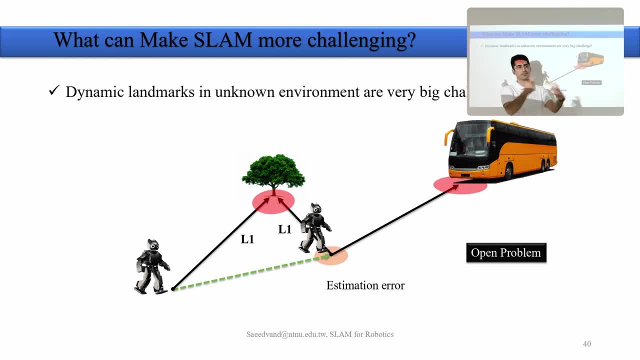 And build your algorithm somehow that, if the elements are changing inside, you're not relying on just one and you can estimate all. But that's not easy. Like, let's say, my robot is seeing three dynamic objects and three static objects. How can I distinguish? 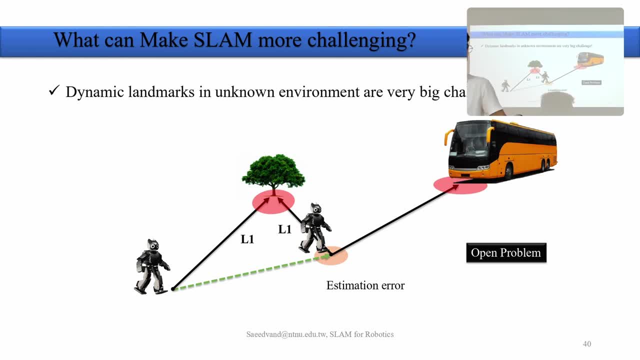 That's not human that knows that this car may go. Robot doesn't know. Robot sees this is something over there And next time it is not there. So that's why also that's challenging. If robot understand, it is mobile, it is dynamic. that can be helpful. 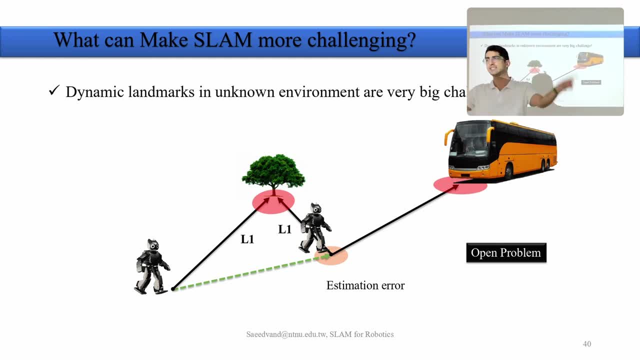 Then we can put some weights on the like. if I see six objects, three of them are dynamic- I can say: the static ones are important for me as robot. Then I have more weight to our math calculations and estimations. So- and this is again open problem- because of that, 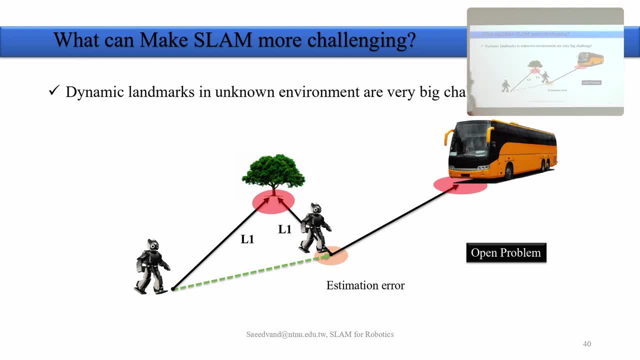 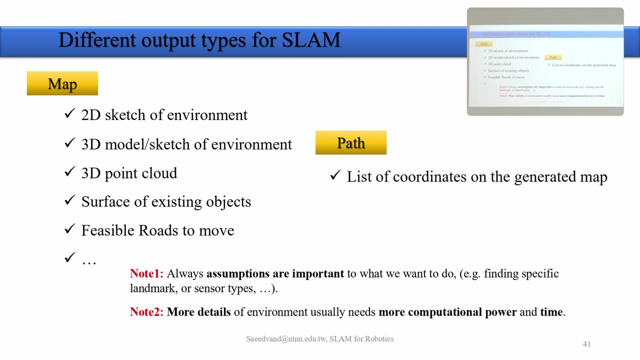 If you can solve it, if you can propose algorithm that is robust. here you can change many things in the algorithms that existing and improve them a lot, And it's still one of the world biggest challenges. Okay, Now let's a little bit talk about the other related topics of the course that we have. 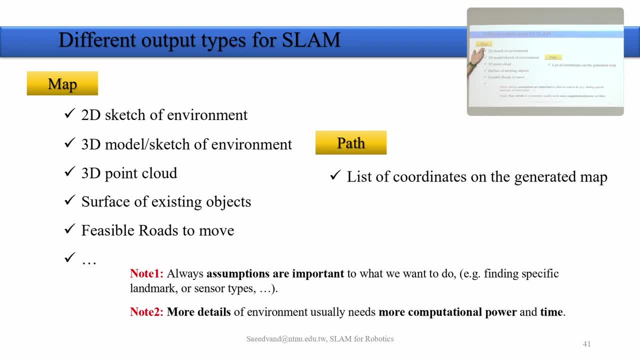 We have the map That this map can be 2D sketch of the environment, can be 3D model or each sketch of the environment can be 3D point cloud. So this is different with 3D model or 3D point cloud. 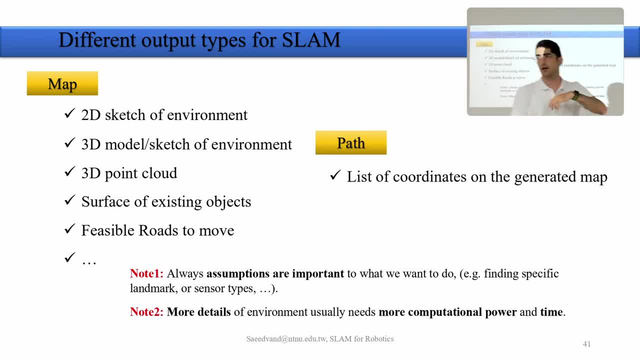 3D point cloud can be like everything that you can see in the environment. robot can scan and can in 3D environment. we can put each one of the things that you can see as distance can put a point over there in 3D space. 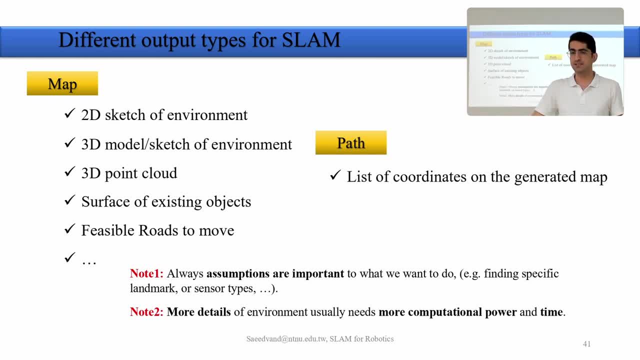 And you can imagine all of whatever see. the ulterior surface of each object will be as a point in 3D point cloud, So that you can imagine in 3D environment you have the same environment. So this is basic of the basics of the 3D modeling. 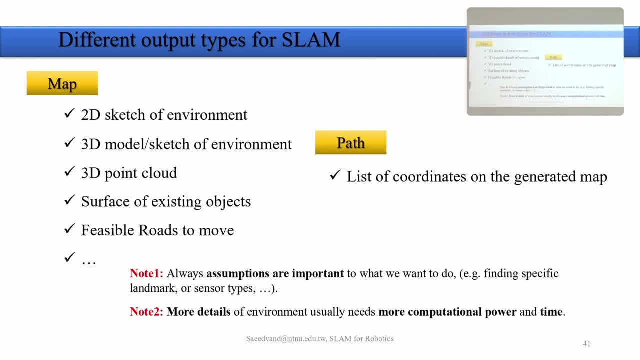 the animations and, of course, the construction, the map and the output of the LiDAR scanner. Some of you guys, I know, have it in the lab laboratory. after you scan it we can construct 3D map of the environment. We can have just only surface of the existing objects. 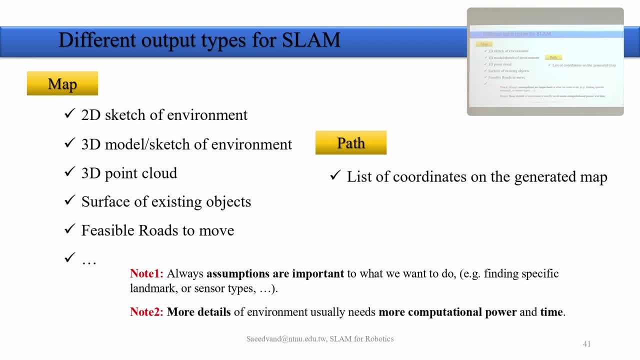 or we can have some techniques to also give the mass of the object and what is the object also not just only surface like 3D or surface, And we have feasible roads to move in the map that also can be included as a part of map. 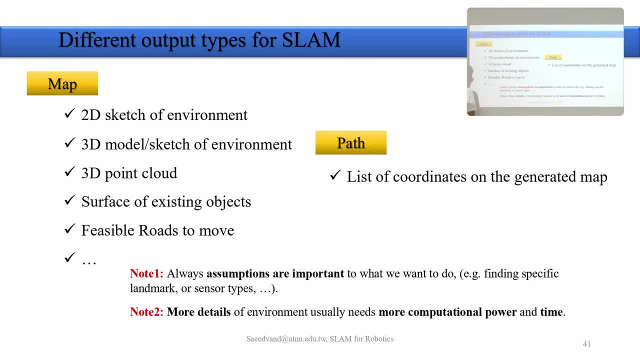 I know, maybe it becomes a little bit complex this part to understand it. but let's say, your robot constructing a map only based on feasible roads, That can be my object. I don't care is it chair or whatever it is, I just care where I can go. 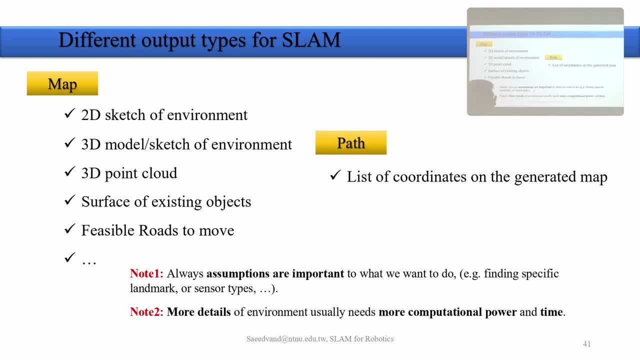 This is very important technique in this lab. Just, we can construct a map based on where is it feasible for my robot to go? That's it. So this is kind of map that we have. In next slide we will see visual some examples. 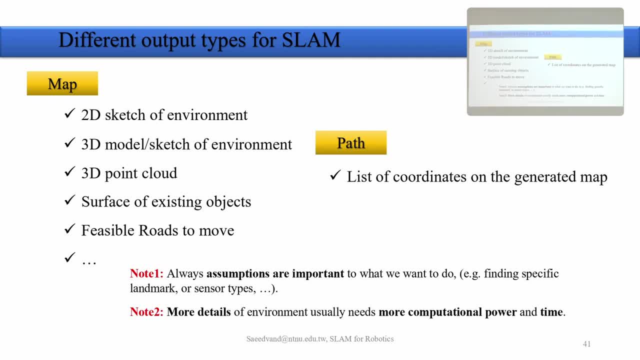 different class of the maps that we can have And the path is list of coordinates that generated based on that map. So when I'm referring to the path I mean usually that the coordinates, the points that robot can move on the map that we construct in this lab. 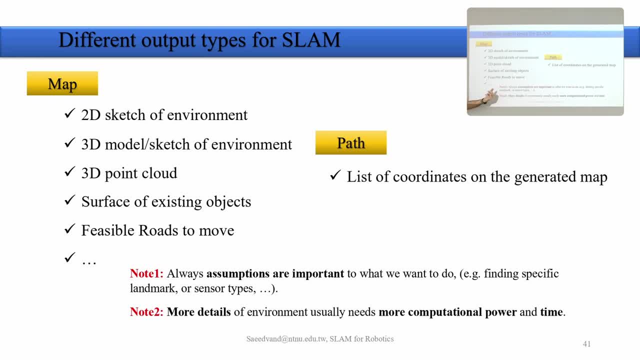 We have some notes. let's see what we have. Always, assumptions are important to what we want to do. You see, based on the sensors landmarks what we want to do And more details of the environment usually needs more computational power too. 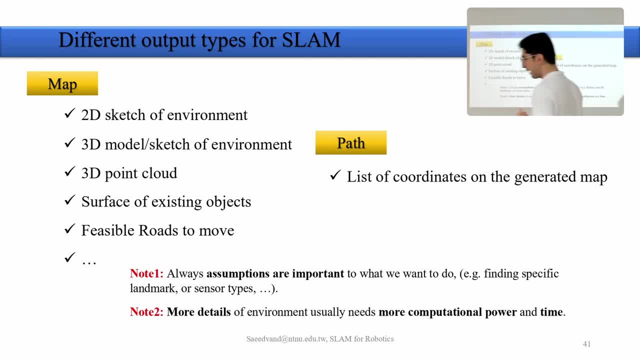 It means that I can have a map, construct a map based on the tiles that you can see, just step by step tiles. It's much more simpler than the map is constructing 3D point cloud of the same room. So constructing those two maps. 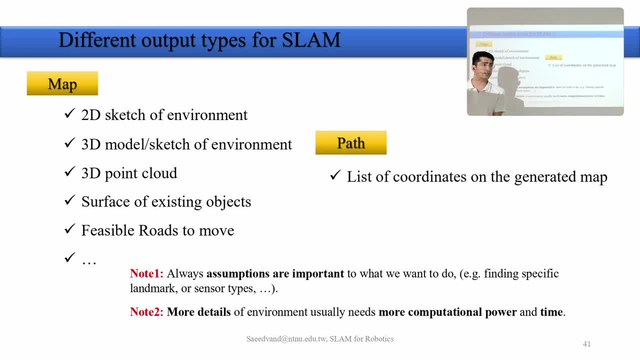 are totally different techniques and, depending on what I'm going to do, can be very applicable. So think about it. 3D point cloud differences with having just the 2D tiles of this environment. Think about the sensors that we can have to detect it. 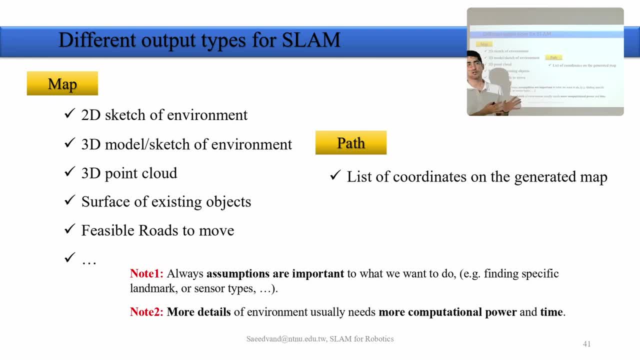 think about the techniques that we can use, the computational complexity. what does it mean? It means that you're writing some code, some for loops, to understand what's the path. And if you have 3D point cloud, it means that for each point, 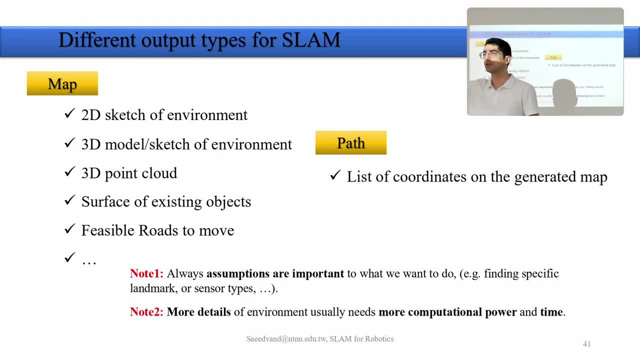 you have a pixel on 3D environment and you have millions of those in just here, Then how you can understand what is the path in between those? No one tells you where is the applicable path. You need to write some code to detect it. 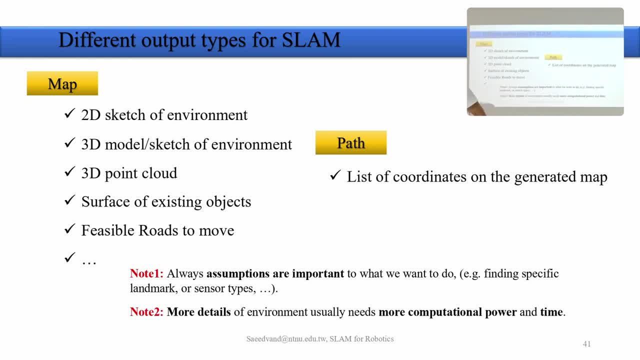 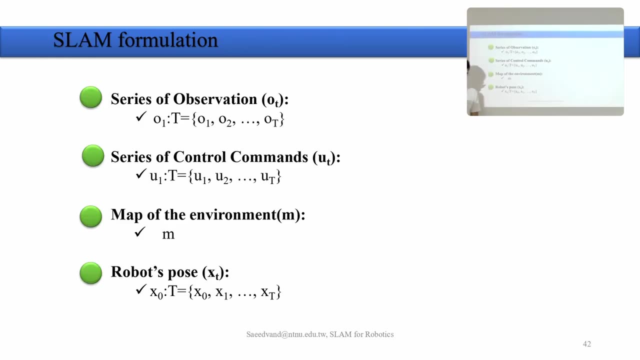 And you have point cloud and even you don't understand the differences of the floor and the ceiling. They are just points on the space plus a lot of error. So that's the note that also we will see. Of course we gradually need to formulate everything. 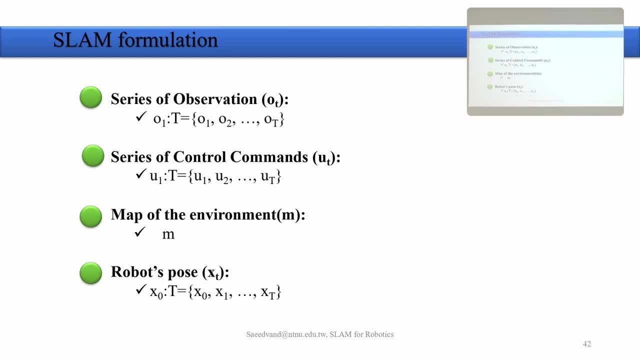 not just talk. We need to bring it to math and the calculations and computer system codes, even Algorithmic algorithm form. So there are starting point that these are the math that you need to know, The basics that we will always refer to, talk about to. 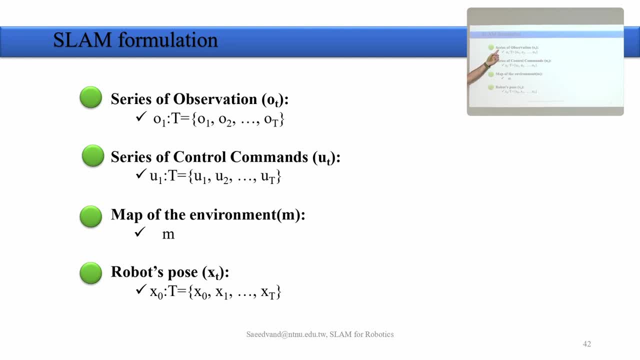 First of all, we have series of observation. Series of observation includes observations over time, Observation over time That this observation is a list of the observations, Observation 1,, 2 up to time t. It means that my robot is moving in the environment. 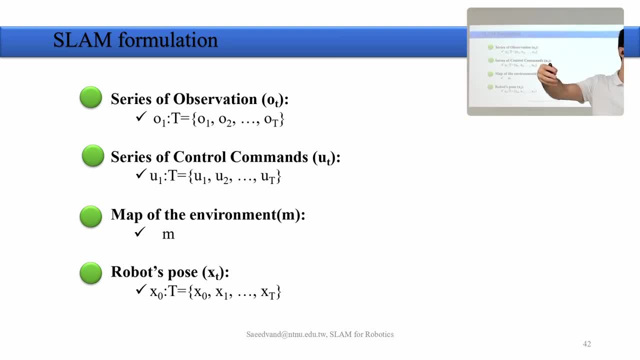 and I have. my robot has each time different observation of the environment and I'm representing it as observations. So you may think: okay, observation at each second, at each minute, at each hour doesn't matter, Depends on us, Depends on what we are going to do. 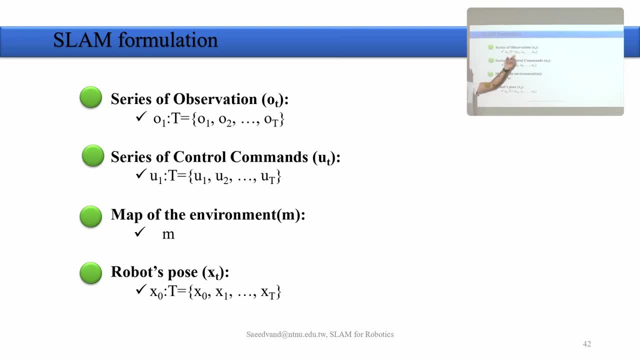 We are assuming observation for now. Plus, you may think what kind of sensor Doesn't matter, Whatever it is, Just whatever robot can get. We generalize the problem now. Observation Series of control commands. We show it with u, u1 to t. 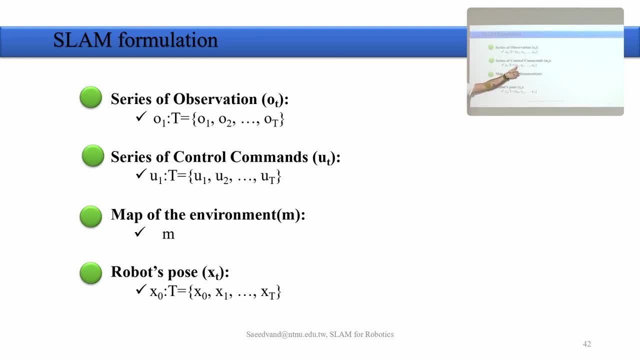 and control commands are kind of like: okay At the state 1, robot is here, I send control command move forward. How much doesn't matter. for now We have general problem: Robot moves, That control command is u1 and the observation that we see there is u1. 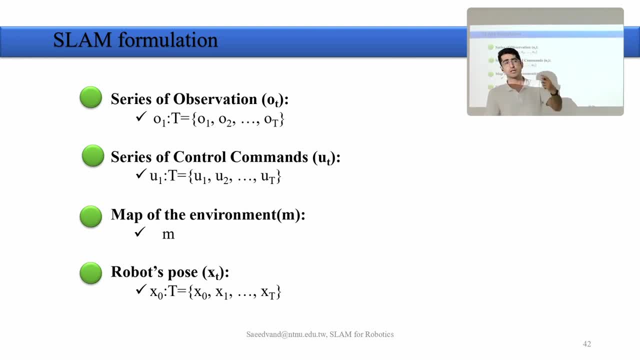 Usually we don't have u0. We can have. this is in formulation of: if you study books later you will see Basically at the beginning we don't consider it, although we can have it. Observation can be at the state 0, 2.. 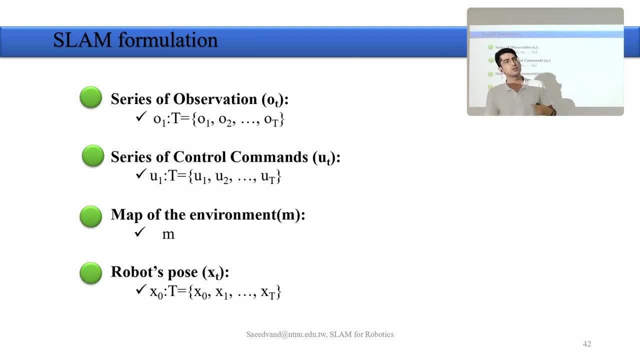 Because without motion command we have the observation 2. But usually we formalize it like this in books in all calculations: So from state 0, control command, observation, Control, command, observation, Control, command, observation Here. 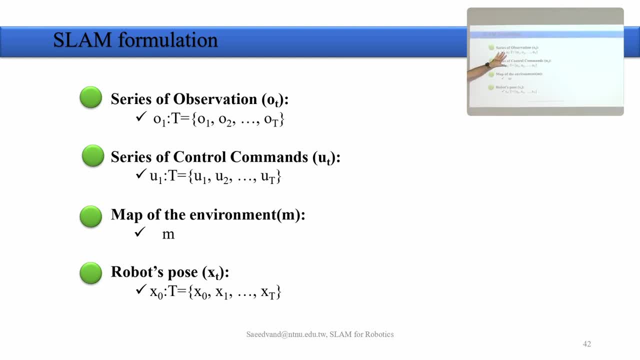 These two And any question. Okay, So then we have the map of the environment during these procedure that we want to construct it. So we wanna run the control commands, Get the observation and construct the map, plus find the robot's pose. 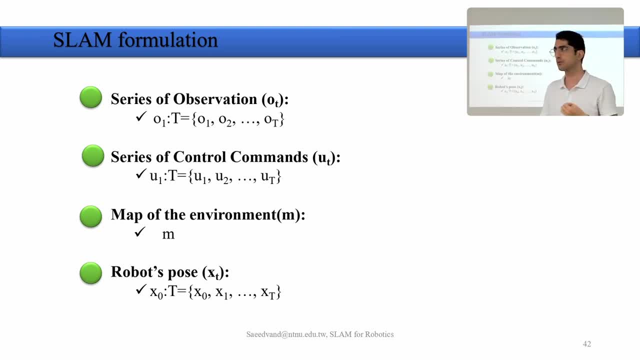 What's the pose? Who knows What? No, It is location, but not the answer: Robot's body. What do you mean? No, Robot pose is important to know. So we have two terms: position and pose. They are different. 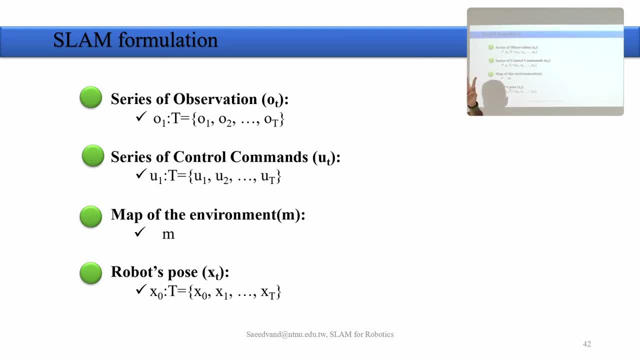 Position means where the robot is in X, Y or even Z if you have 3D environment. Robot pose means not only X Y, Z, but also where the robot is heading to The angle of the robot. 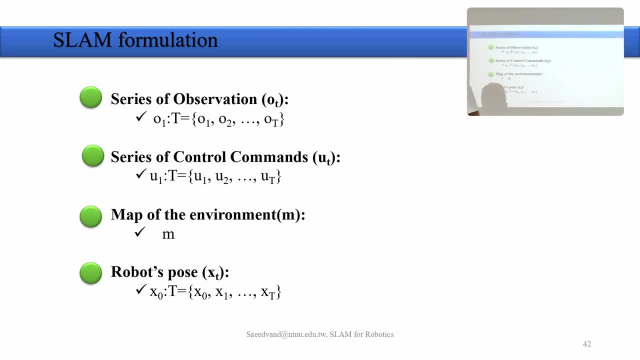 It is important, very important, because then you say, okay, move forward. depends on where is the forward? for me, the environment. If it's like this, it's forward. That's the pose. So what we want to do, 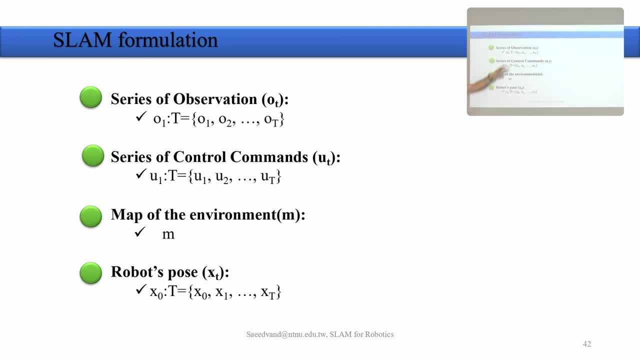 we want to, based on these two, also get the robot pose That we show it as Xs, X0 to T shows the pose of the robot. So each time you're running the command motion commands in your robot, you get observation. 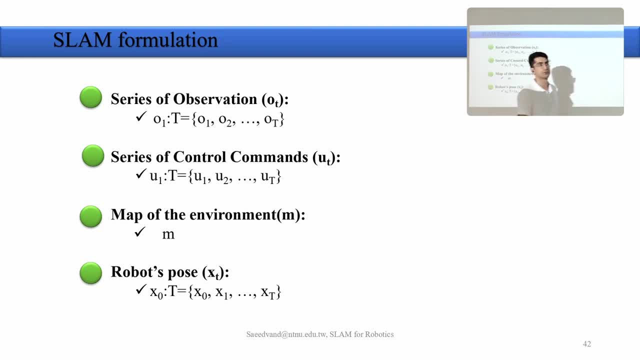 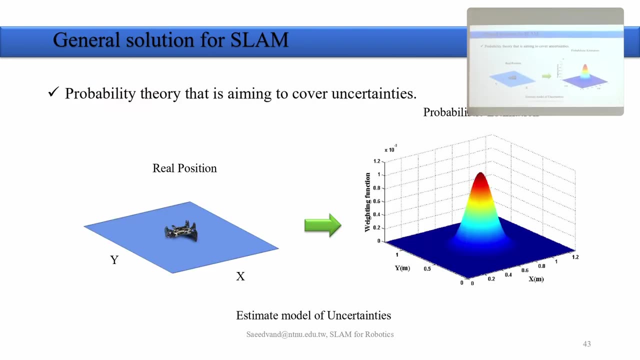 and you wanna construct the map and you wanna find the pose of the robot. So this is whole problem that we are gonna solve in mathematical form And all these will be always using- we will use these in the math stat calculations that we have. 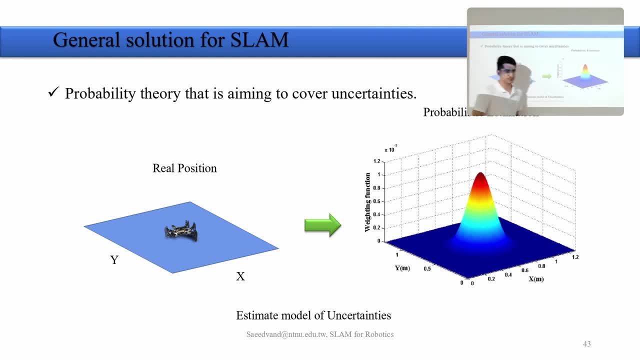 So, as I explained a little bit about the error and the probabilistic error, I said that, okay, you're running motion command and robot moves somewhere in the environment. then you have estimation of the error based on the sensors, from odometry or visual. 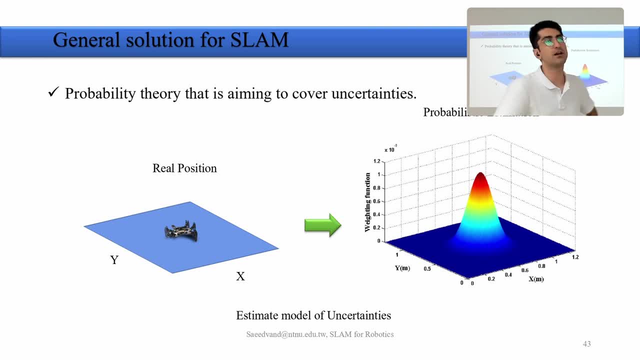 Both of them: That where the robot is, you can put a circle somewhere around there And that can be shown as a probability. And that probability- like if the robot is here in real position- can be shown like this: Why it is like this. 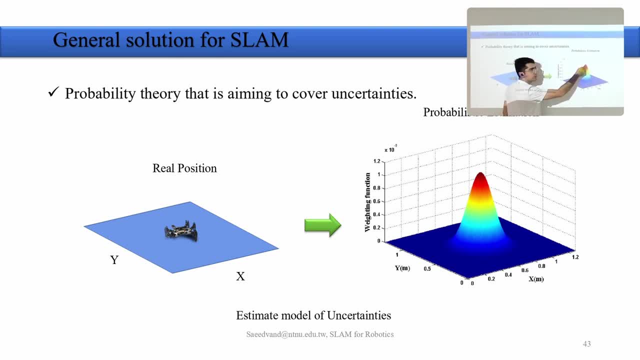 This shows more certainty, Like if the robot is here, more certainty And how it goes to the corners. the certainty is decreasing And of course we wanna. this is like Gaussian model. If you look at 3D Gaussian model. 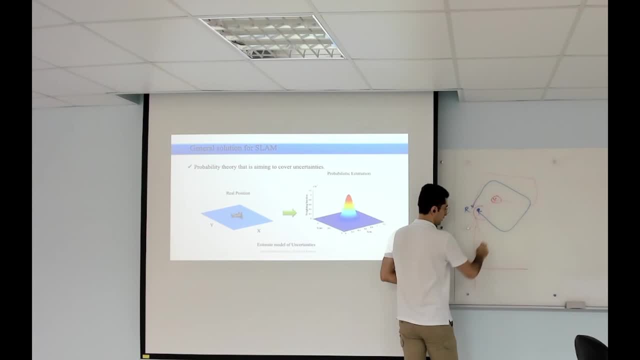 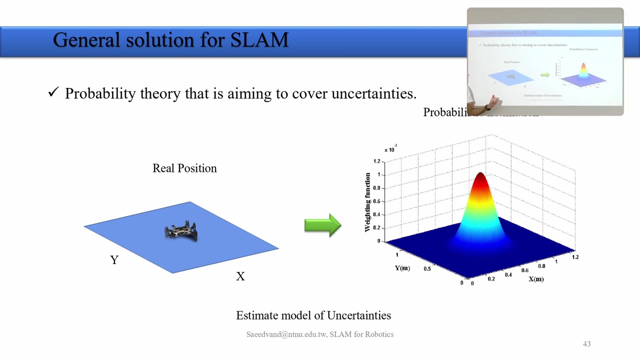 we have the Gaussian model. that shows we can represent where the robot is and how far we go. the probability of the being there is getting lower And how much we are in the center it gets higher. We will also explain it soon in details much more. 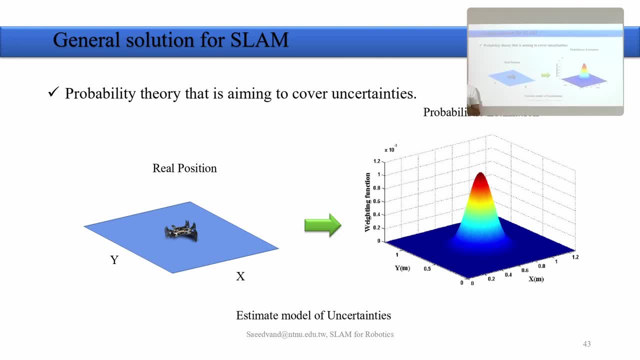 So all the things that we are going to talk, we are trying to the robot pose, estimate the robot pose based on the probability form of the where the robot is, Because let's think a little bit in mass, Like. 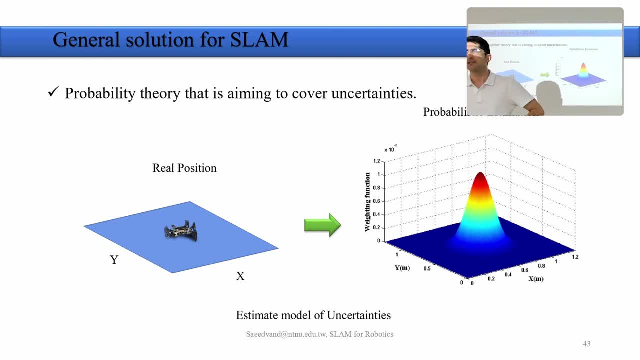 robot is in xy. You wanna estimate where it is? Can you estimate like one exact value? That never can be correct, right? But instead of that exact value estimation you can say it is Gaussian model somewhere around there in probability form. 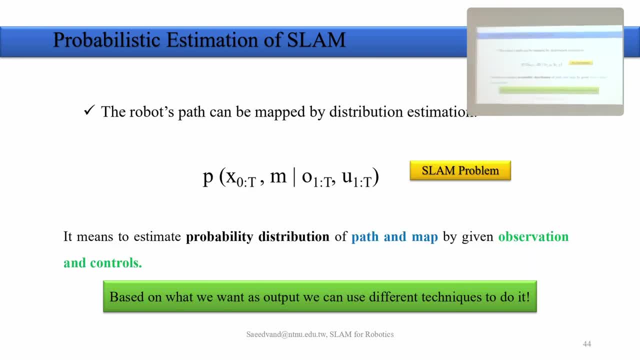 So that this is the thing that we have. So now let's show the SLAM problem in mass. We can say, okay, we saw the formulation and we saw the probability form. Now we want to put it together. We say we have the probability of the. 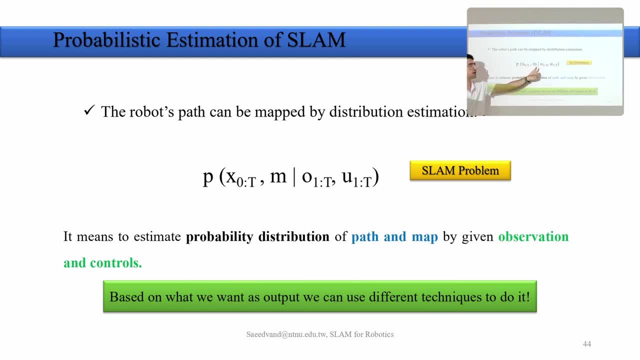 x0 to t and f given by observation and motion commands. So we wanna get the pose And the map given by. we read this line, as given by observation and motion commands, that they are 1 to t and 1 to t. 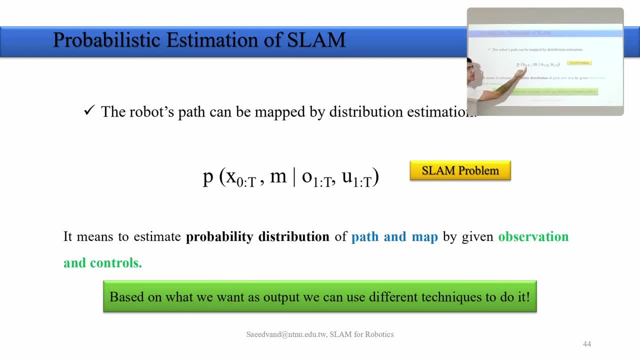 So you can see here the point that I mentioned: x is starting from 0, because the pose of robot starts from 0, but basically in formulation we start from 1,, observation 1 and motion command 1, in order to calculate the problem. 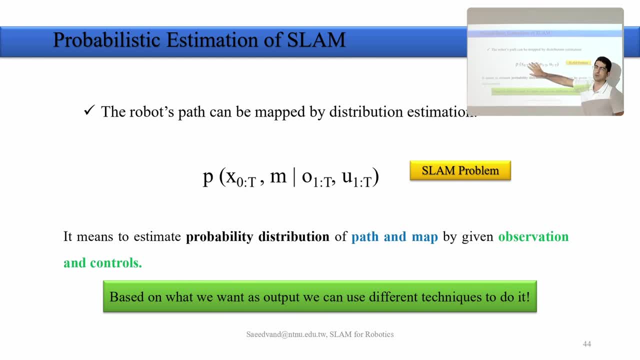 So we want to solve this, All that we are. I've talked so far. we want to solve this and get the probability where the robot is and what's the map. So I've written here for you guys later when you study. 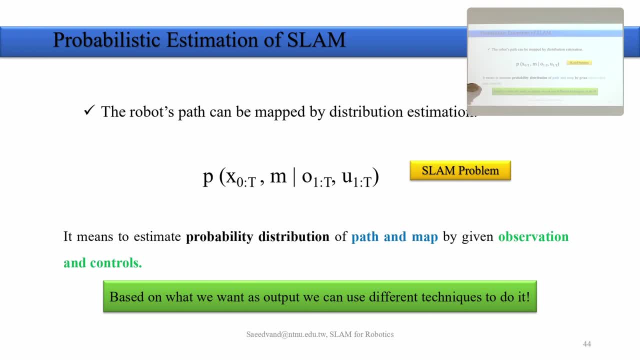 it means the estimation of probability, distribution of the pass and map by given observations. Because, why? why this can be called as pass? Because I told you the many poses we call it as pass, So that if you have all of it, we can call it also the pass of the robot movement. 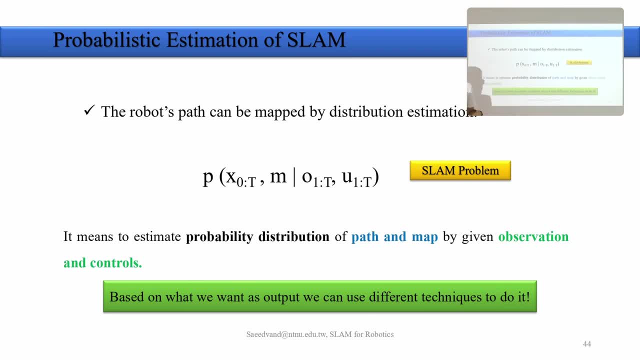 in the environment. So it means that if your robot moves in the map in the in the environment a long while, then we want to estimate where it was and construct the map also meanwhile. So we have we saying based on what we want. 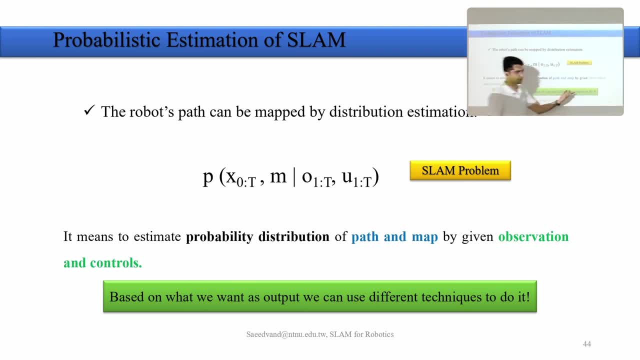 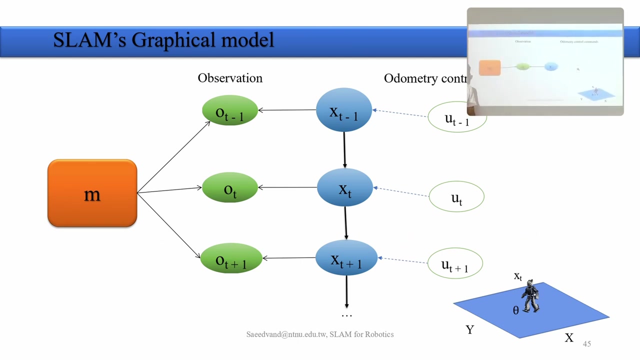 as output. we can define different techniques to solve this problem of the Islam. Any question? Okay, So how we can show it in graphical model? The graphical model of Islam can be visible like this: We have the XT, the current pose of robot. 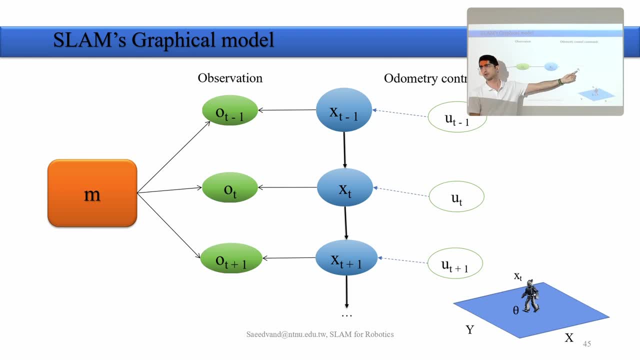 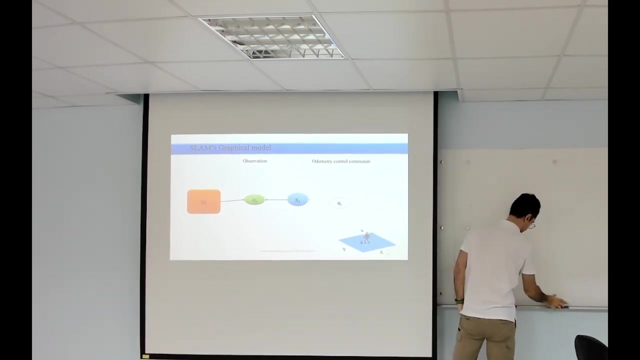 Then we run the motion command. Based on that motion command, we get the observation, and observation can come from. observation can come from both the state of the environment and can come from the map itself too. What does it mean? So this is the map. 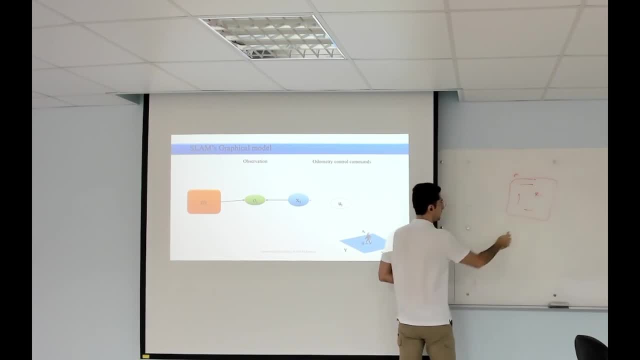 Robot is here and we have some kind of map, And this one is robot and this is real environment, And robot is, for example, somewhere here and there is somewhere there. So the observation not only comes from the real environment, but also can come from. 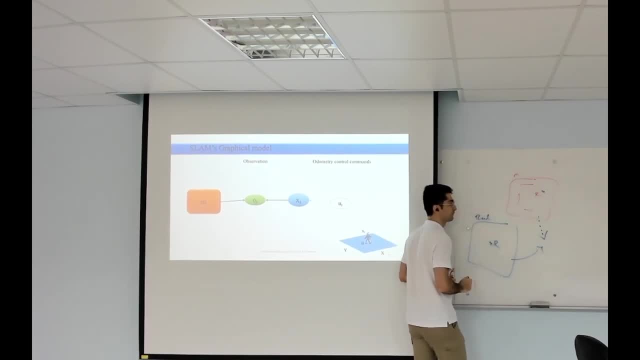 can come from the map itself too, Right? Also, we need to see how to use those two. information that comes from real environment comes from map. how to, how accurate which one it is? when we need to rely on real environment, when we need to rely on the map. 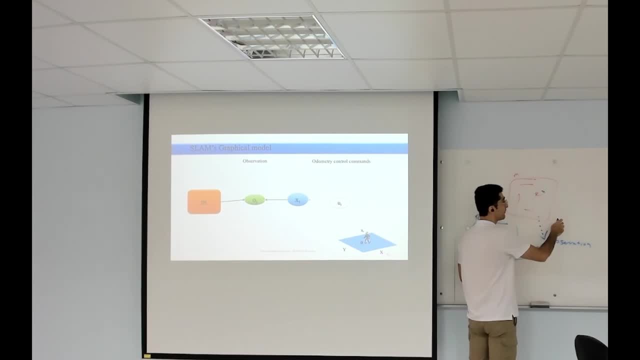 If you want to simply say, okay, this is like, this is OR observation of the map And this is the observation of the real environment, Okay, you can say simply: observation of the map added by, for example, observation of the real environment. 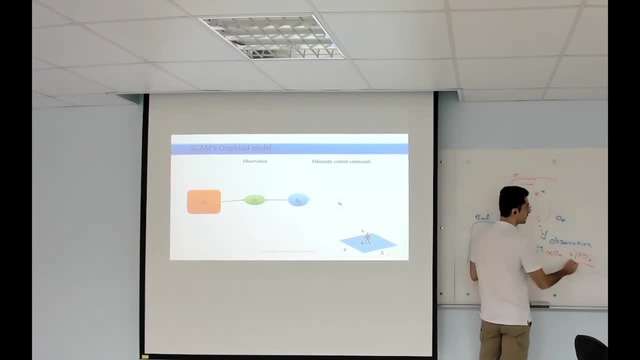 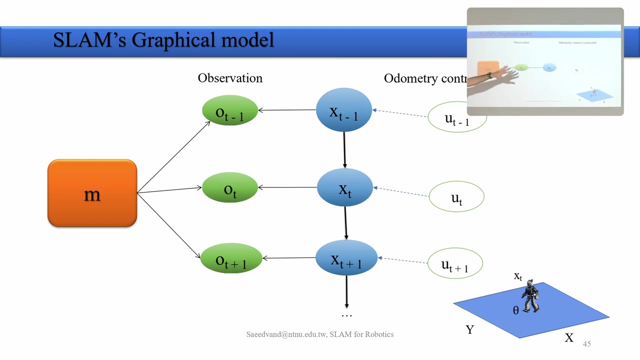 by some weights- Alpha, beta, for example, Which one is more important? give more weight to calculate where it is in simplest understanding form. But of course we cannot do that directly. Later we will see how we can do that. So 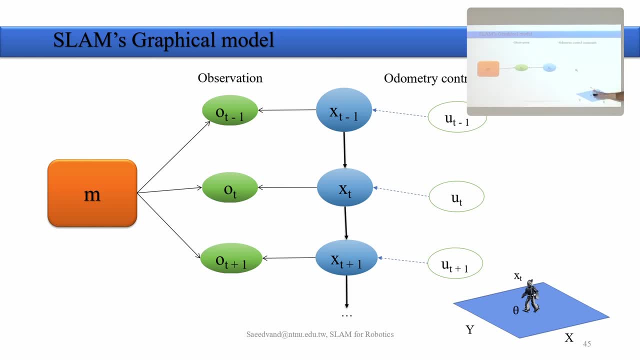 this is the model of the environment and this is the robot that you can see XY and depose, But the, of course, if we have that in current state, we have one previous state that this is. this is XT, the state after where the robot is. 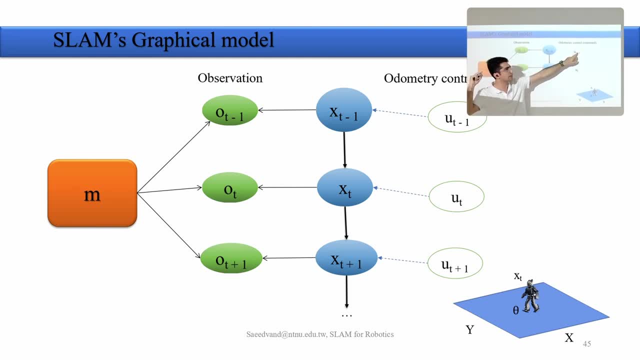 This is previous one, where it is coming from, and previous motion command that we run to came here and observation, previous observation that we have, Of course. then we have the future one too, XT added by one: the future motion command and the observation. 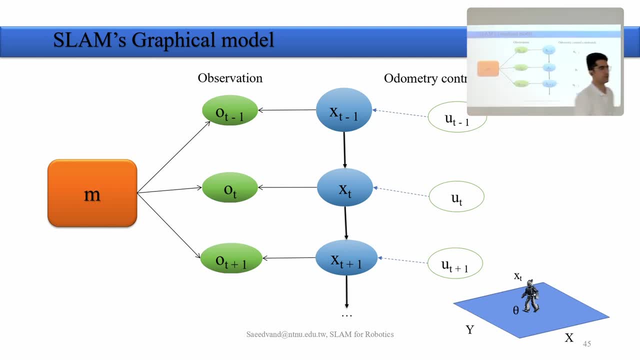 that we may have. You may say this is obvious why we need to represent it like this. Of course, we talked a lot about it, But we need to formalize it and bring it in the graphical mode so that when we are solving it in mathematical form, 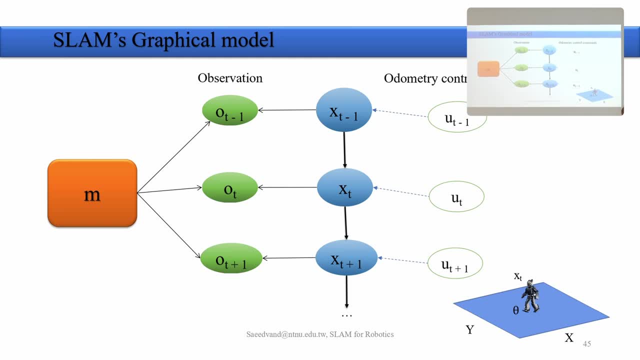 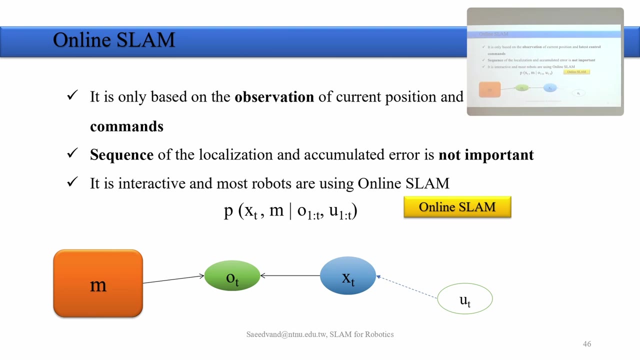 you understand it. what's happening better? That's the reason that we have graphical representation and we have some algorithms. even they are working based on the graphical representation. They are relying on this And we need to see what's happening. Now let's make the problem more dramatic. 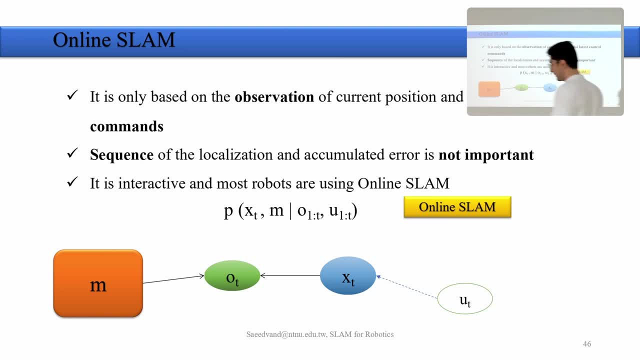 What is the dramatic part? We can classify SLAM algorithms into two general approaches. One is online SLAM, second one is offline SLAM. What does it mean? It means that everybody listen, pay attention to me. So I'm here. 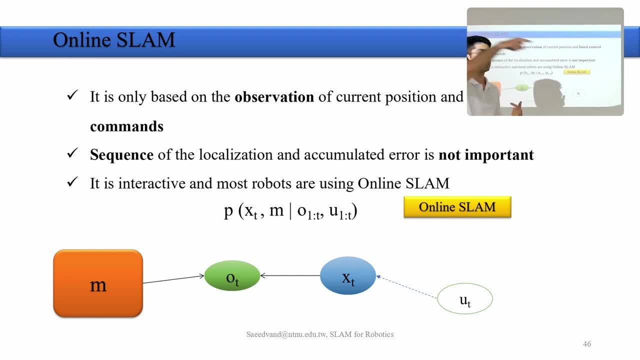 I can start to move as robot and come back here Then, when I finished, construct the map and localize the puzzles that I went through. This approach is called offline, If I do after finishing, But if I want to construct the map every time. 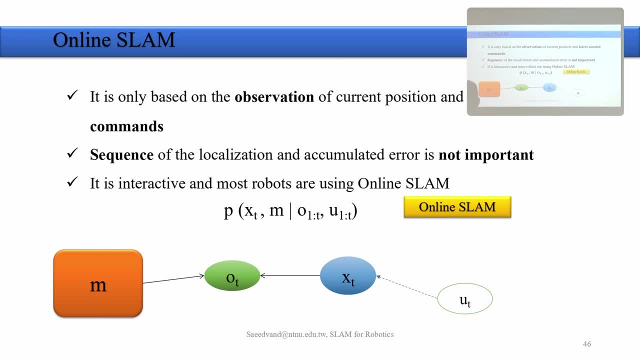 and after each moving and localizing. this is called online SLAM. The techniques are quite different. Think a little bit about it. Why can be different? It's like one time you can see everything. then you want to construct the map. 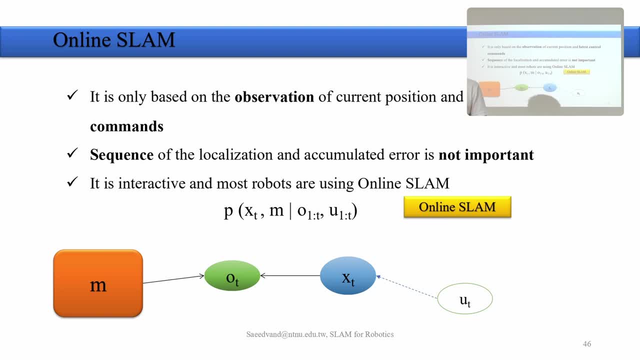 in offline SLAM, That's easier, kind of can be easier, but that's offline, That's not kind of. you cannot use the map meanwhile that your robot is moving in the environment, But in some applications that's quite useful. 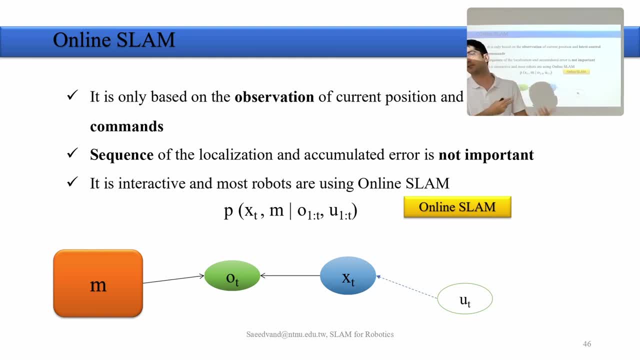 Because you can achieve better results. but that's offline later. On the contrary, we have online map. that online SLAM in online SLAM robot is moving in the environment and each step tries to construct the map and the localize the position of the robot. 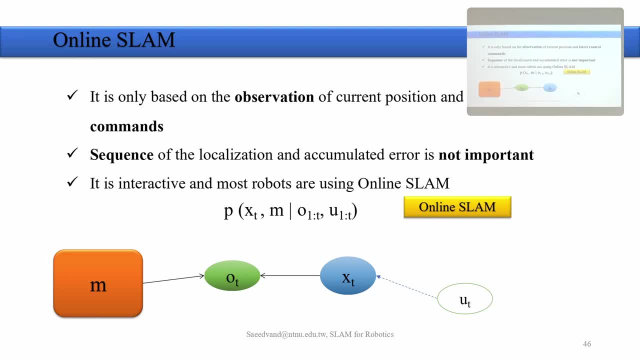 That we have two, two branches for it And basically in this course we will talk about the online SLAM. Mostly we move toward online SLAM And you know about optimization or the algorithm optimization algorithms. those usually go to offline SLAM. 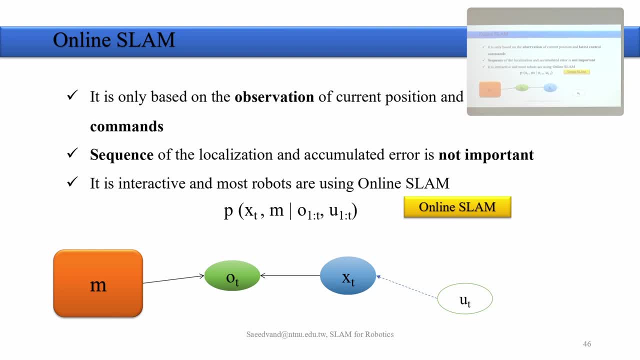 But they are very strong, They can be, they can be work very well. But also we have some advanced techniques that, trying to merge these together, They say, okay, I have the online, but some in some points after some time, 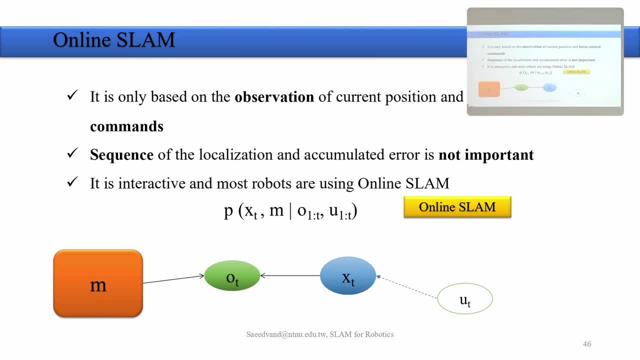 I can. I can apply offline techniques to improve it too. And and if you want us to show the online, we show in this form, not X1 to T. In previous time we saw general problem X1 to T. 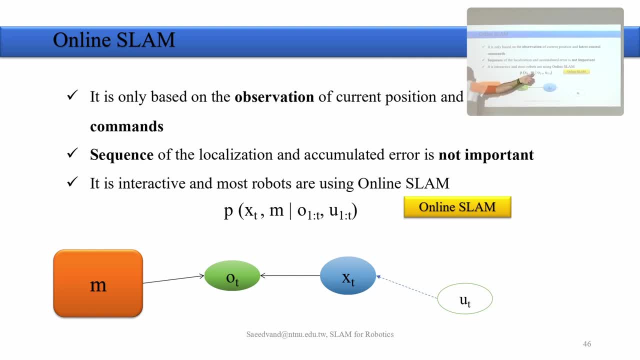 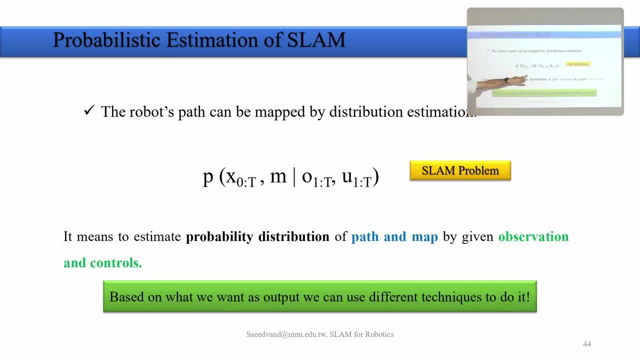 Here we have probability of the X, T and M, Not the pass. just the pause Here. if I go back here we have the pass. general problem of SLAM. We wanted to find the probability of pass and the map. 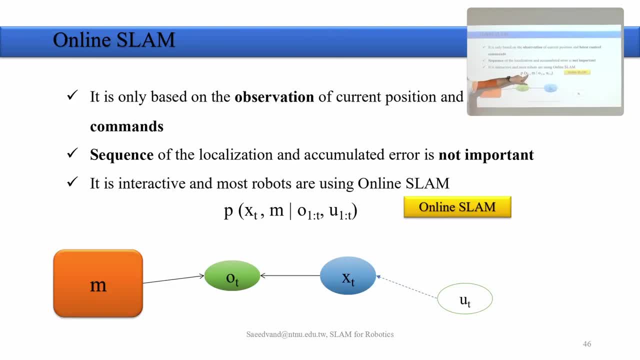 But here we have the probability of the pause and the map based on the observation one to T and motion command one to T, And based on this we only have this part over here, Not the whole graph like this: 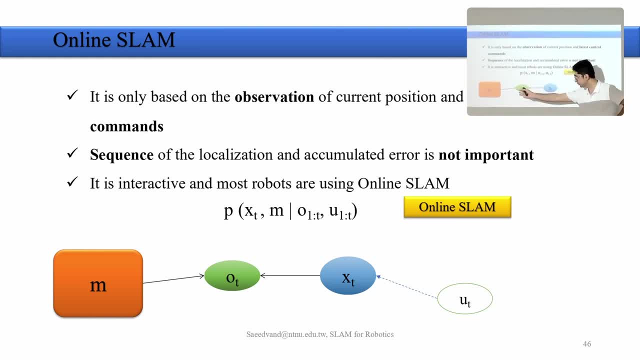 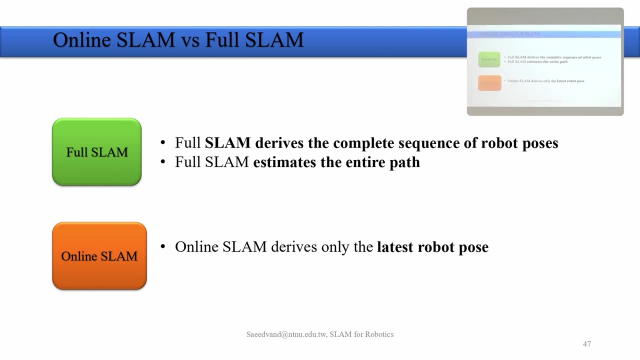 I mean, I mean, the calculations are mostly relying on this And in next chapter we will start with base filter that we will see. the assumption is like this, And goes on, goes on, just the belief that we- I will introduce. So 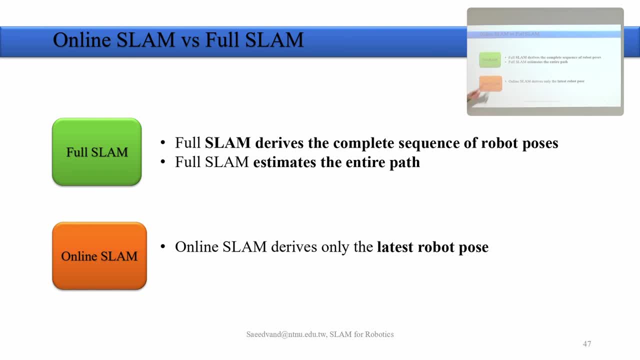 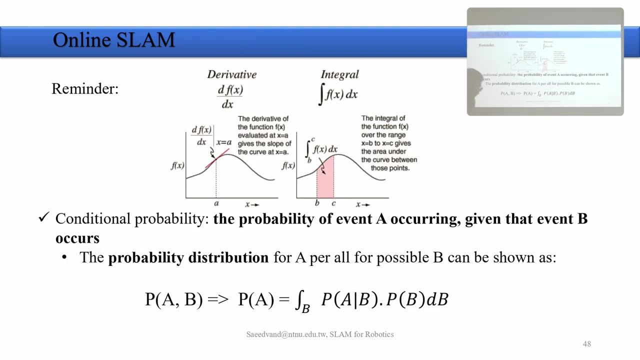 offline SLAM also can be referred as full SLAM. Full SLAM derives complete sequence of the robot pose and estimates the entire pass, But online is only on the latest robot pose. So, of course, since we are going to use math, 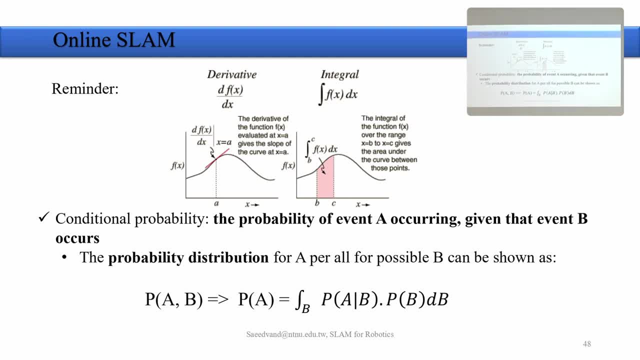 you supposed to study many of the things that are related, But I'm trying to, during the course, introduce and quickly refer what I'm talking about so that you can understand what's happening. For example, we have derivative. What does it mean? 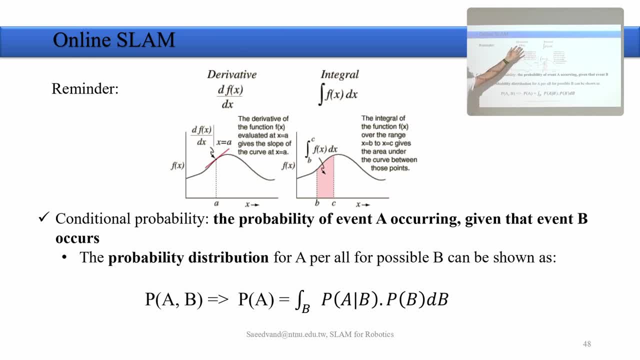 Because we are going to use it in our equations a lot. We have integral. What does it mean? Because we are going to use it a lot, You may forget it. So, whatever you forget it, please study during weeks for next week. 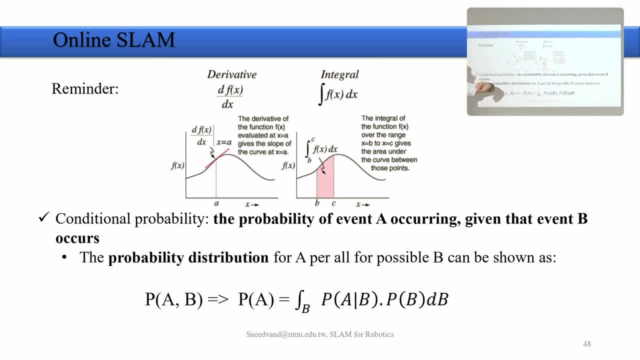 But I quickly try to mention it. what's the general topic? For example, when we are talking about the derivative, the part that is important for us is the calculating the slope of the, the slope of this probability, Like we have. 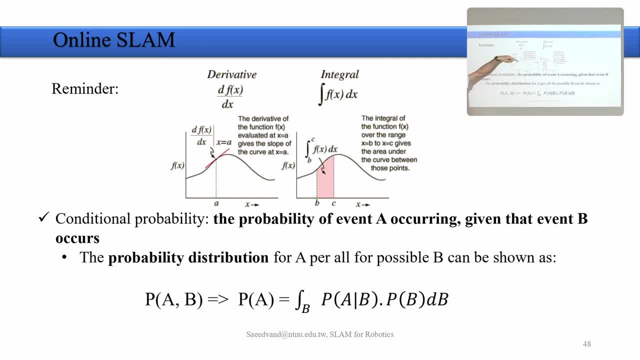 for example, Gaussian and for given point, like A or X, here for given point you can calculate the slope of the this curve here. So we are going to use it. And if you have studied like other courses, 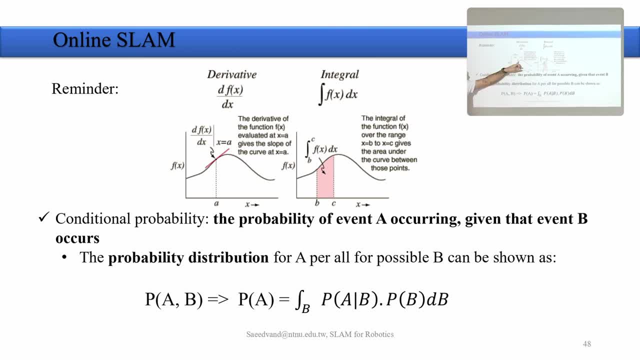 like machine learning, deep learning, reinforcement learning- you may face with it And that's very useful for learning. We have integral. What is the integral meaning that we are going to use? And this is very important for us Because 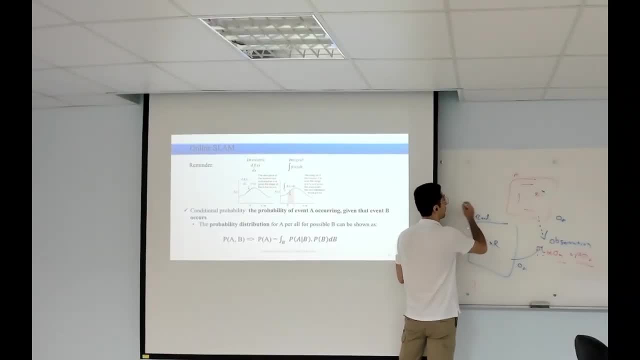 I told you we are, we will, our, our. all talks are about the probability and the estimation of based on the Gaussian model, And when you have Gaussian model, you need to know: okay, what's the probability based on value. 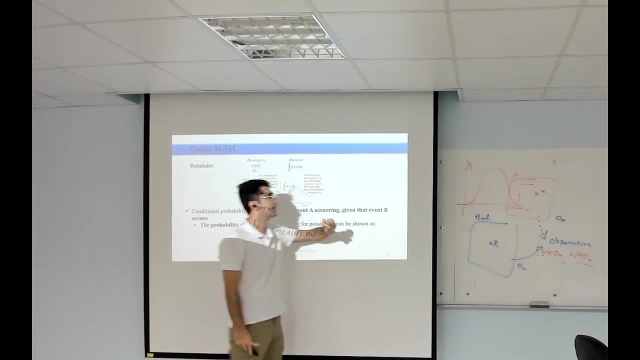 Calc bring some value based on this And how you can do that. You can use it integral And in integral you can say: okay if you, if you want to say the integral of the function fx between b and c. 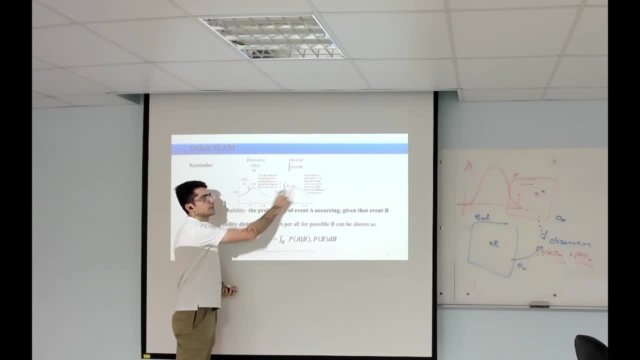 shows the, the area under this part. So we can say what is the amount, the value that shows the area under this. And you know, in math it's impossible to solve directly Because, because this slope should be, 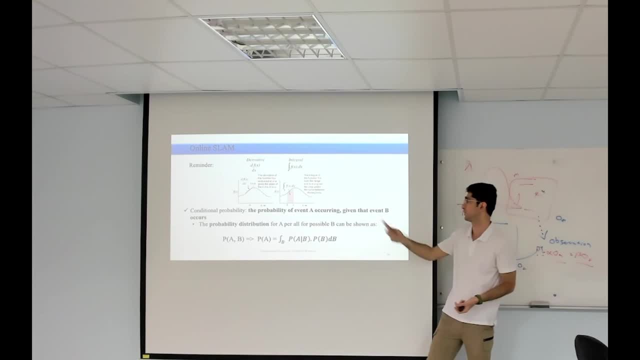 and and if you want to write the program- and we usually just criticize this and we can solve the integral in descriptive form and get the value of the what's the area under b and c And then, based on that calculation, we will use it in. 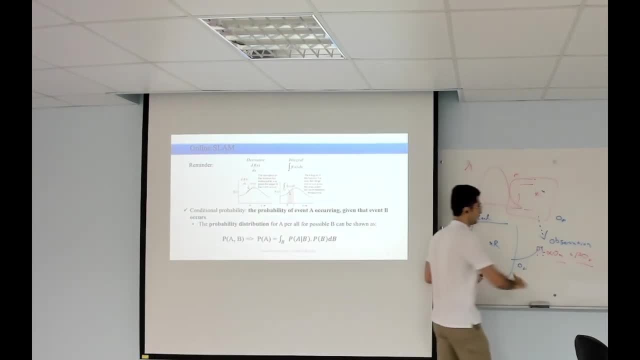 in, for example, if you want to compare to Gaussian models, for example. simply, Of course there are many, but just I: what is the that one and this one, the differences, what is the like, the area? 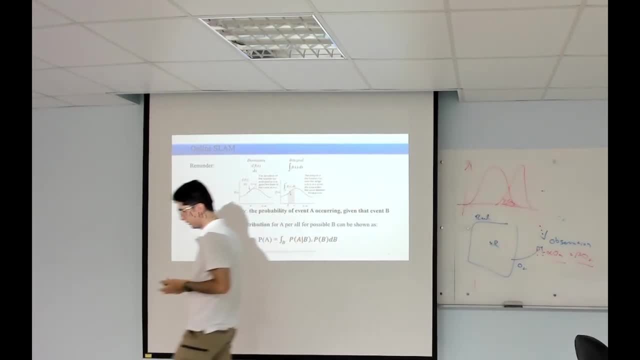 that is covered. So, based on those things, you need to know what's the topic. Plus, we have the probability distribution. That that still. if you forget it, just have a look The probability distribution for all. 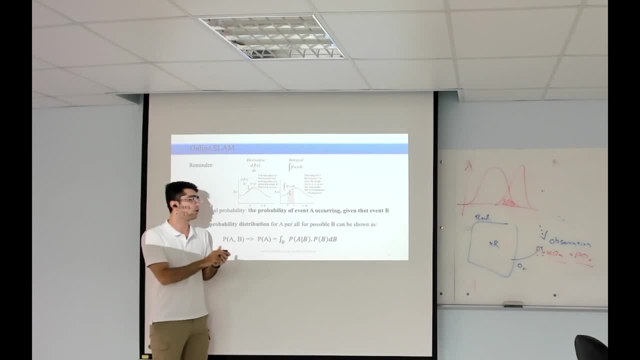 in conditional form that that still. if you forget it, just have a look So we can say we can get the integral of the probability A given by B times probability of the B that it says the. 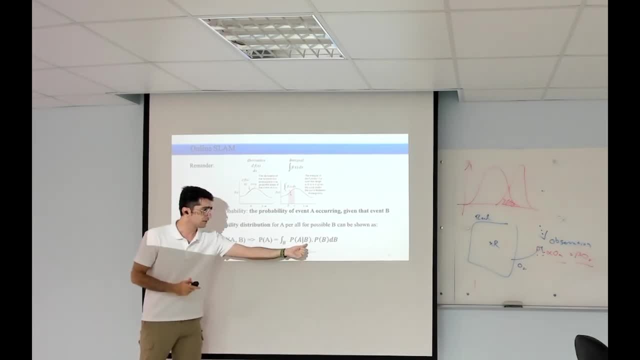 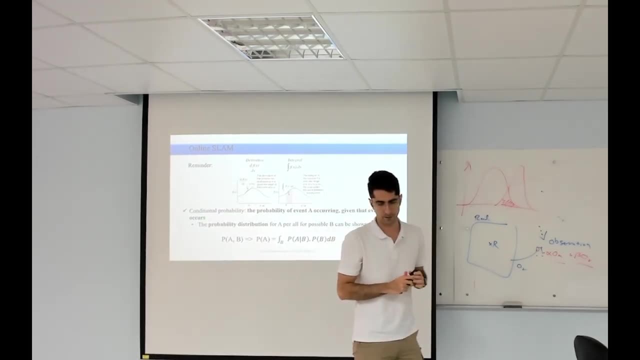 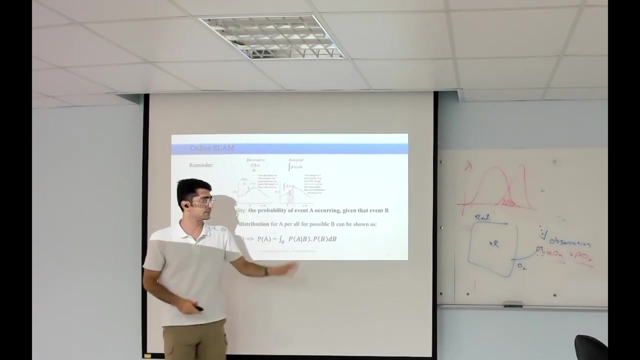 for all possible B's. for all possible B's by giving A, what is the probability So A is given? and for all possible B's, what is the probability that we can get integral of these term over there? And? 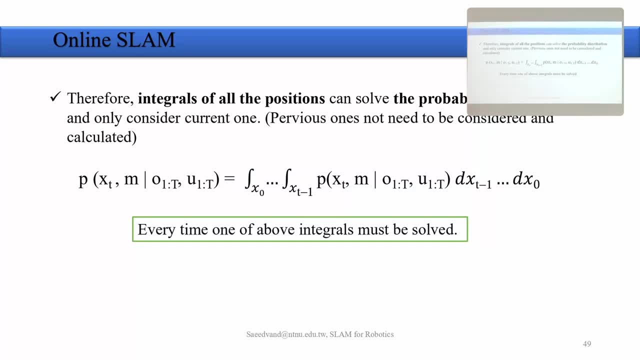 you can have a review if you forgotten. So, based on that, what we want to do in online SLAM. so we want to get the integral of the, the probability of the XTM given by observation and motion command. 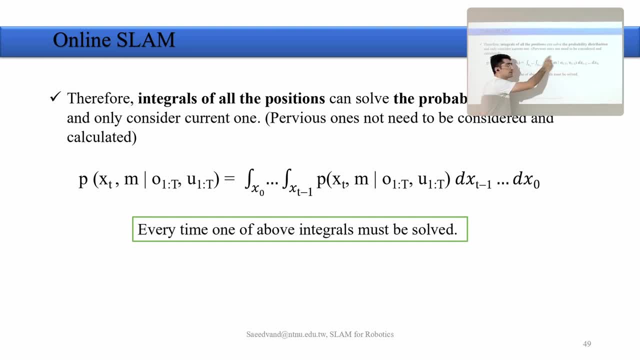 So convert it kind of to a value that what is the probability of the where the robot is and the map is? And if you want to solve full SLAM, it is all of them. So 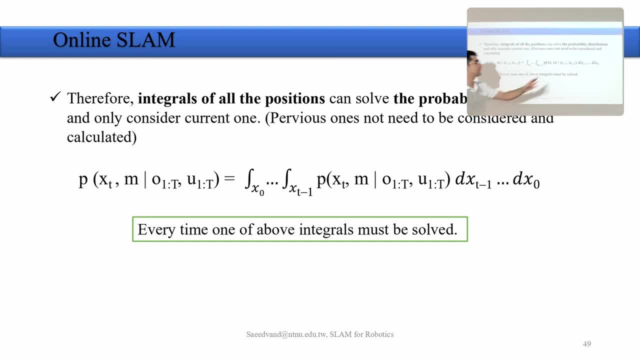 for each pose and the map that we have based on the each motion command and the observation. So if you want to calculate all of them, we have full SLAM If you want to just solve one of them. 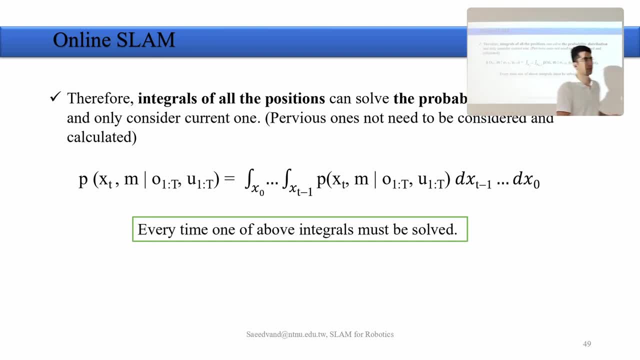 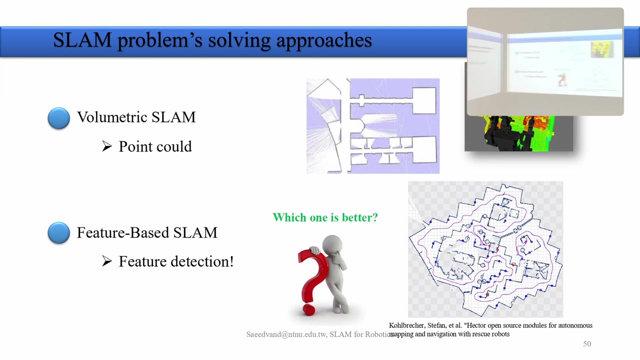 we have one of this one- So this is called probability distribution- and of the where the robot is, and we opened it exactly what's happened so far. So about that we will talk more. 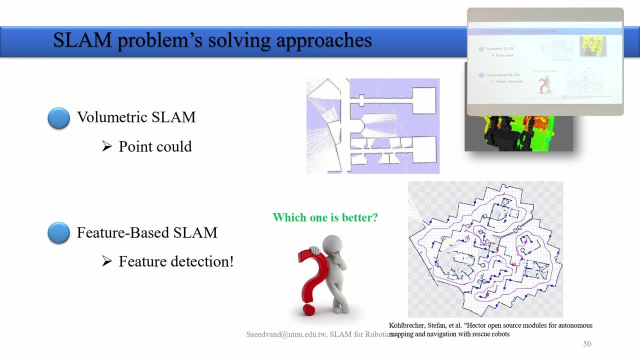 We will extend it and use different algorithms to do that. Let's talk a little bit also about the maps. We have different kinds of map. I mentioned a little bit. We have volumetric SLAM like point cloud, So 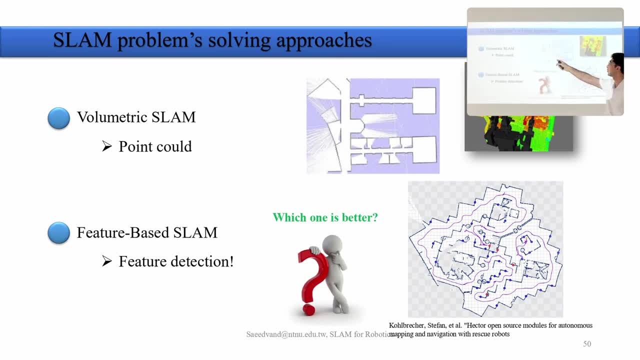 volumetric SLAM can be as point cloud and it shows the volume of the environment. So this is the scan of the LIDAR scanner. This is the robot in our lab and this is me. that robot is scanned. 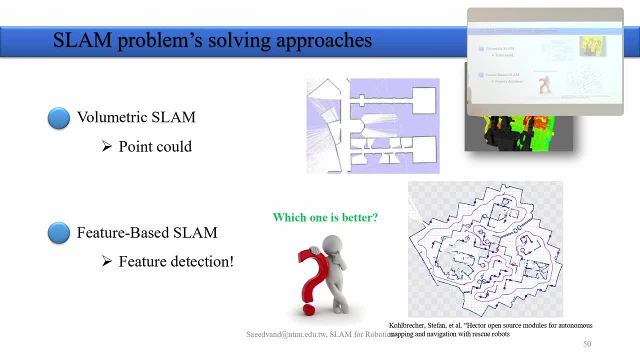 me by LIDAR scanner and you can see that it is point cloud of the environment. That's one kind of map that we can have in 2D form or 3D form. We can have feature-based map. 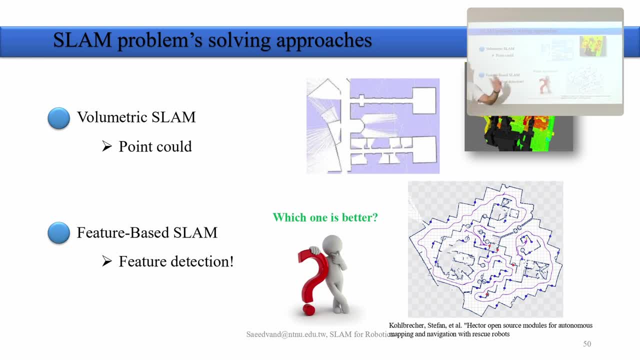 that the feature-based map detects the features of the environment instead of having the, the volume of the objects like, like say, let's say, in this environment, I just want to get the corners and edges of the. 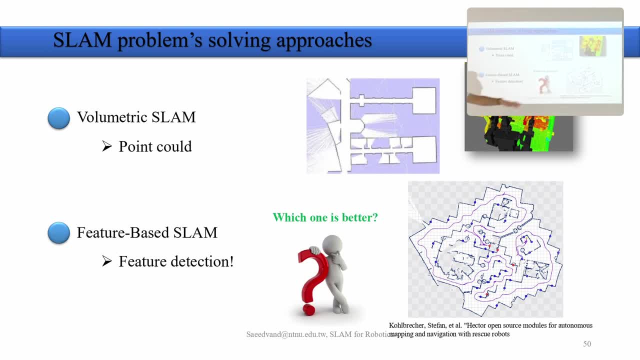 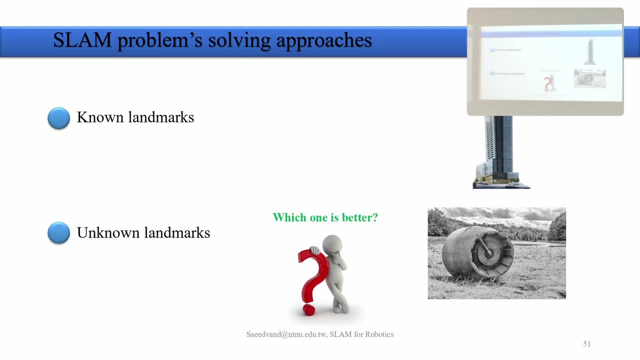 each, each object, Then that's feature that I can extract and construct the map like that. We will also see this technique how to really implement and how you, how you can do that, So we can have known landmarks. 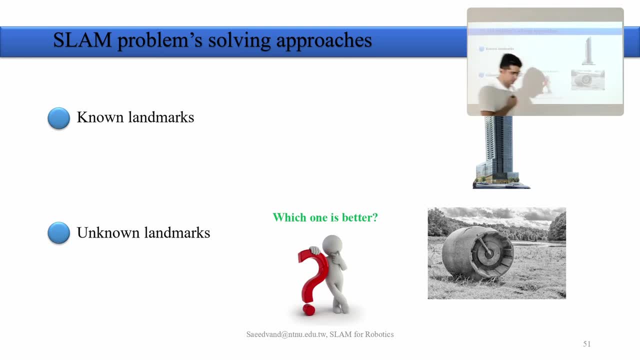 and unknown landmarks based on the map that we want to construct. Known landmarks: it means that we know the landmark exactly what it is and we we can detect it easily. For for this class at the beginning: 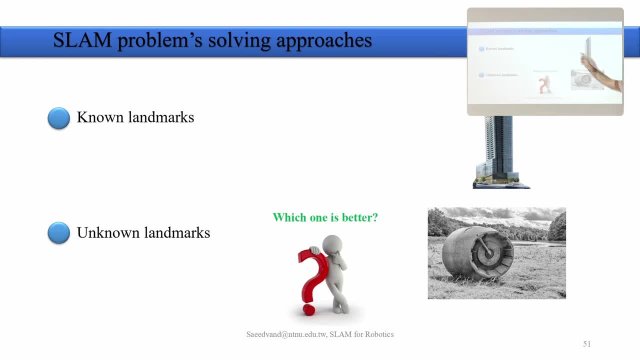 we consider like that because we don't want to solve that problem for now in the techniques that we are using. So we will assume that, okay, the landmarks we know at the beginning, but there can be unknown landmarks. 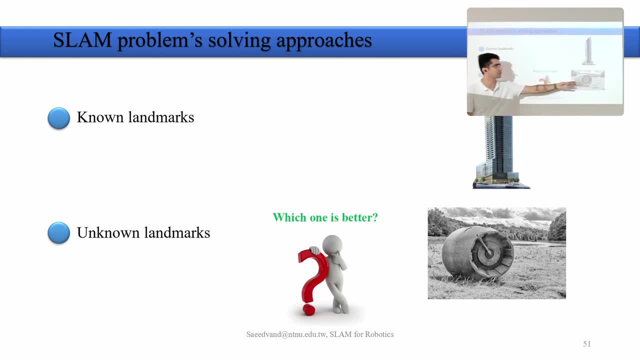 that we don't know what they are. even a human. who knows what is this? No one, Okay, I think. I think I mean no one human, doesn't? They found it and they don't know. even scientists don't have any clue. 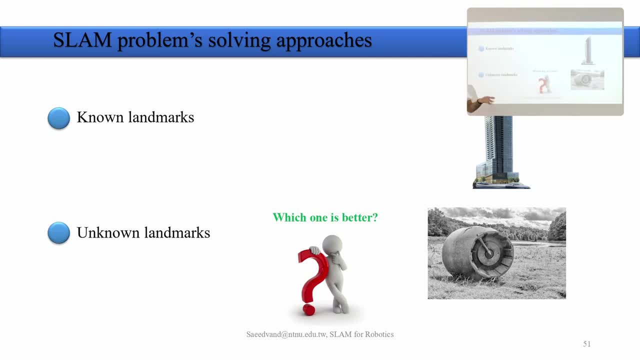 what is this Right? And this can be valid for a robot for everything, Because robot doesn't have any idea what is this chair, even Unless we define it, So we can have unknown landmarks, We can have static environment. 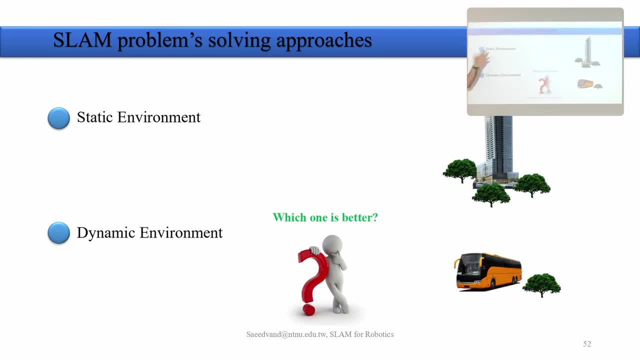 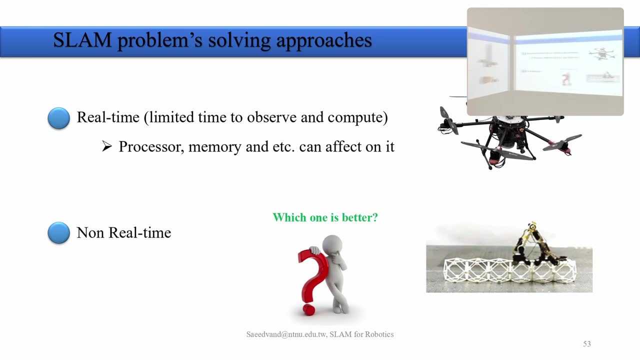 dynamic environment. we talked about it. Which one is better? Of course, if we can cover, dynamic environment is better. We can have real time or non-real time environments. that also, this is another class of the model. 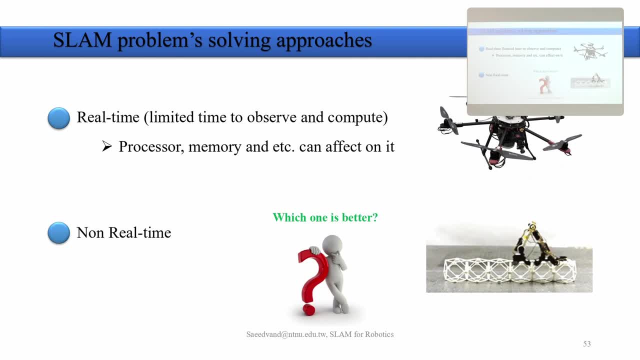 but you can kind of consider it is similar to online and offline one And we can have also this is another class of the model, but you can kind of consider it is similar to online. 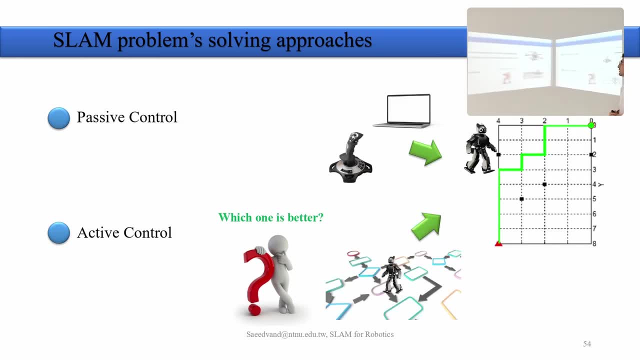 and offline one, The online and offline SLAM, or full SLAM or online SLAM. Then we have the control part of the SLAM. that is another perspective that we need to know: Passive control, active control. 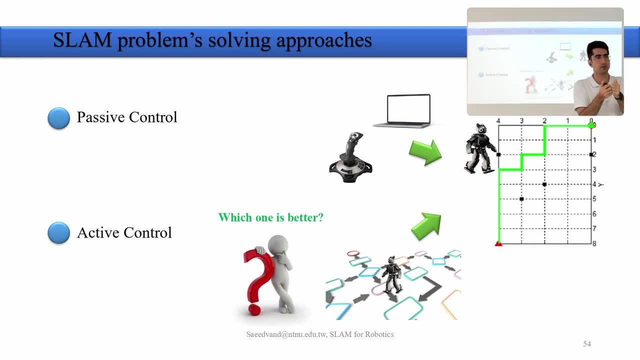 Passive control is mean. it means that, like I have a robot, I wanna use the joystick to control my robot goes and come back. then I say that the what is the locations of the robot and what is the map. 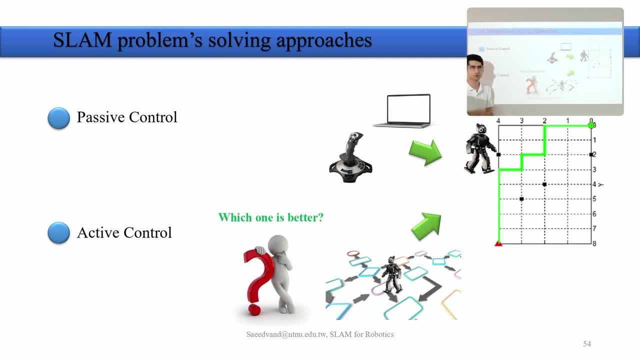 that's called passive control. but an active robot needs to navigate itself. So also at the beginning, we don't consider the active control, that we don't take care about the navigation, because 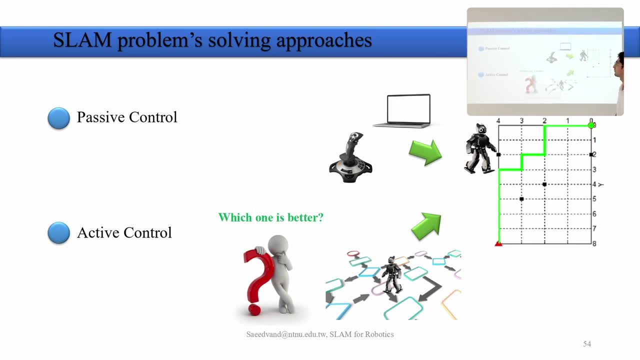 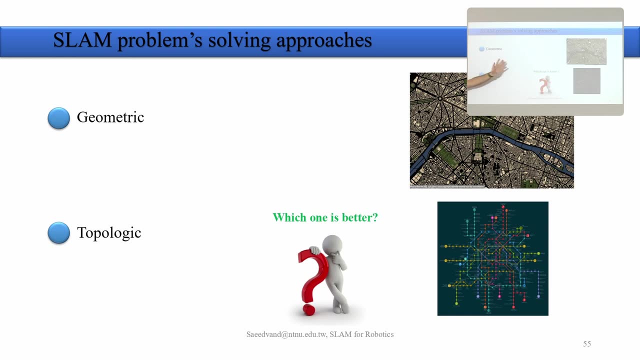 we need to break the problem and solve it small by small, Otherwise it's impossible to solve. We have the class of the geometric maps and topologic maps. Geometric map: you have map like this from satellite. 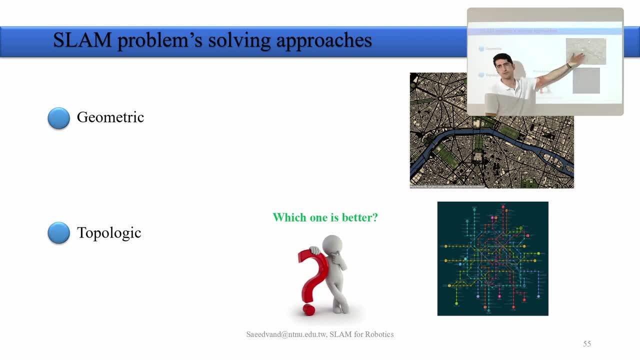 But this is nice. but it has a problem of the hidden passes because, like there can be some, some passes indoor that you don't see in this map, But we can also have. 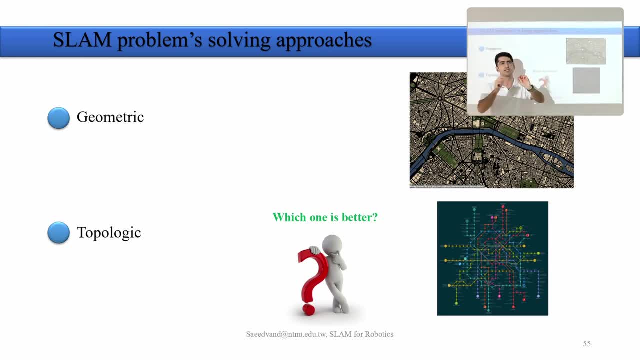 topologic based maps that shows the connections also the just the links where they are connected to each other. So maybe you have a problem that you need to get the output as topologic map with robot. 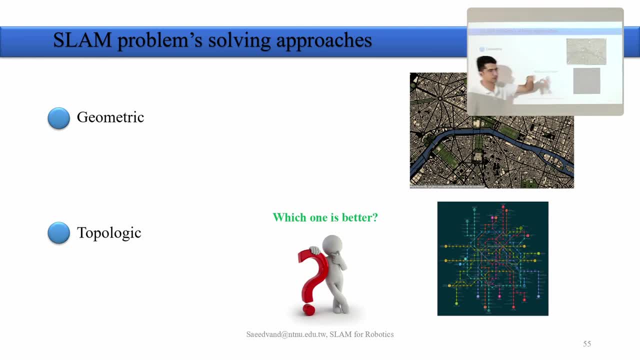 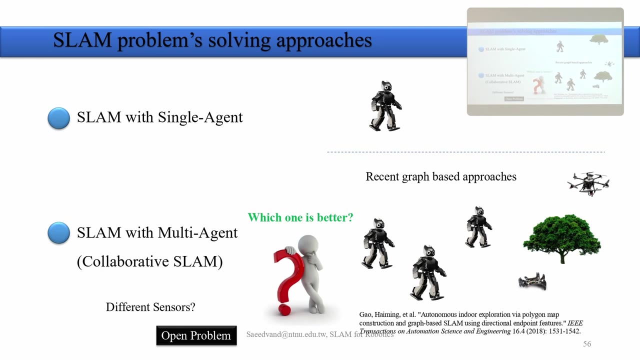 So, or maybe you have a problem that you need to construct something similar to a geometric map as robot, So as developer, you need to decide. We also can have much more advanced algorithms like SLAM with single agent. 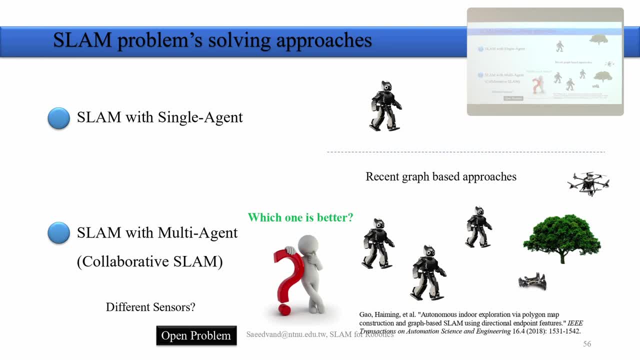 that we talked so far, and also we can have multi-agent. What does it mean? We want to localize independently, construct a map, but finally the map is one map based on different robots that we have. Those can be. 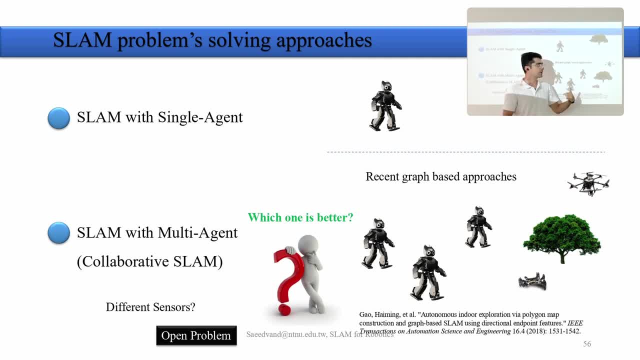 humanoid, those can be quadruped, or hexapod, or drone, or whatever. it is different sensors, they are moving in the environment and finally, we can have one single map. So how to do that? 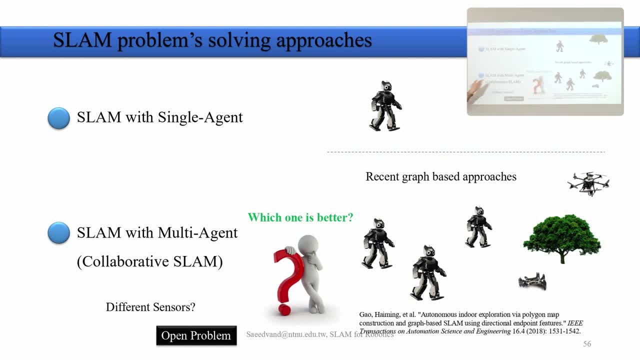 is multi-agent one. that is it also open problem. that is is a challenge and this can be easily appear. this can be easily a PhD thesis for for who wants to study or 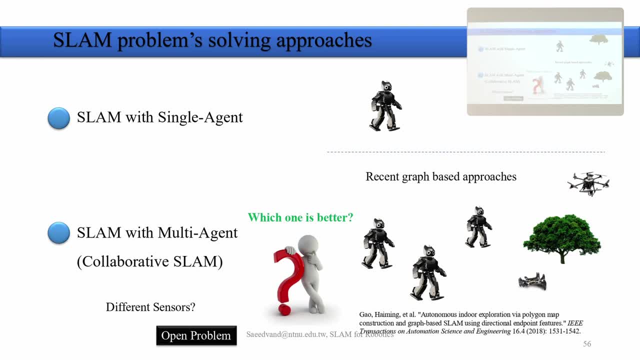 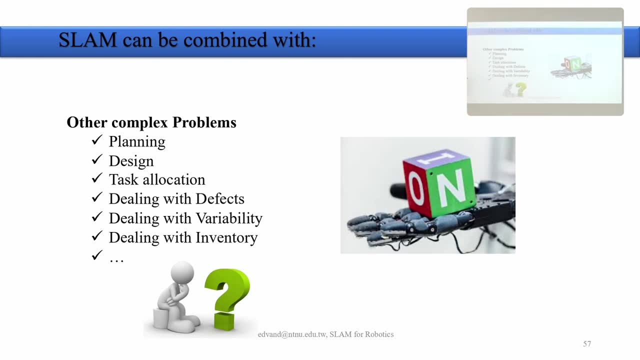 this is open problem for companies, you know, and big problems. So I already talked about the related complex problems. like we have planning, we have design, that in design you can think how SLAM. 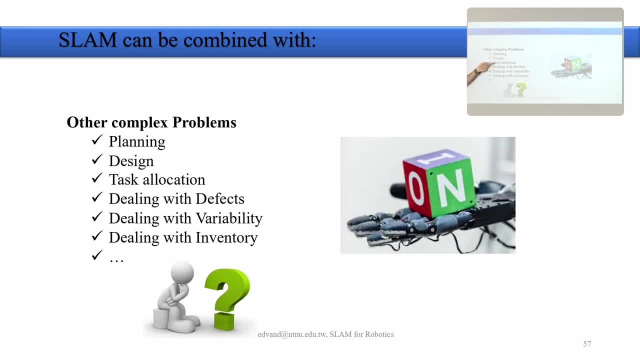 can be important. that's using your imagination, task allocation. we can using task allocation problem very diverse and big problem that I can say there are hundreds of problems of task allocation. it can be robot to. 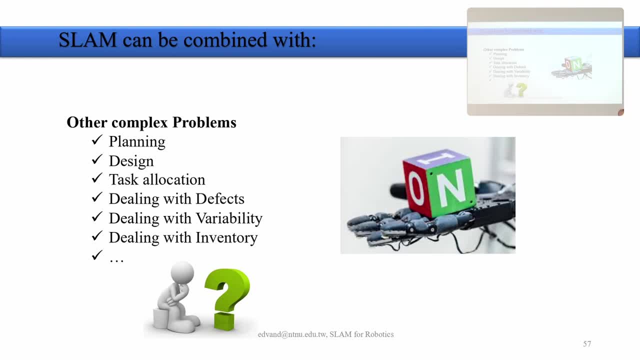 to pick an object. it can be traveling salesman problem- I hope you know traveling salesman problem- and many, many application programs that are very well known in the world and it can be used there dealing with. 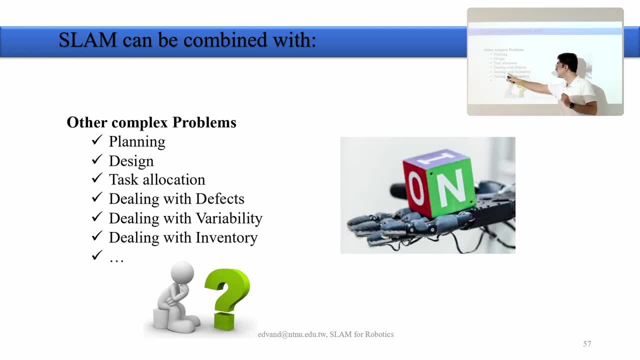 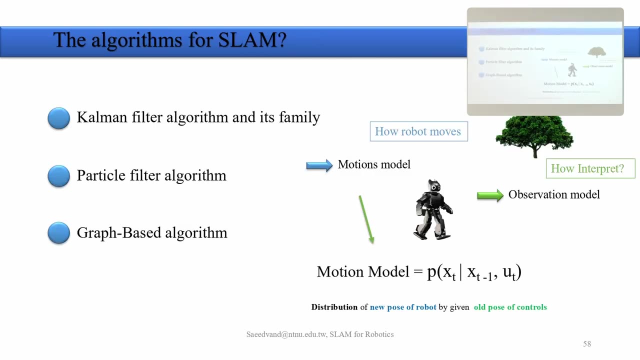 dealing with the defects, dealing with the variability and dealing with the inventory. there are also some relevant ones that can be combined and used with, and the algorithms that we have. first, 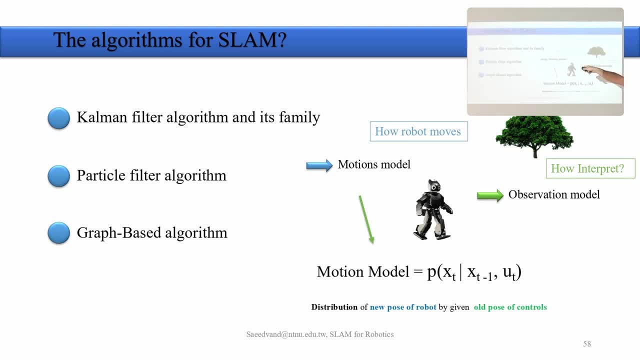 we will start with base filter then. that is underlying of all these algorithms when we go to Kalman filter, family particle filter and graph base algorithms, and all of them are going to use motion model. 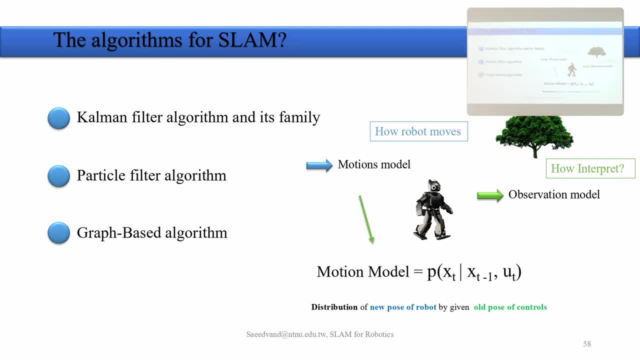 and observation model. so what does it mean? we are going to use observation and motion model, combine them together with these techniques, in order to achieve first simply localization, then later how to construct map. 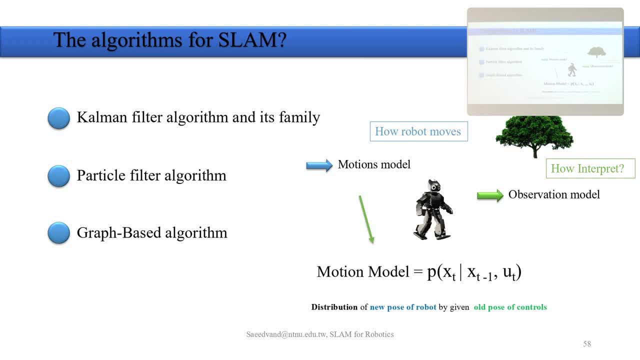 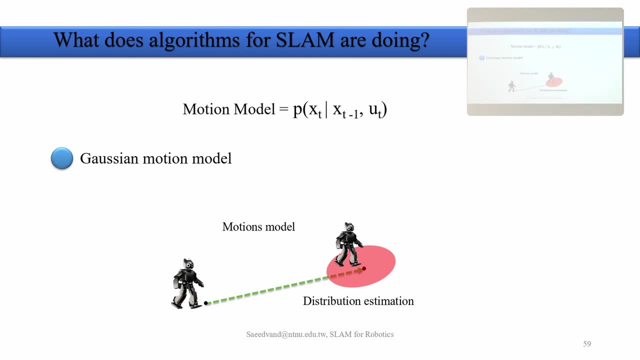 and we. we will see them separately in the next video. so motion model can be seen as the a little bit different than what we've seen. motion model is equal to probability of 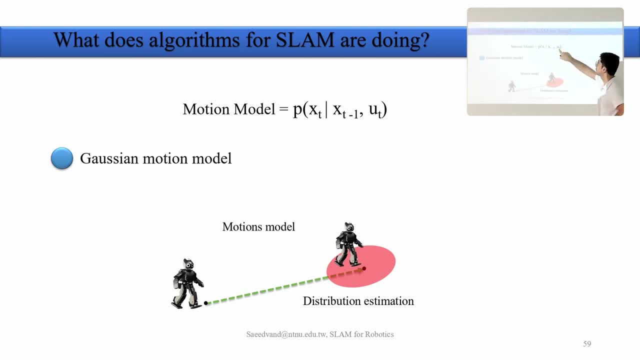 xt given by xt minus one and ut, it means that. so my current robot's current pose is based on the previous pose and motion command. next week we will talk about that space assumption. 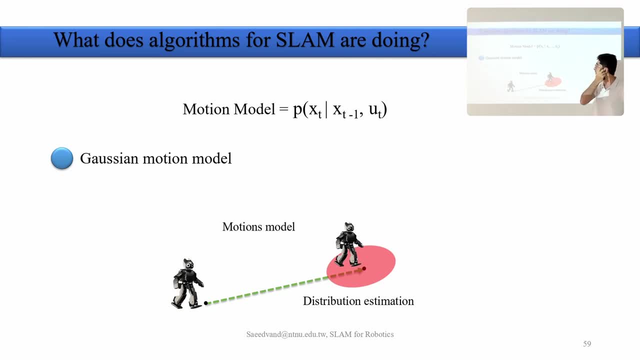 I'm not going to explain now- and we have the Gaussian motion model- that this Gaussian motion model is the distribution estimation that I explained a little bit there. these are as input, the second one. 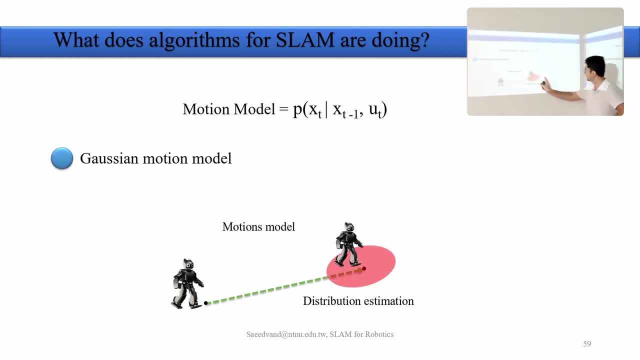 sometimes we can have like: this is the Gaussian distribution, but in some problems sometimes we can have non-Gaussian distributions. then we will see what kind of algorithms also can can deal with. 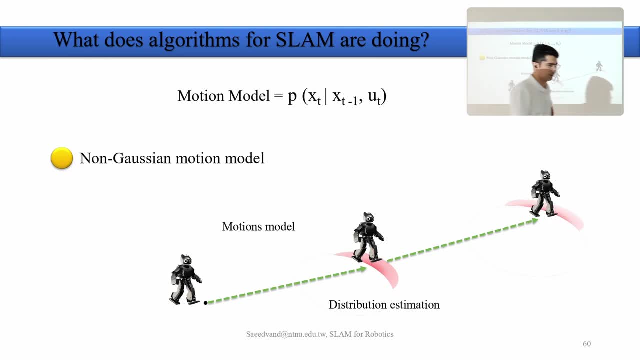 this one. why? why we can have non-Gaussian distribution. we can say that we are able to distribute and, you know, can have non-Gaussian distributions if we want a single yeah has. 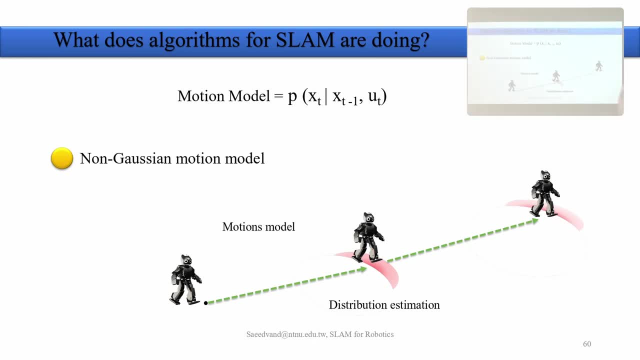 equal or small distribution. for example, one time we can have a double interaction of source and the whole field start from each of the Y-axis. So this is what you are trying. 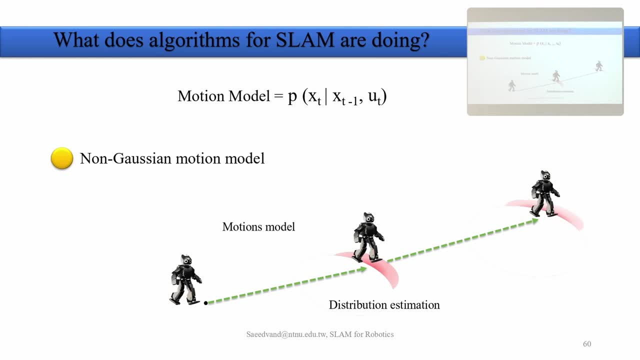 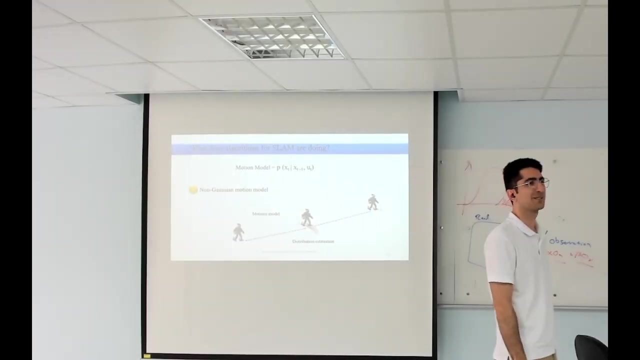 at. You are a master student. You should be very active. Who can answer this will get a direct positive mark? Maybe if we have outside factors that shift the lower position probability to a different point. So the distribution curve is asymmetric Very close. The answer is very close. 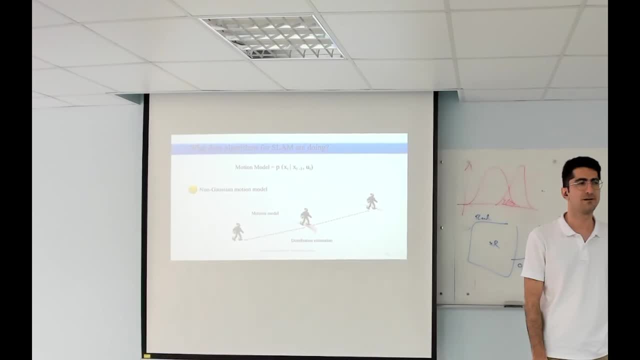 If we have a drone that has sidewind and then it's more likely to be angles in a different way. So this side of the Mm-hmm The pyramid is more steep than the other one. You're very close, but explaining a little bit far. 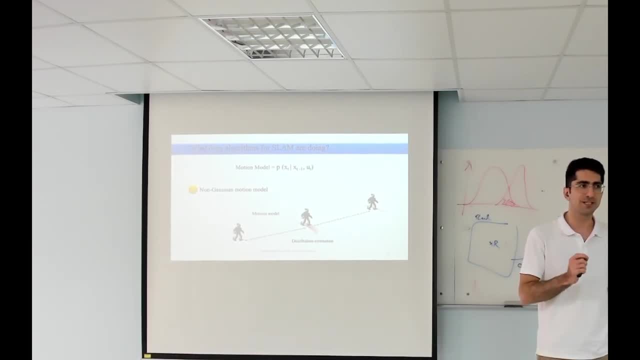 But yeah, very, very close. We have two parameters, that they are different, but not on the curve. On the curve, but you should think 2D not 1D. You're thinking about this model, Think about the Gaussian distribution. 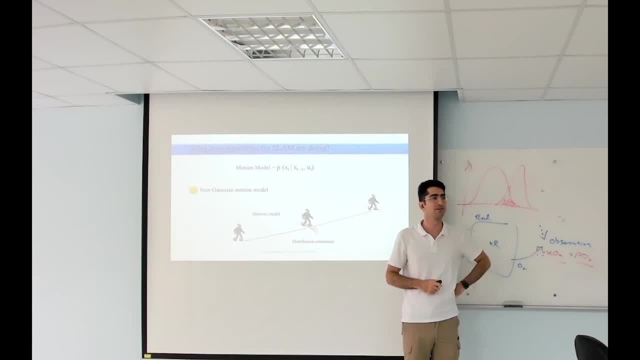 Gaussian distribution in 2D We have two models with the map and we have two poles. So maybe if the map is wrong, the distribution will get Very, very close. Map and poles and Very close. but I know what you want to say, but you don't know all the parameters. 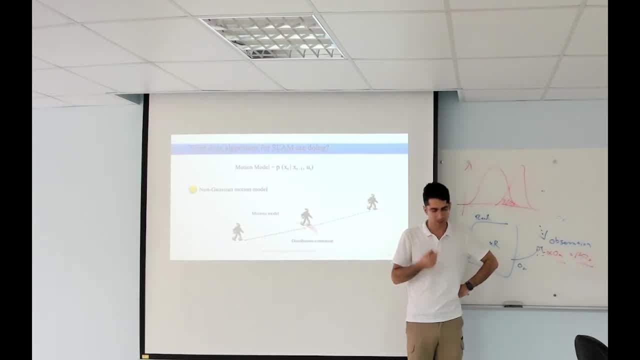 Okay, I can almost accept. but let's see, Yeah, because you're getting very close. Like, let's say, robot is here. Okay, If I have rotation ability and move forward ability, that I have two parameters. right, If the error of both are same, I have Gaussian distribution there. 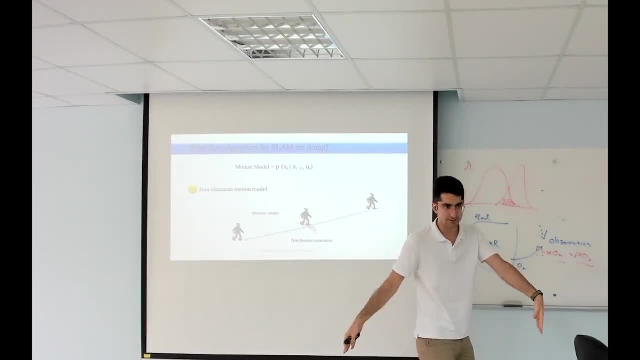 Because if I move forward, the error is like this amount And if I rotate, rotation error is the same, Then it will be circled there. But let's say my moving forward error is Moving forward. error is too small. If a robot moves too forward, the error is too small. 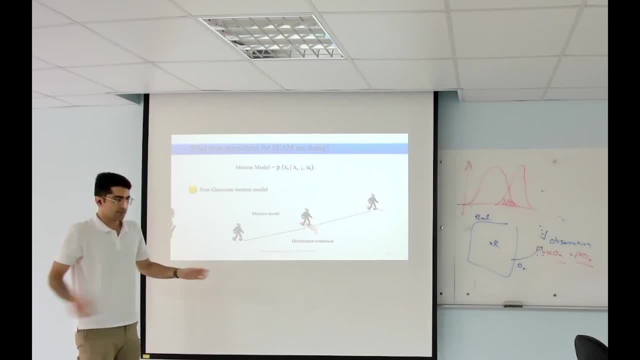 But my rotation error is too big, Then my curve becomes something similar to this: Move forward error is small, Then it shrinks, And this is not Gaussian anymore. It means that this is not this form of the distribution anymore. So moving forward error is the same as the integral error. 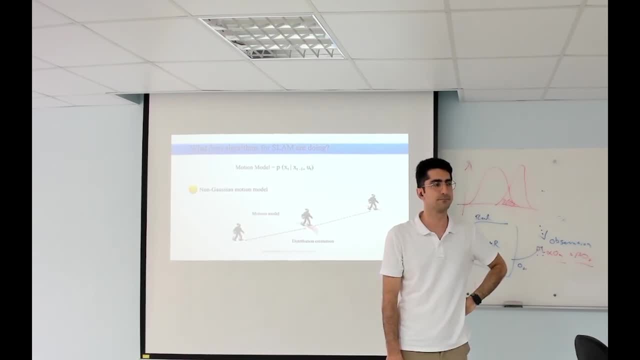 Then the error of the position will be like Gaussian distribution. Yeah, that's simple, Like, let's say, my forward. I have motion commands, right, Two kinds of motion commands: Move forward, rotate, Move forward, let's say, for me zero. 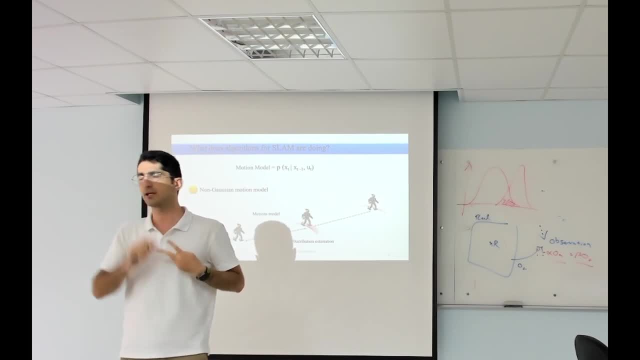 I have zero error in moving forward With millimeter accuracy, I can run it. But I have a lot of error on rotation, Completely wrong, random. Then what happens If I say move forward one meter And turn like Turn zero even. 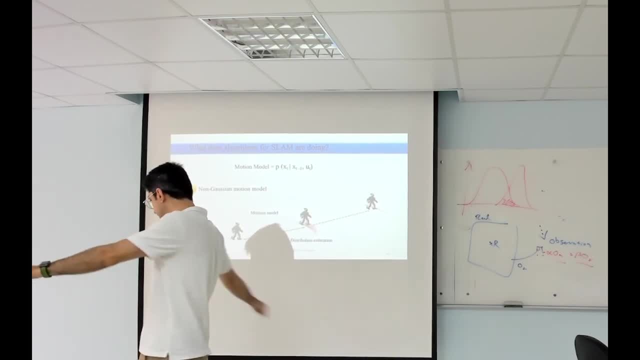 Then I maybe can be end up one meter around circle on the edge of myself right Wherever I can go, But one meter like One meter like here or there, If it's completely error, And this is This is the understanding. 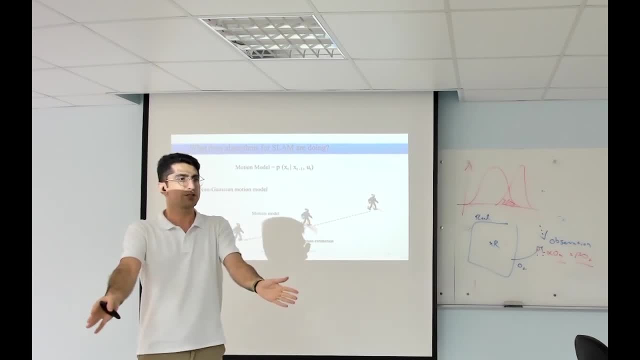 And if the error is lower, like 45 degrees in the rotation, Like let's say we have minus plus. Maybe better write it here. Robot is here- If the moving forward Error is zero And if If the rotation Theta. 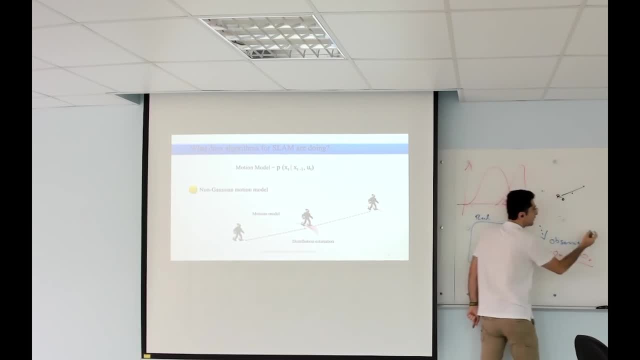 Theta can be completely random. If you run the motion command ut equal to ut, as like Move one meter, As ut equal to Move one meter, And theta rotate like Zero, Then robot can end up Everywhere Somewhere after one meter. 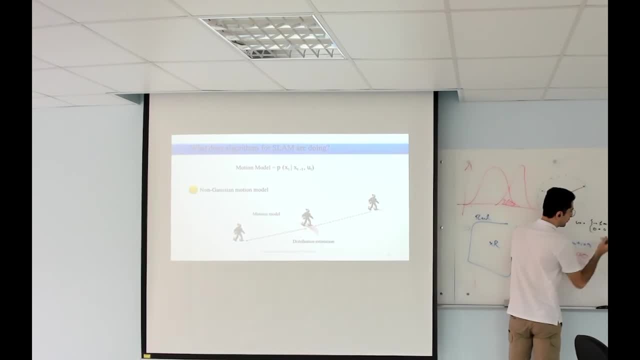 But if the error is For theta is like 45. Degrees, Then robot may end up Somewhere around here With zero error on the moving forward. With 45 degrees error on the theta, Robot may be here, End up here. 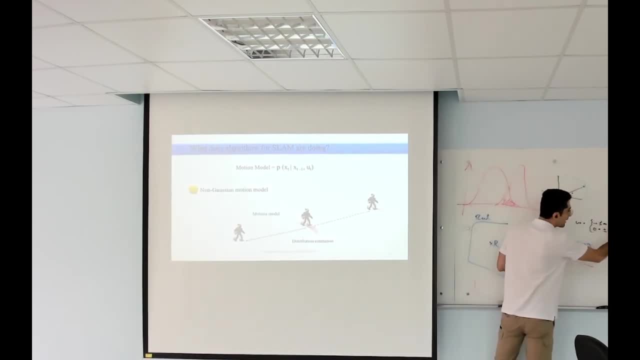 End up here. End up here Because of the error that we have. If you have some error here, For example, 10 centimeters error here, Then this can be Somewhere around here That this is 10. Right. 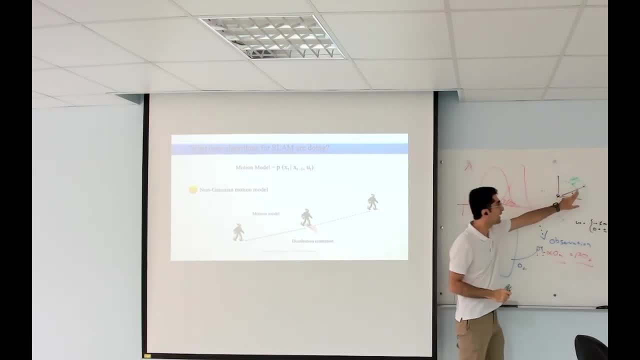 Everybody understand Exactly what's happening. So when this is happening And the error is different in these two parameters, Then we don't have any Gaussian model anymore. That's not circle anymore The estimation of the way the robot is- Because that can be- 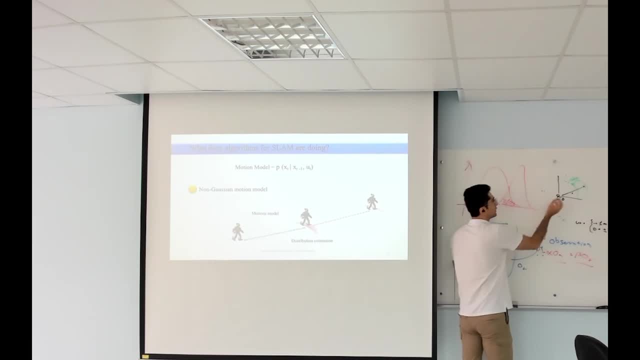 The form of the. This Gaussian distribution says, okay, Where the robot is If errors are same, But if they are not same, This becomes Some other kinds of curves like this: That That it is not Gaussian And we will see algorithms. 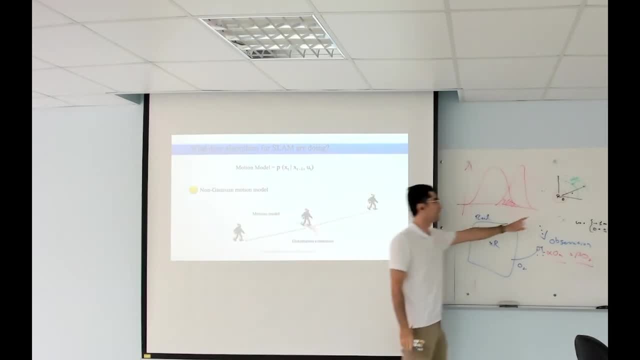 First how we can solve that problem. Then we will see that if, If the, If the model is not Gaussian anymore, Then how we can solve the next stage. So the single variable probabilities are both Gaussian, But the overlay of both is not Gaussian anymore. 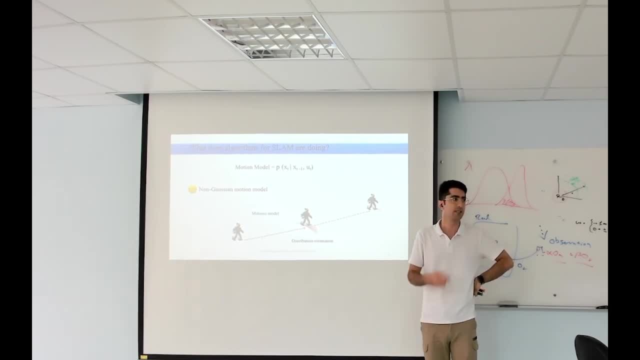 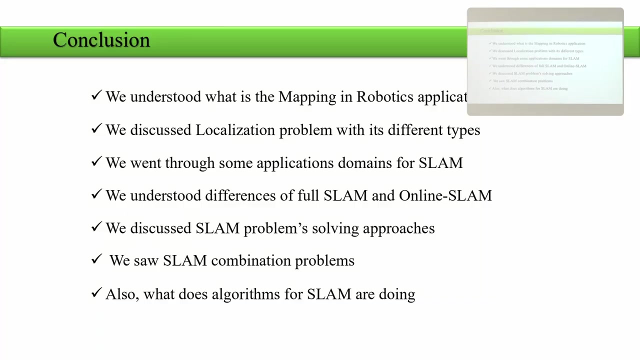 If they are different, Yeah, But if they have same value, Even if it's 10D, Then that's still Gaussian, Okay. So where is my remote Here? So let's conclude this chapter. We had understanding of mapping of the robot. 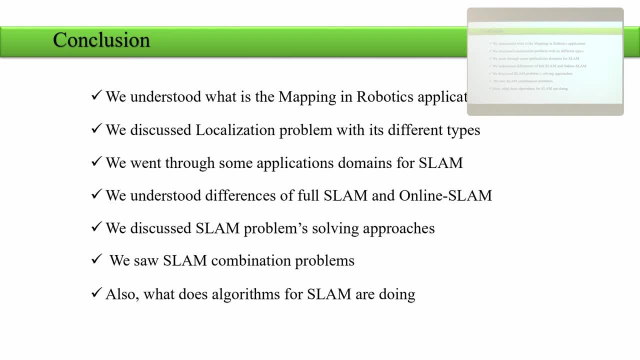 We discussed the localization problem With different characteristics, Different types, And we talked about the some application domains for SLAM. We understand the full SLAM and online SLAM differences As very important Because we have different algorithms in its split directions. 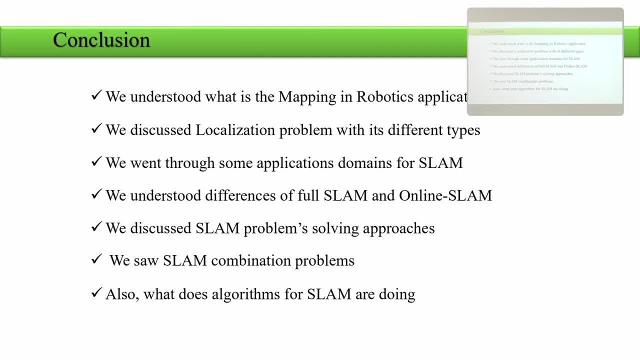 And we discussed the general problems that we need to solve with SLAM algorithms. Then we saw how the combination of problems can make challenge for us in SLAM And finally what the techniques that generally we can solve it That I introduced, for example, 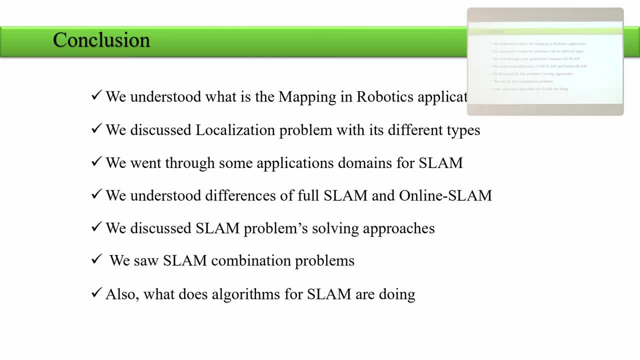 The much magical representation. Then we discussed that there are some techniques Like Bayes filter, Kalman filter, Extended Kalman filter, Etc. That next week we will start to talk, Dive in details of those, with some examples. Simple representation: 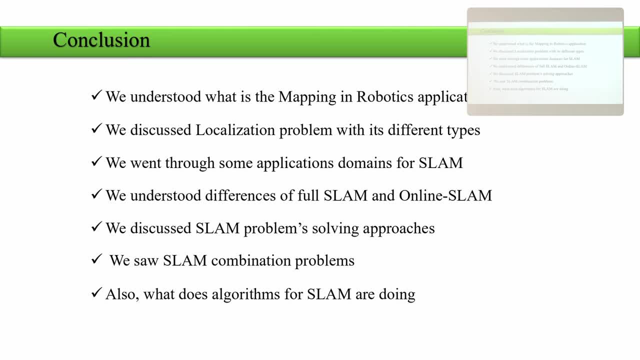 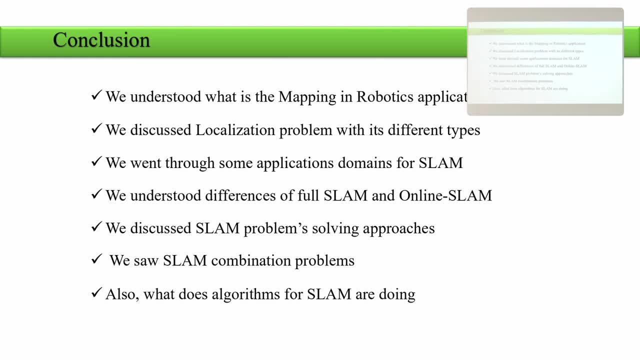 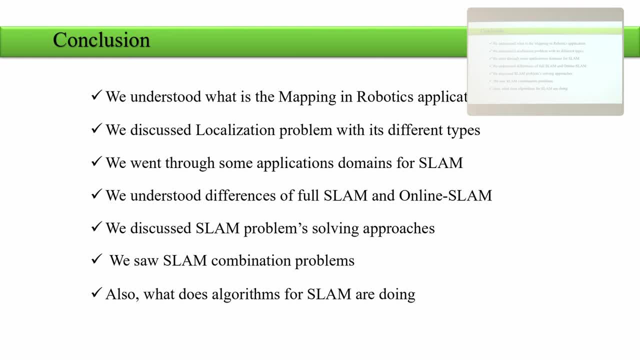